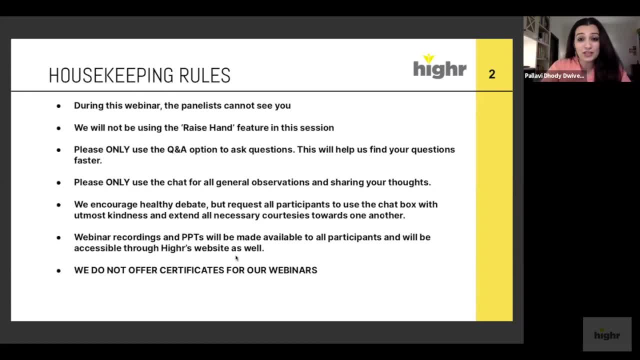 your sharings, making any pointed comments that you would like to make. We encourage a lot of healthy interaction and a lot of healthy debate, but we also request you to be mindful of everything that you put out there in the chat box or in the Q&A, and we encourage you to use those shared comments as well to help us find more questions. So thank you so much And I hope you will stay with us. Thank you. 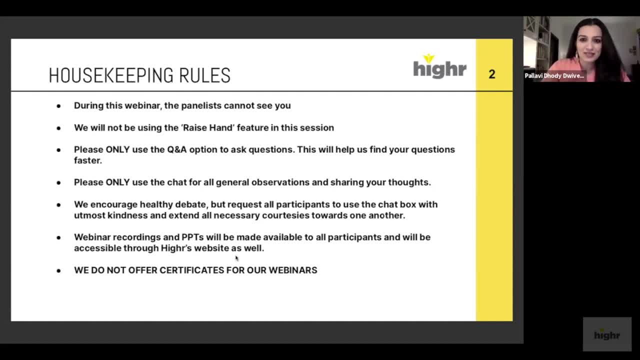 ask you at all times to be kind and extend all the courtesies that are required on online platforms like this. the world needs as much kindness as it can get these days. um, also, for all of you who do, who are interested, um in uh, in the recordings in the ppts, we will be mailing these out to all. 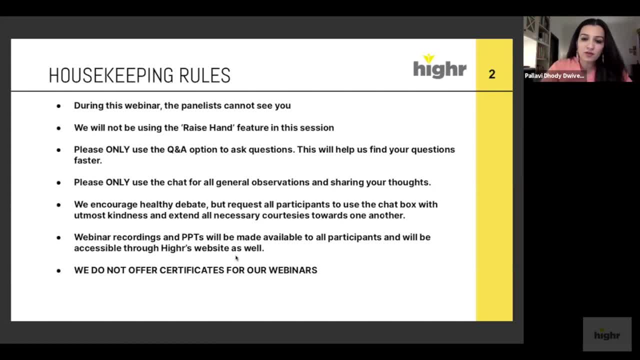 registered participants. these will also be made available across higher social media pages as well as on our website. um, just a gentle reminder, we don't offer any certificates for our webinars. our webinars are open learning, free events and they don't come with any certifications. we do. 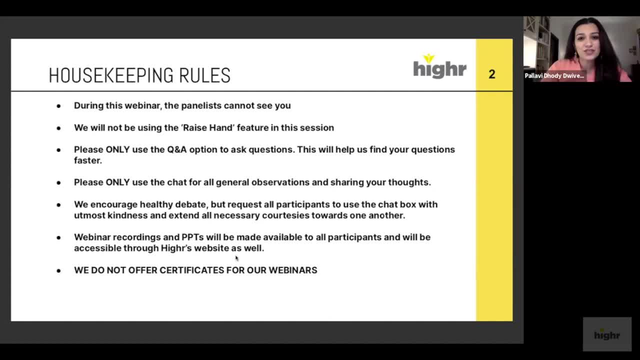 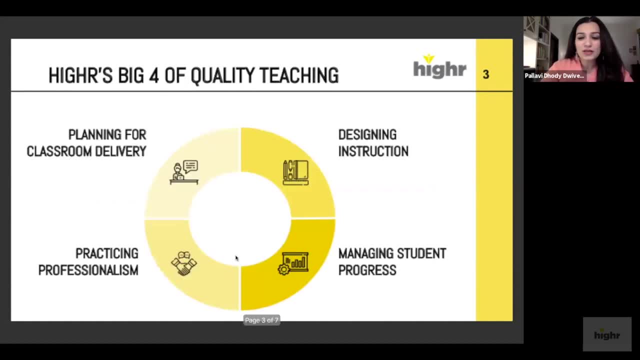 offer certified workshops, so in case you're interested in those, we request you to sign up for them on our on our website. um, so i did want to talk a little bit to you today about higher's big four of quality teaching, which is really the dna of what we do at higher and, as i was saying, everything that we do at higher. 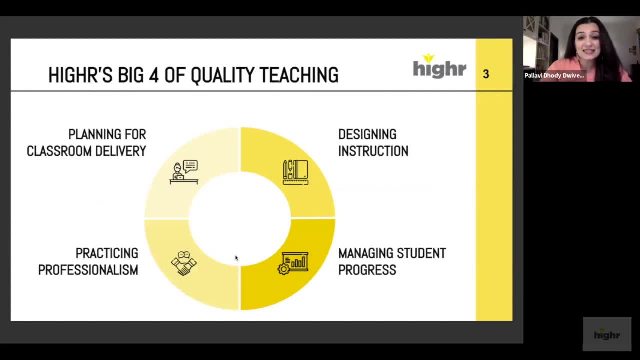 is about quality teaching and this is really encapsulated in our evaluation framework, which we call the big four of quality teaching. so all of our events, all of our workshops, all of our evaluations focus on these four key teacher competency domains, which we think are absolutely crucial for good teaching to take place. 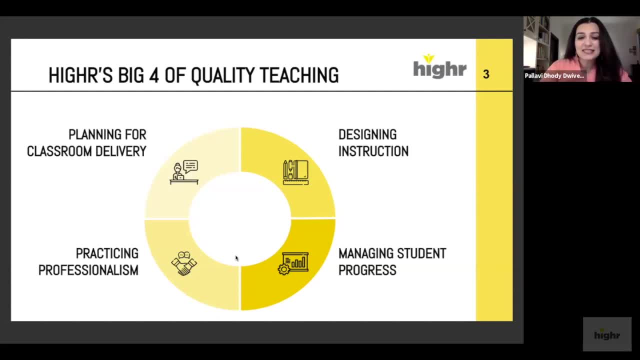 the first of these is planning for classroom delivery, the second is designing instruction, the third is managing student progress and the fourth one is practicing professionalism. every week, for all of our events, we focus on one domain of higher's big four of quality teaching, and this week we're going to be focusing on designing instruction and specifically we're 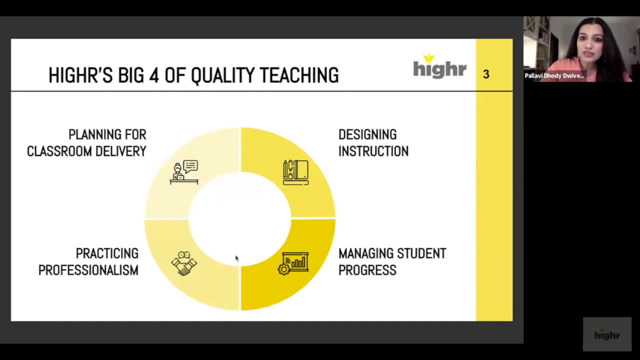 going to be focusing on designing instruction using technology for math and science. everything in the world that we see around us has uses some principle of math or science or both. how do we get our students curious about that, and how is it that we can actually use technology? 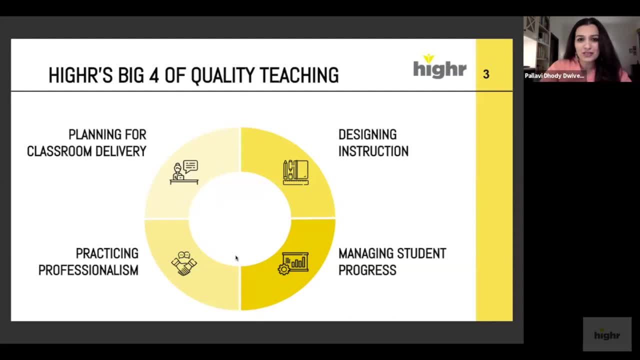 to engage our students, to pique their curiosity, to make them question or wonder about the world around us, get them interested in everything from sulfuric acid to circles to triangles, to even how sanitizers work today. and how do we use technology, because technology can really help us connect. 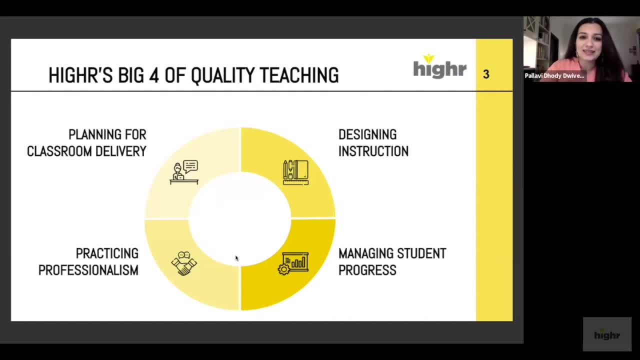 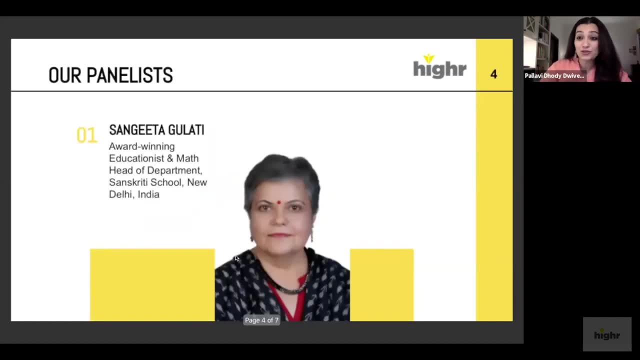 these dots and help our students see them more clearly, and that's precisely what today's panelists are going to be talking about. so, without further ado, i wanted to introduce you to all our panelists for today's session. uh, first up, i'd like you to welcome miss sangeeta gulati. uh, sangeeta. 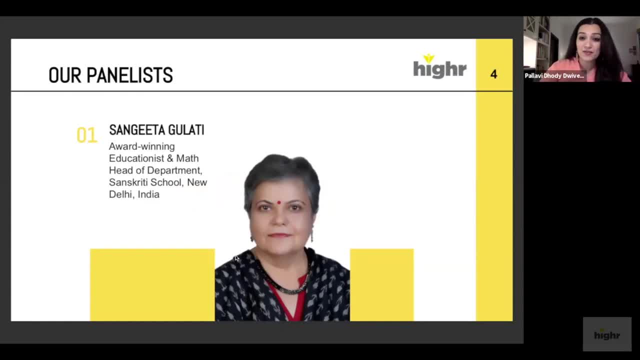 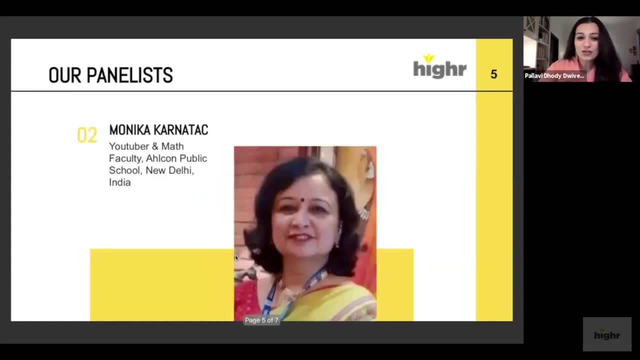 is an award-winning educationist and she's the math head of department at the sunscreen school in new delhi, india. welcome to the session, sangeeta. we also have with us uh monica karnatak. monica is an avid youtuber and she's also the math faculty at alcon public school in new delhi. 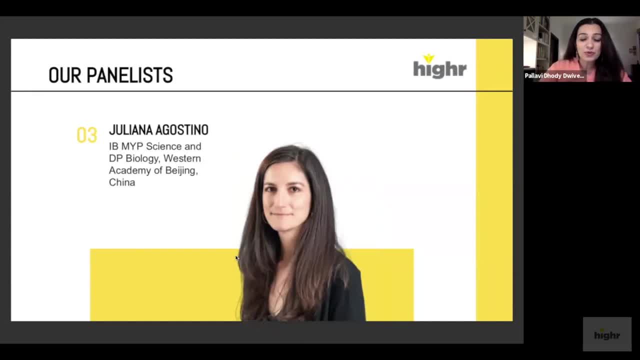 welcome to our session, monica. we also have with us all the way from canada, which is on canada time but does teach at a school in beijing. uh is juliana agostino. juliana is an myp and dp ib faculty. she teaches at the western academy of beijing in china. so lots of interesting observations. 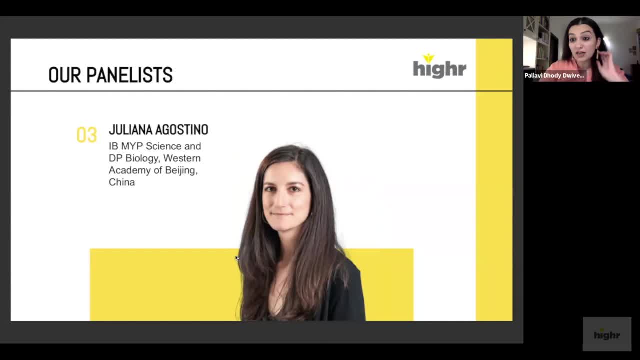 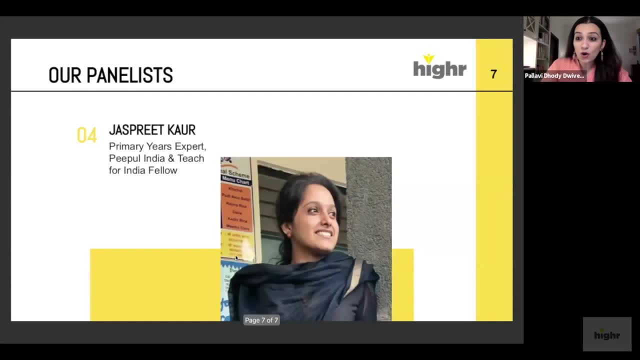 from her coming up about, uh, blended learning and where schools have reopened, uh, we also have with us uh ms jaspreet kaur. jaspreet is a teach for india fellow and she is also a primary years expert and is teaching at an stmc school with the people foundation, india. 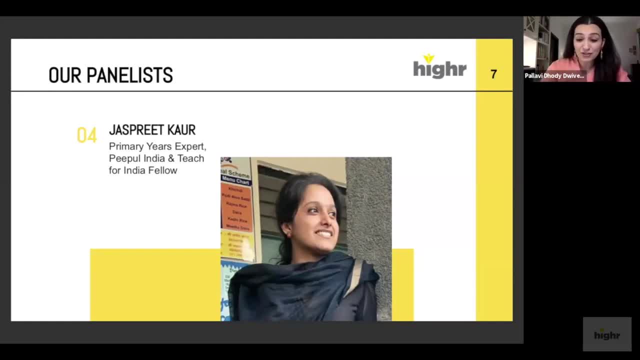 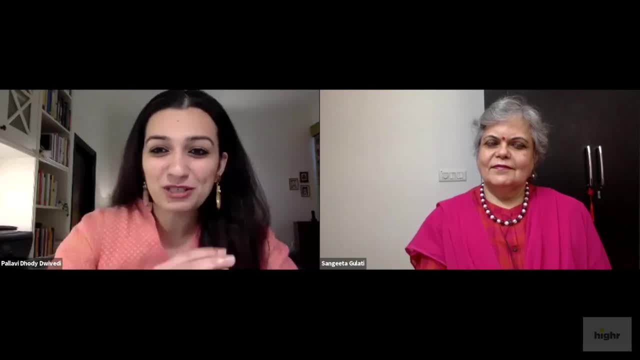 so that's our panel for today and, without further ado, i'm going to stop sharing the screen and hand over instead to our first panelist for today's uh discussion, uh, which is miss sangeeta gulati. so over to you, sangeeta, thank you. thank you, palavi, so much for your. 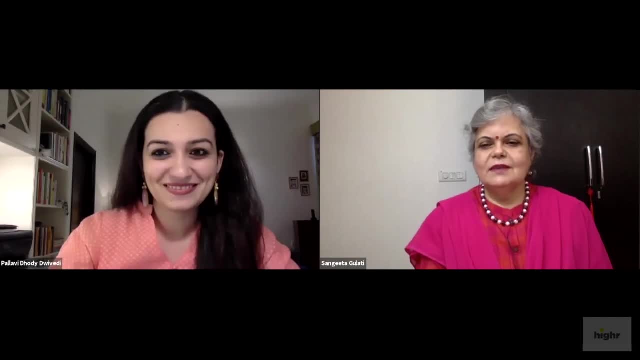 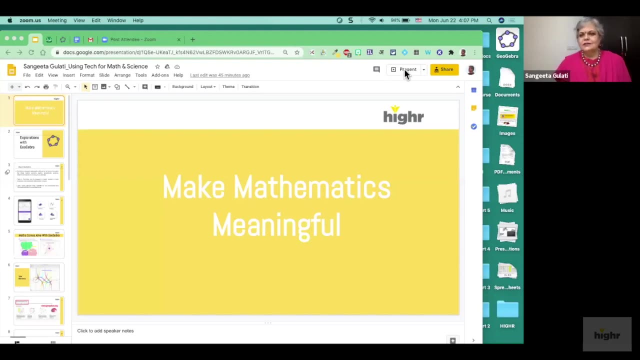 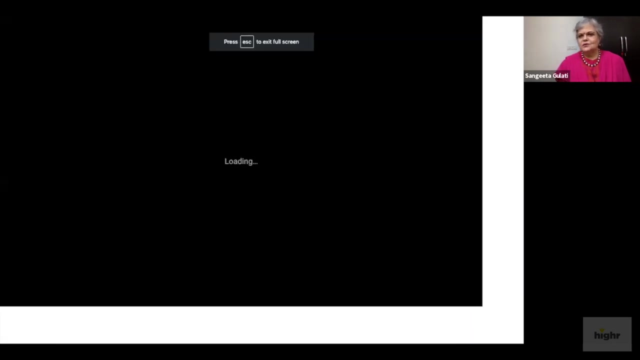 invitation to this seminar webinar and also for providing this platform uh to our teachers to share and learn from each other's experience. so it is definitely important at this time for each one of us to open our experiences uh and share with each other so that we can. 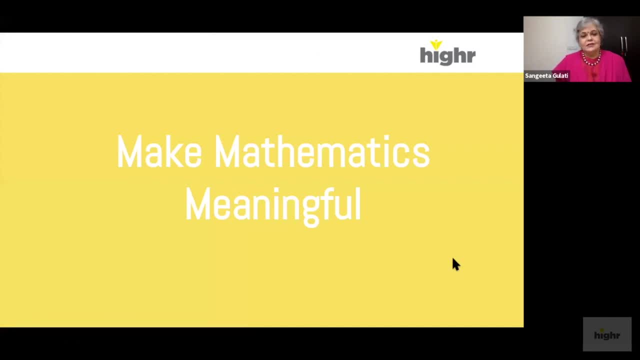 all learn and grow together. uh, and, as you said, yes, maths, when we think about uh, does has its own challenges and, as far as the maths curriculum goes, uh, we very often teach our students to do maths and the assessment gears more around finding, solving and, of course, 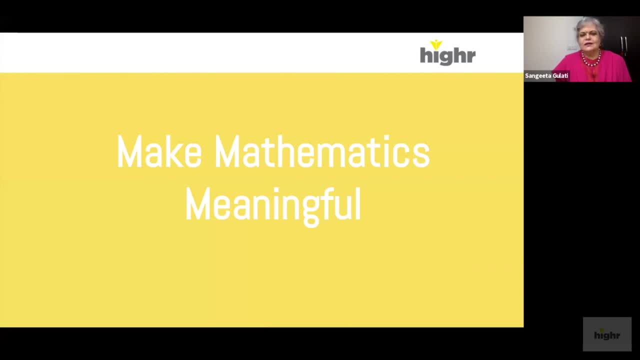 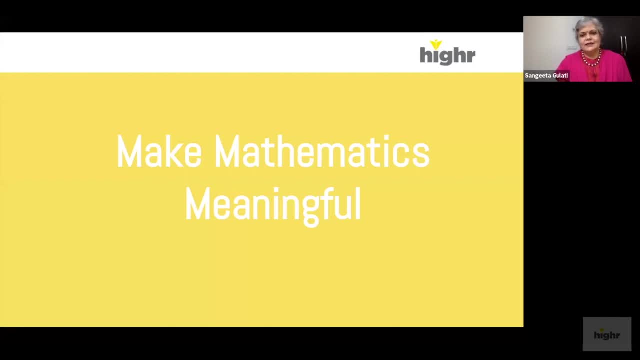 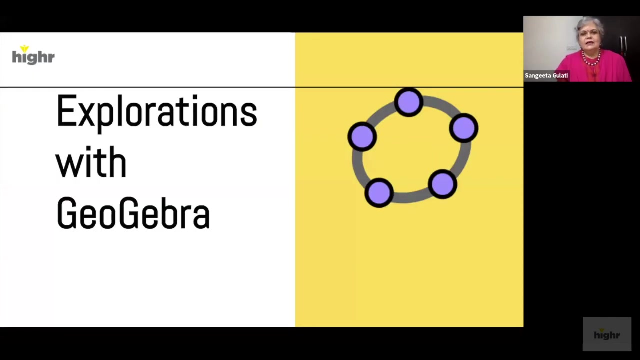 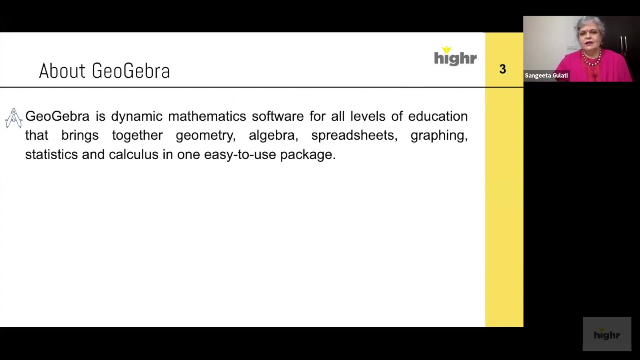 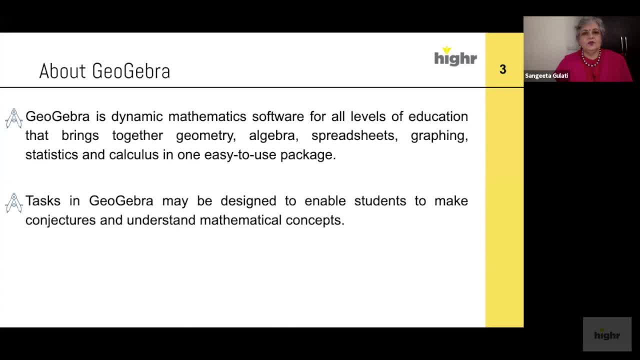 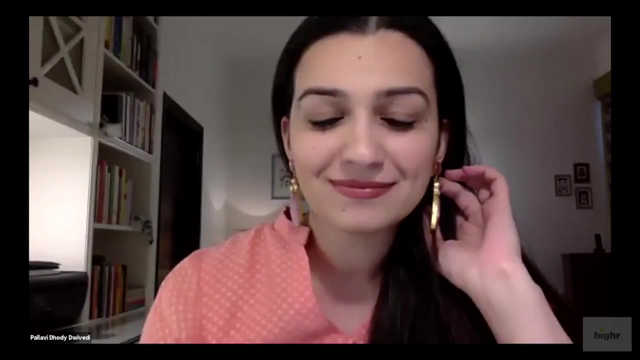 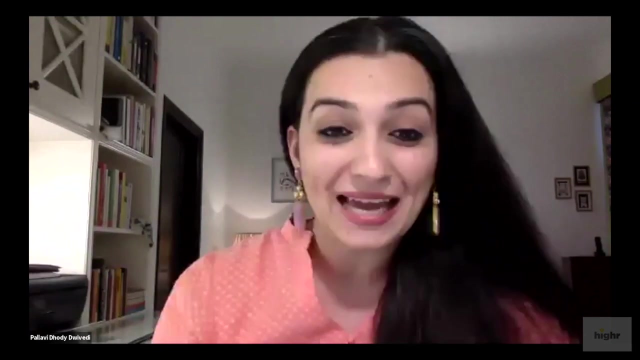 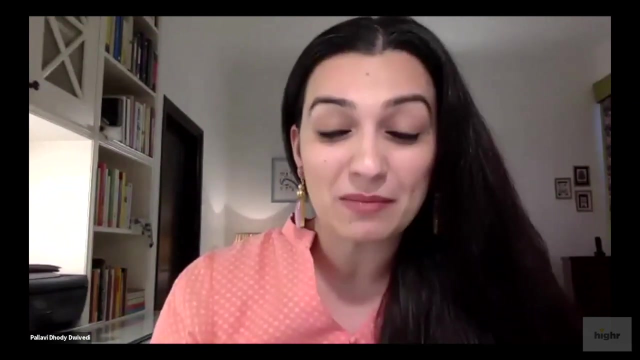 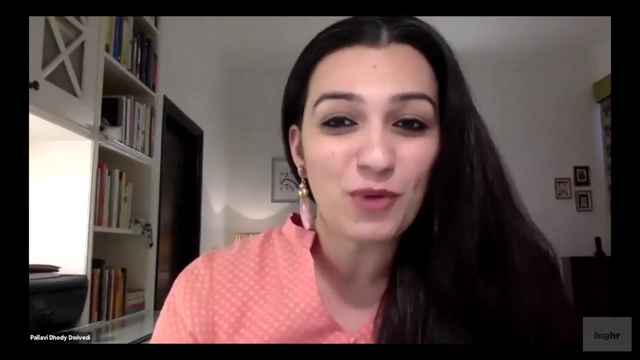 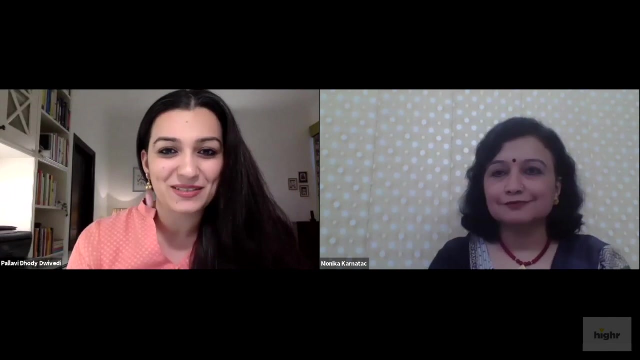 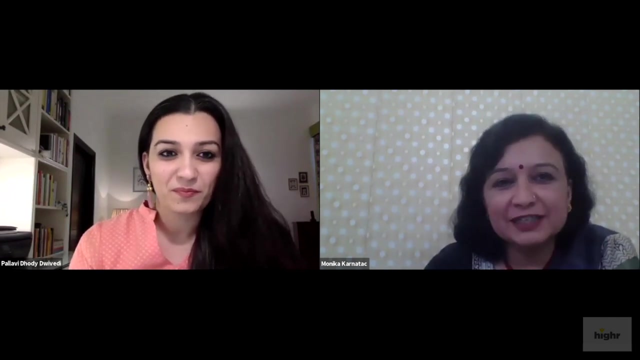 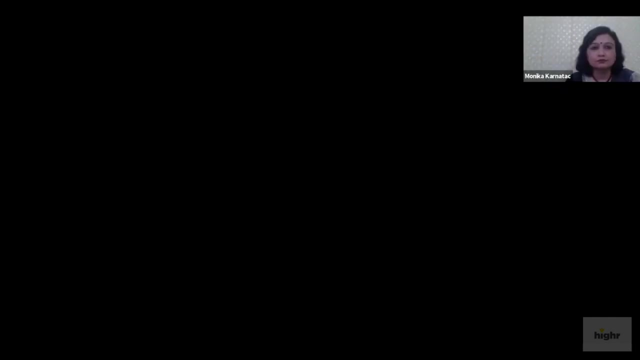 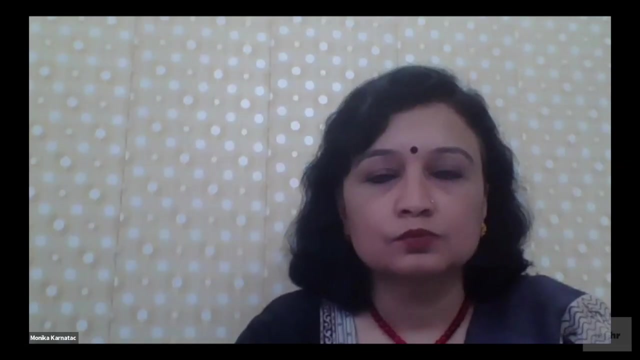 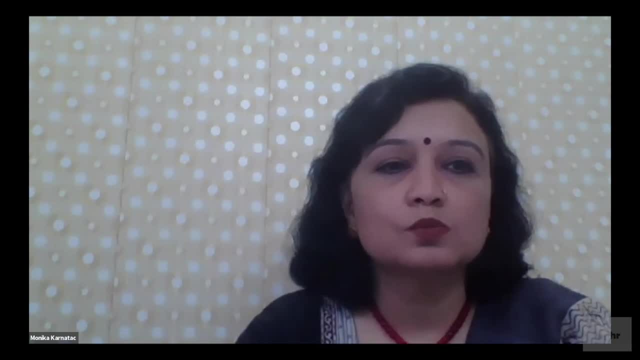 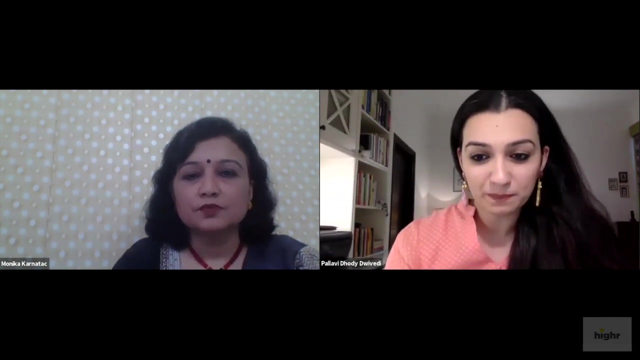 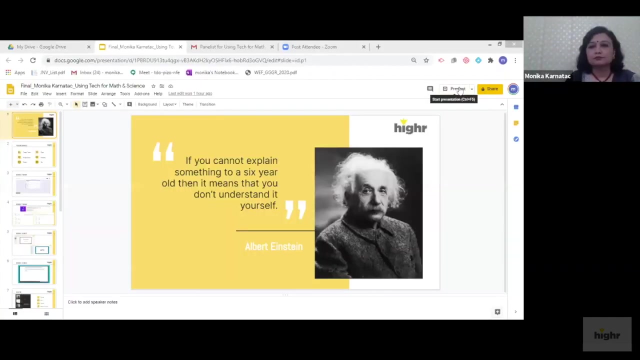 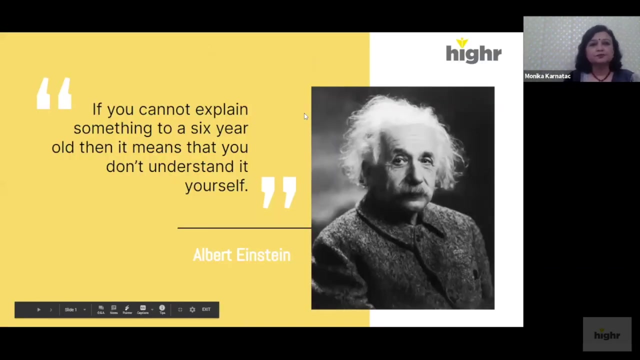 Monica, would you like me to share your screen instead? no, no, no, I'm just sharing just a second. yes, are you able to see? yes, yeah, go right ahead. a very good evening to one and all present. the great scientist Albert Einstein once said that if you can't explain something to a six-year-old, 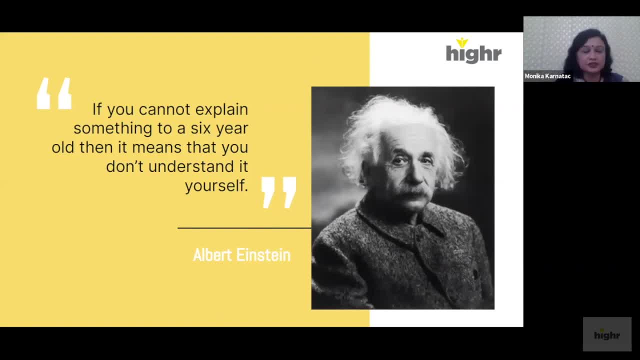 then it means that you don't understand it yourself. and in today's time, I believe that we all are playing dual roles: that of teachers and of a six-year-old. we all are finding of a way, through technology, by ensuring that we are doing justice to our 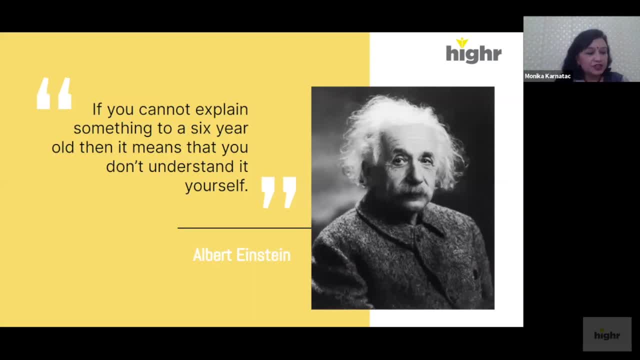 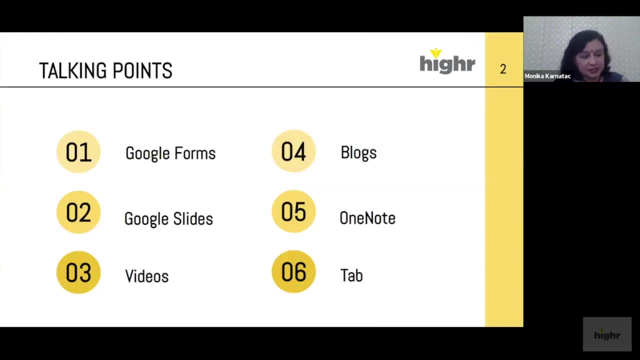 students. before I begin, I would like to take this opportunity to thank higher Pallavi and all of you who are attending the session discussion. I believe that this is a great platform where we all can learn from each other and learn from each other, and learn from each other and learn from each other. 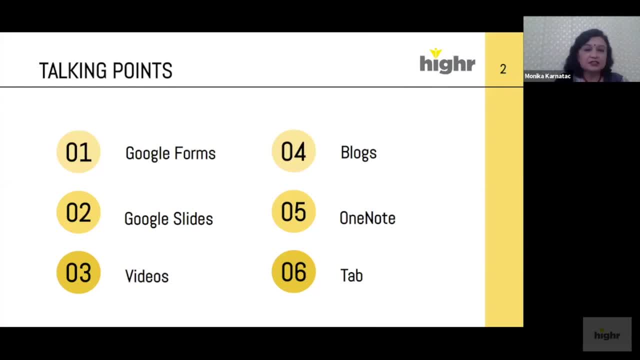 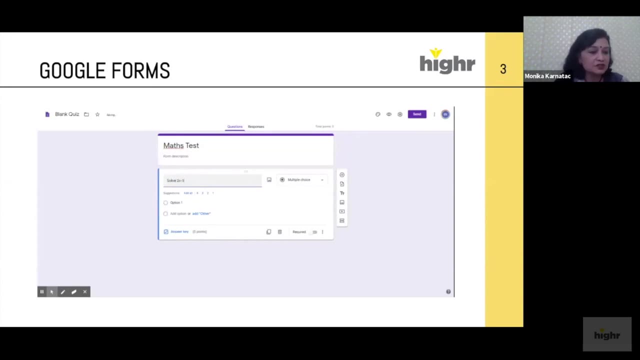 how to increase digital literacy and its impact. one resource that I have extensively used in the past one month is Google Forms. Google Forms can be used to create tests and quizzes for students. after every class, you can give your students a link to a form which has a number of questions. 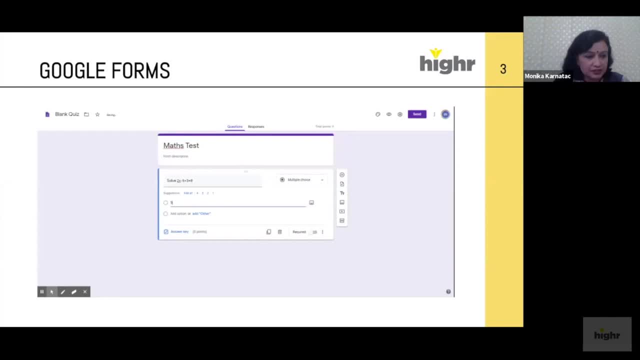 we can add questions of our choices. and we can add questions of our choices and we can add questions. we can make them tough or engaging, as per our liking. these questions can be such that they allow students to engage more with the topic and generate their curiosity. once the topic, once. 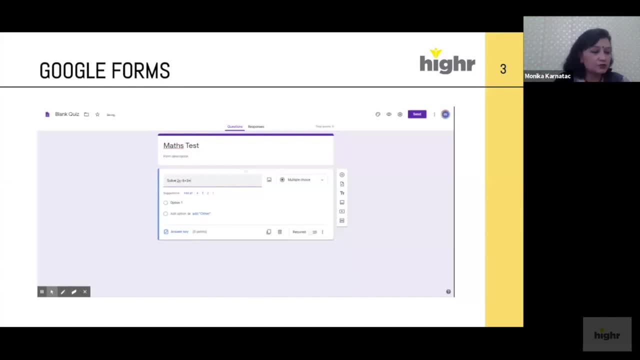 the student attempt the questions. based on their performance, we can analyze how effective our class was, what the students understood and what they didn't. just by looking at the responses we can make out this: that whether the student have understood step one, step two, and then you can. 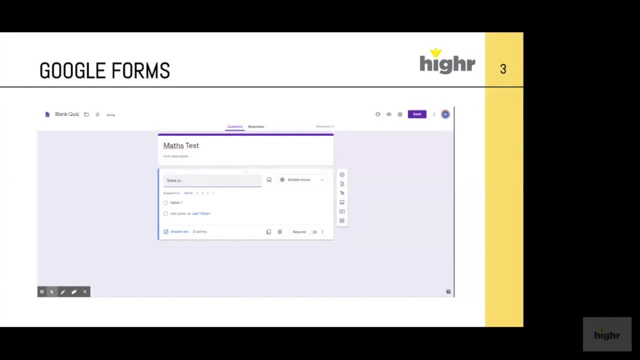 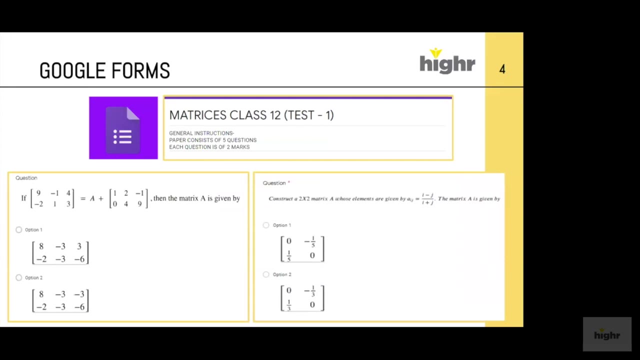 discuss it with the student. by analyzing what answers each of the students selected, we can make a guess about what concepts were clear to them and what wasn't. I particularly find Google Forms resourceful for maths teachers when used with EquatIO. there is nothing more comfortable for us. EquatIO is a 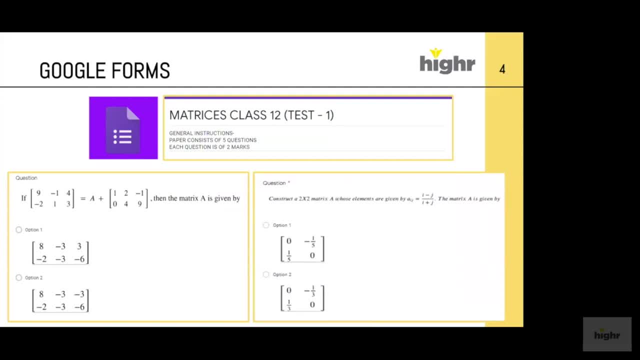 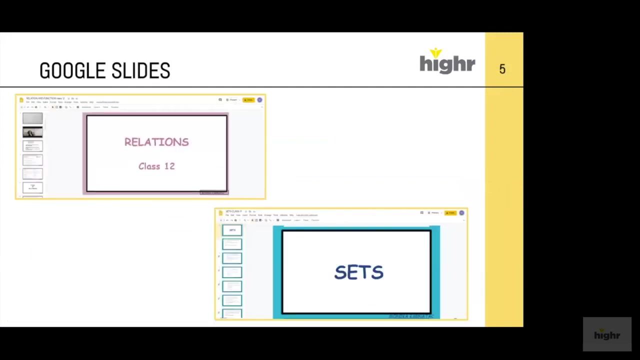 software that allows easy typing of math symbols and equation. Sangeetha man will show how it is very much how the life has become very comfortable using the app EquatIO. once a teacher starts using it, I'm sure leaving it will not be an option- another important resource while teaching. 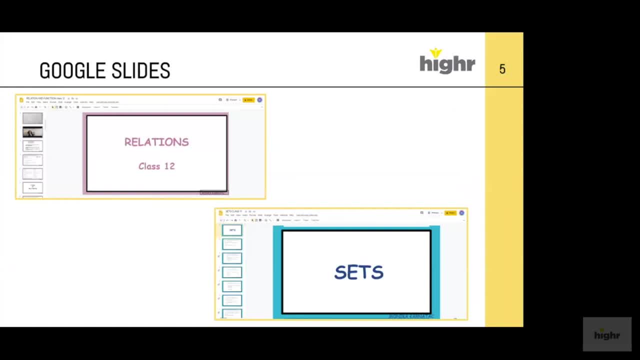 students online is Google slides. just like PowerPoint in Microsoft, Google slides can be used to make presentations. the difference between the two is that we can share your Google slides any with anyone using a simple link. different people can collaborate to a single slide from anywhere in it. you can embed videos, present text of 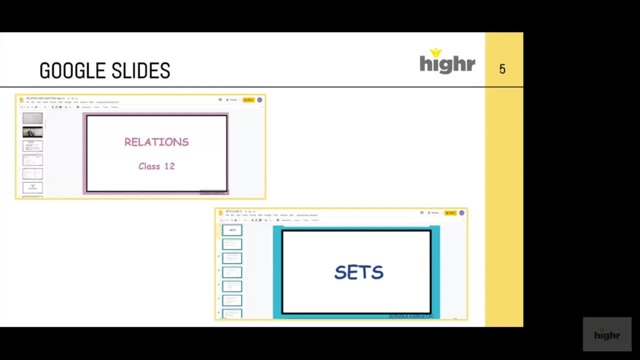 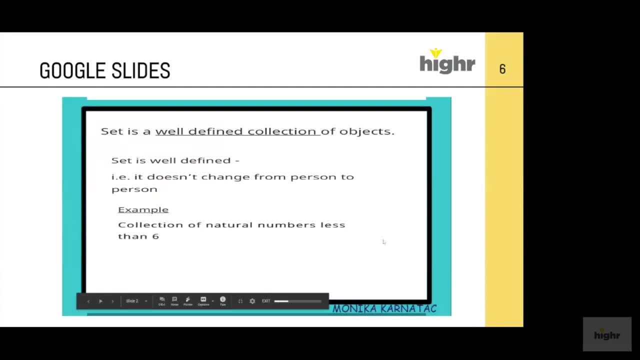 your choice, insert images, tables, graphs and mathematical symbols. it also allows you to use animation that can make your class more interactive and generate the interest of your students. one way of doing this is to animate in such a way that the questions appeared on the screen first, then we wait for the. 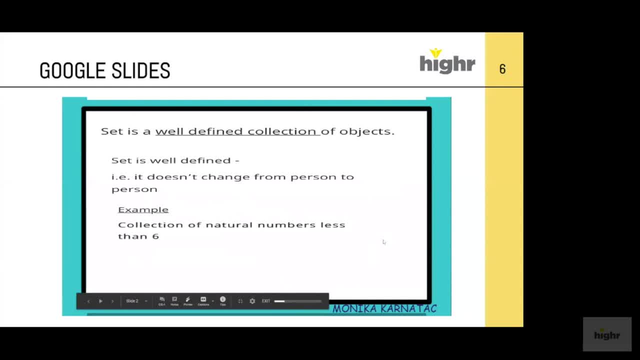 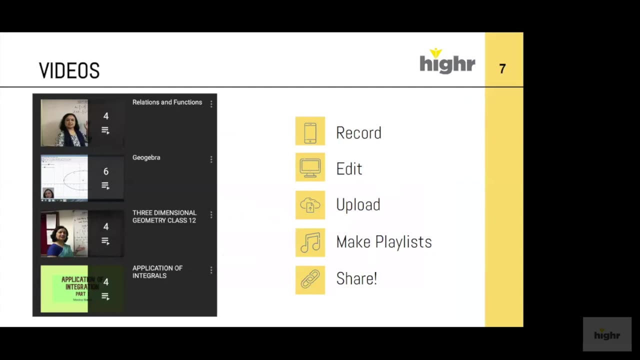 students to think and answer and after that make the answers appear, or you can embed videos. anything you want that Google slides permit you to do it. another digital tool that I found useful is the have extensively used in past are videos. making videos is easier than we think. it is all you need. 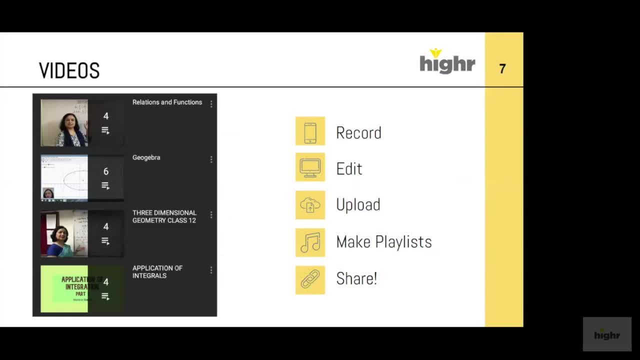 is a phone. you can shoot on it and even edit on it as well. just go to the play store and you will find many free video editing software. or you can edit on your laptop, like i have been using it. the software the power director i am being using. another useful resources resource is screen. 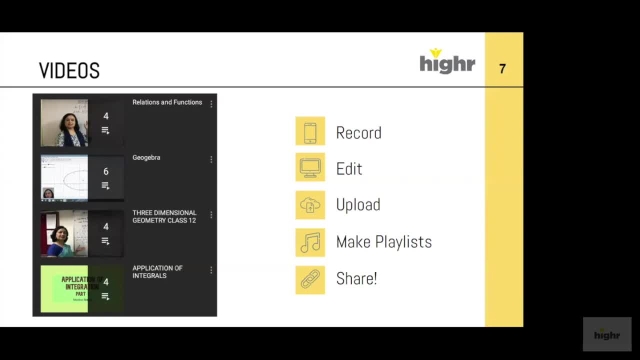 castify a software that allows you to record your screen and make small videos for free. what i like to do is to take small topic record myself while i'm teaching. then i upload these videos on youtube. i make playlist which collect all the subtopics into one. videos are a great. 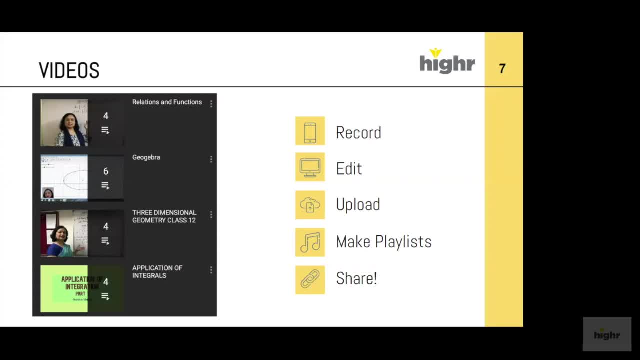 way to do that. so i like to take small topic and record those videos, all the subtopics, into one, to enhance asynchronous learning. they help the students to revise or to go back to a concept that they haven't fully understood, and videos can help them to make a digital archive of your own. 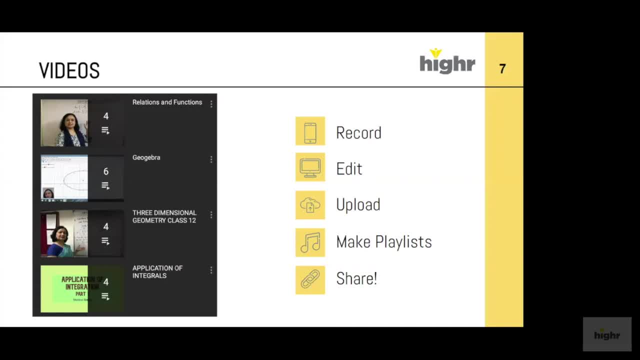 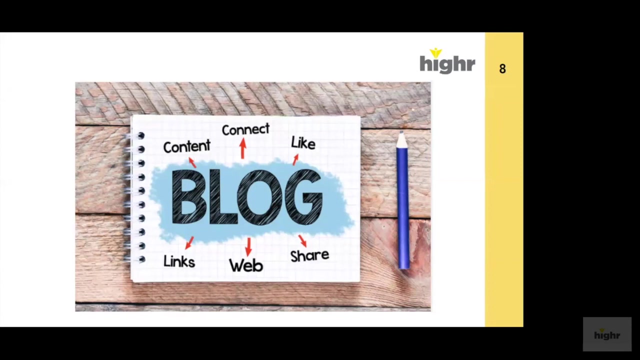 they can be assessed by anyone anywhere. through just a link, you can share them with your students or colleagues on whatsapp, mail or through any other platform. it's like your small portfolio present out there for the world. i would now like to talk a little about blogs. a blog is: 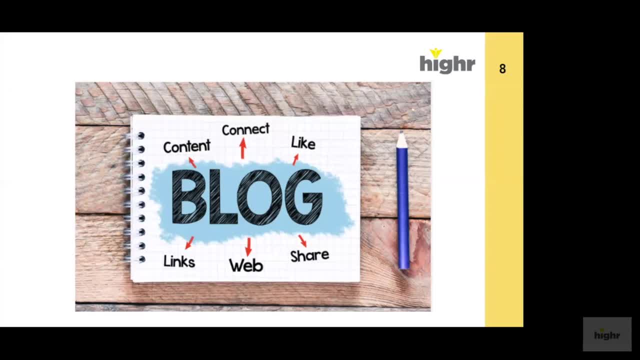 like a personalized website of your own where you can add any material that you want. there are many sites on the internet that allows you to upload and organize your page and share your materials. For example, I use WordPress, which is a free website You can create. 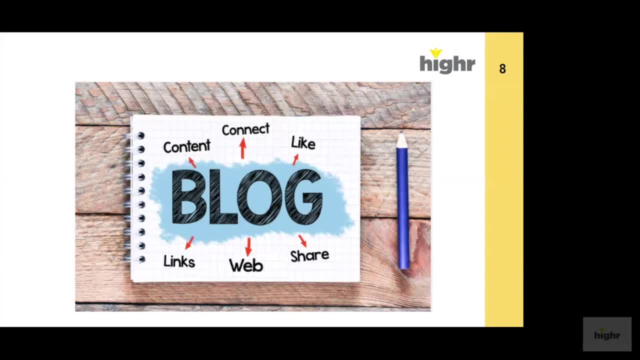 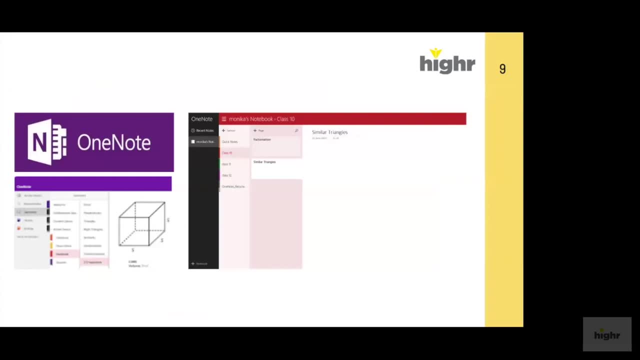 your own custom name, add your material and then send the link to your student. A resource that I have recently discovered is Microsoft OneNote. I like to see it as a digital notebook and it is very useful resource to teach maths or any other subject. You can embed PDFs, images, videos and 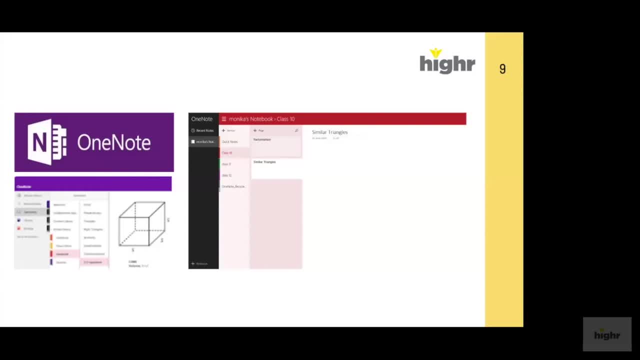 annotate on it. It helps you organize your lecture by dividing it into different sections using pages and sub pages, and you can then share a link of the same to your students and ask the students to share a link of their notebook so that you can be updated about their 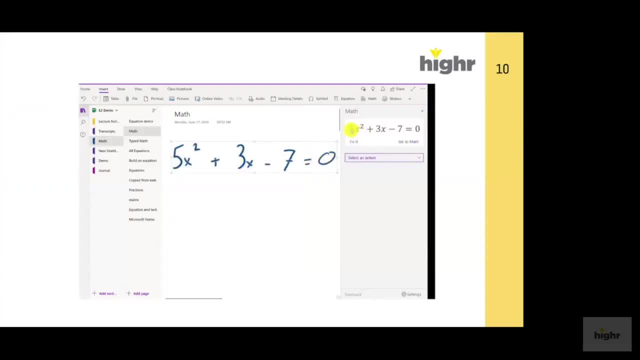 program OneNote becomes even more helpful if you use a graphical tab or a digital pen. You can just write any complex maths equation using your tab, or OneNote will convert it to text using the feature Ink to Text, and it can also create stimulating graphs based on the same. This visual depiction can allow your 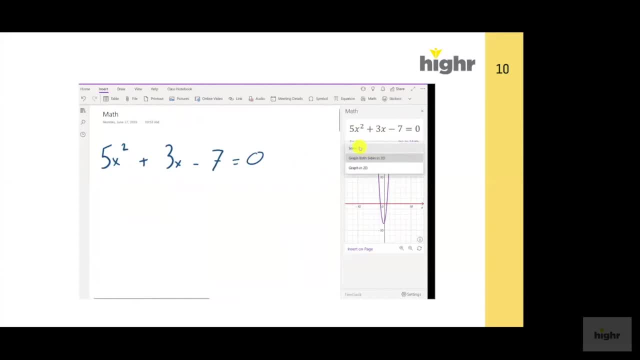 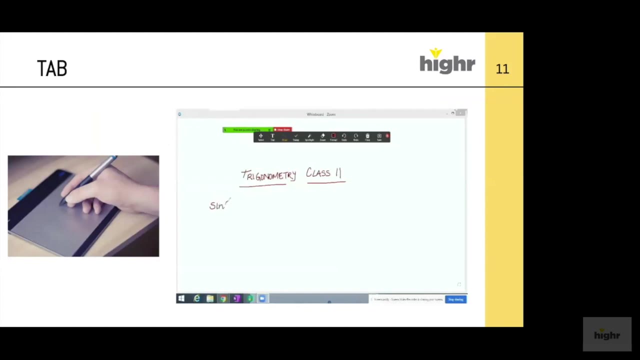 students to better visualize the change in their learning process. change in graphs as you keep changing the values Based on the same steps for the solution can also be seen. Now I would like to talk a little bit about graphic tab. So I recently brought one myself and it has made life so much. 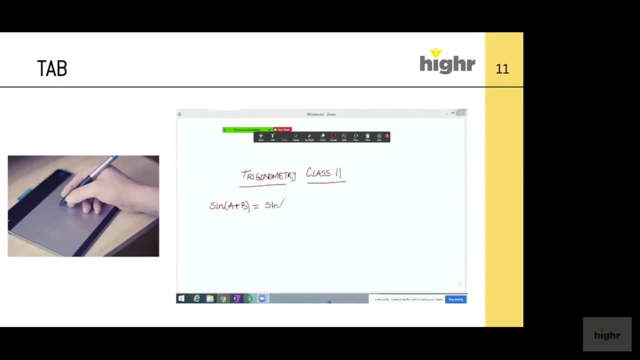 easier. My decision to buy the tab was stemmed from the fact that, as a maths teacher, I was facing the problem of writing the complex equations. Even if I would annotate on zoom whatever I wrote for one class, I could not store it once the meeting ended. Using the tab on OneNote, I can save everything I write. I 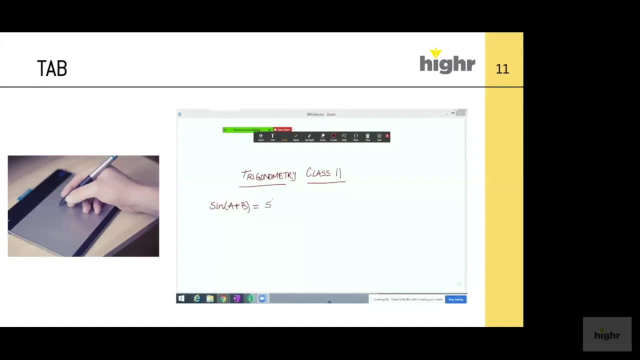 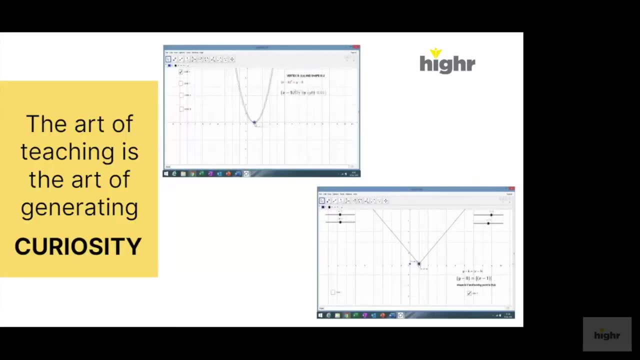 can even use it to annotate on zoom or meet by sharing my screen. One more thing: I want to tell that last year I had conducted a study to analyze the effects of using technology on students performance. For the same, I divided my class into two groups, consisting of students who have scored 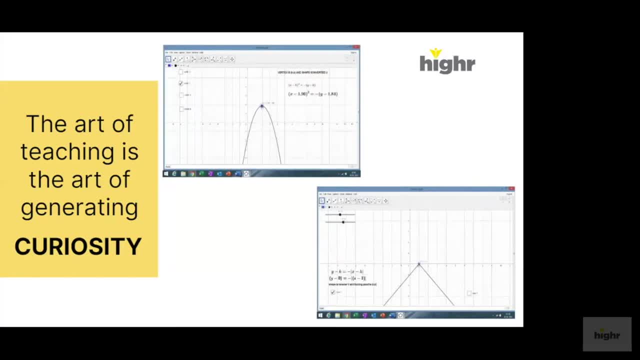 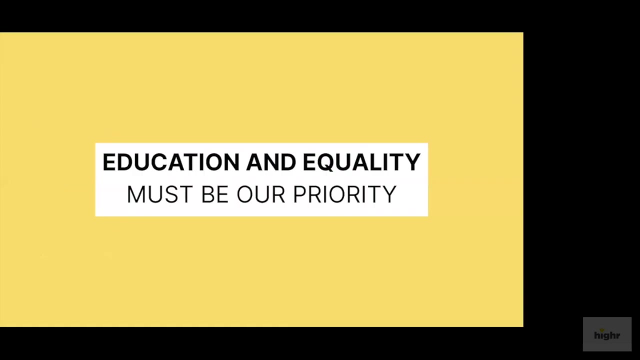 60 to 75 marks To one group. I showed videos for each topic after every class and after the study. I analyzed the result and found that the group that was taught using technology had seen an improve in their performance and accuracy performance. The pandemic has brought extremely tough and challenging times for each of us. 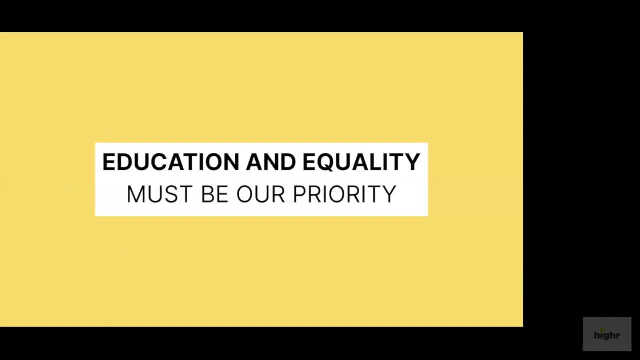 It has made us teachers explore and utilize the digital realm. I see this shift of technology as a positive term. It has challenged us to constantly evolve, to find new tools and ways to engage with our students and generate their interest. But even as I say that, I would also 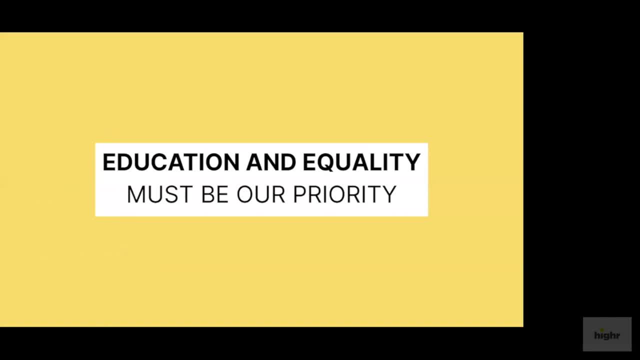 like to mention that only a very small amount of students have access to technology, A stable internet connection. gadgets and a space to use them are still unaffordable for many, So it is important that we, as teachers, continue to be humans and not become robots. It is important. 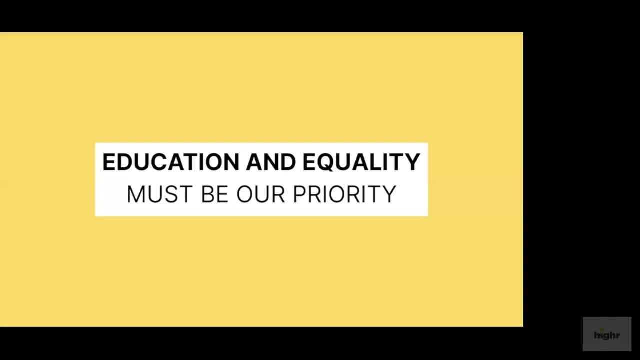 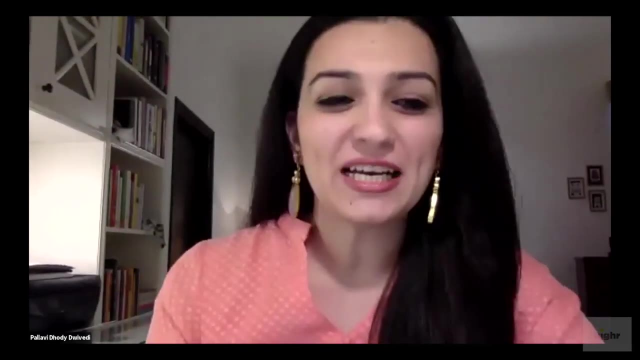 that we respond to the needs and situation of each of our students. I hope we continue to learn from them And from each other. Thank you, I just hand over to Pallavi Monica. thank you so much for that. Some very, very interesting suggestions coming in. 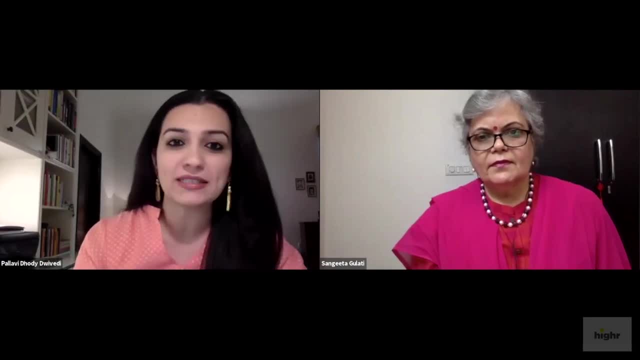 And especially liked the fact that you were able to talk to us a little bit about using our tabs. And there was a question, Monica, if you'd like to take that on- where somebody was asking what tab it is that you have bought and which one are you using. If you could just let me know. 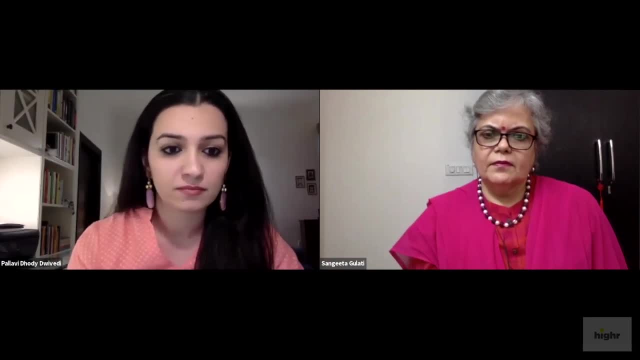 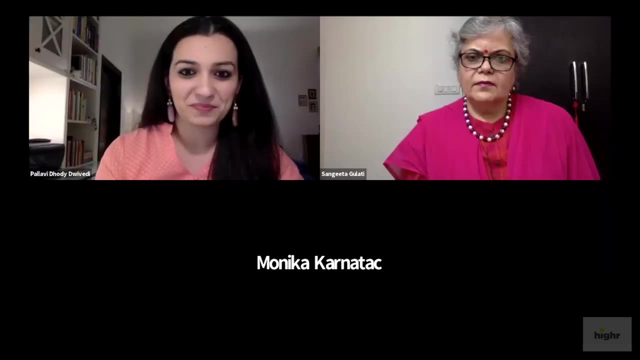 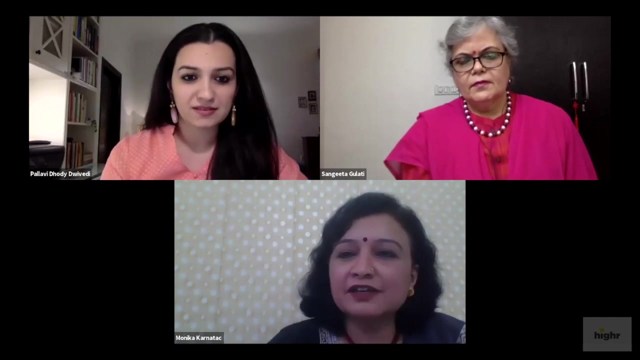 I am using. can you switch on my video please? Oh sure, Yeah, I am using a very simple tab, Very simple, It was just for 3,700.. You can use it for writing And otherwise it starts from 3,000 to 3,000,000.. 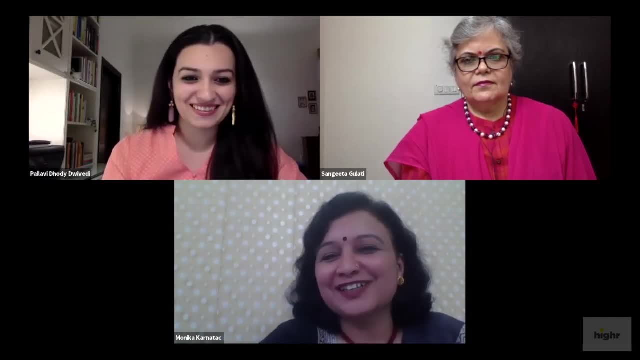 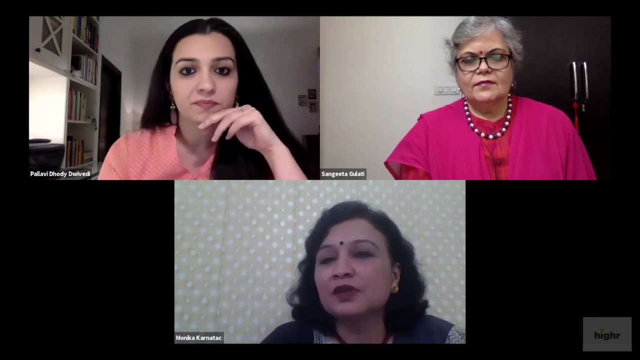 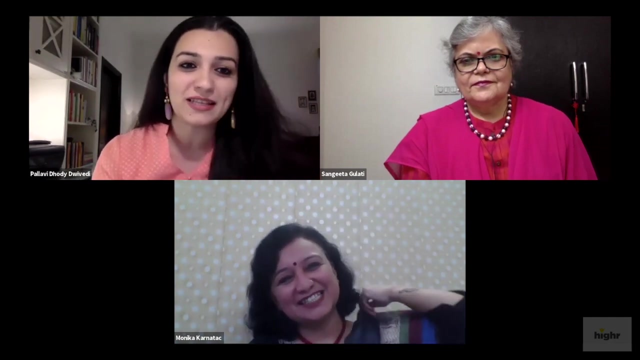 So so. so varieties: There are so much of types, Okay, But you can go for a very simple too, depending upon your need as well as your pocket allows. Very, very true, And that's a very important consideration also at this point in time. 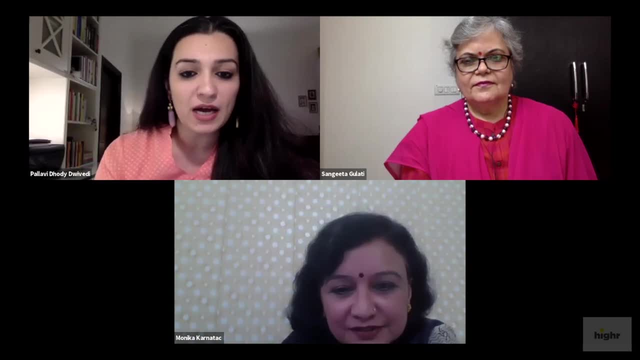 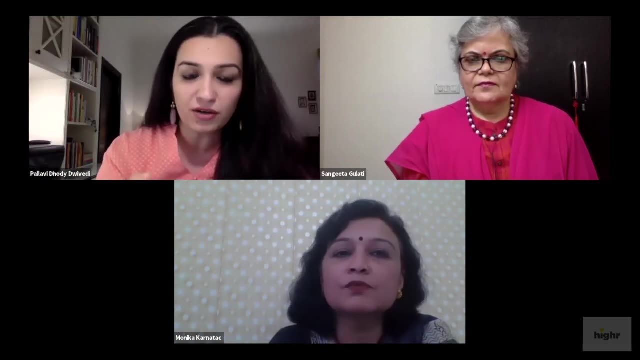 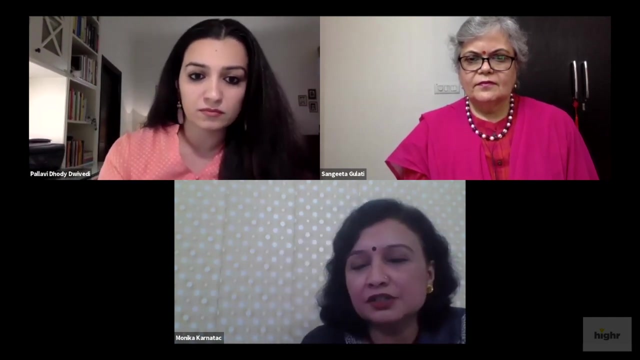 There was another question, Monica, about the app that you mentioned. I think the one that you were talking about is EquatIO, And I think Salida ma'am is also going to be talking about that as we go further. Yeah, Actually, Salida ma'am will elaborate on EquatIO. It is a very useful app provided by Google. 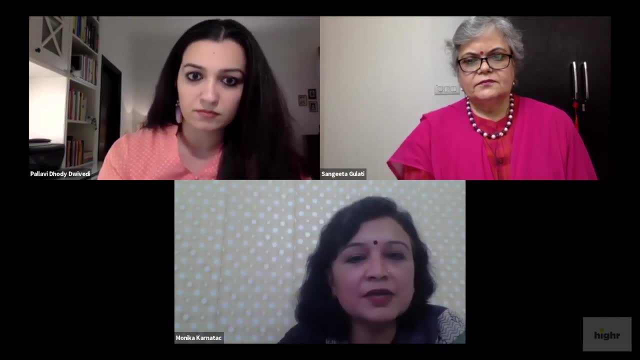 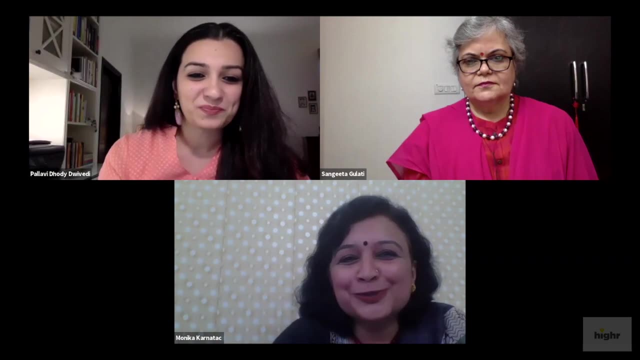 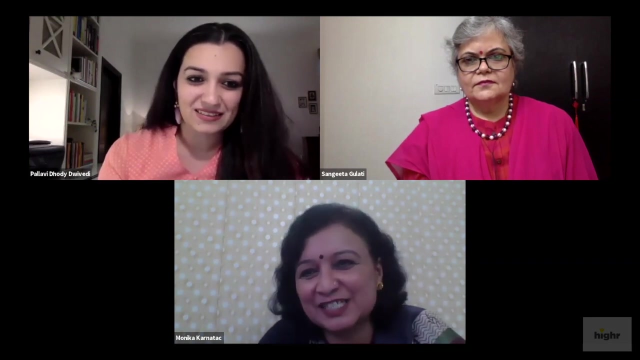 Once you have started, because I also started after attending Salida ma'am's workshop- and once I have started I cannot think of leaving it. But our school is not a Google-certified school, so we have to pay for it. Otherwise, if the school is Google-certified, then the teacher will get access to that. 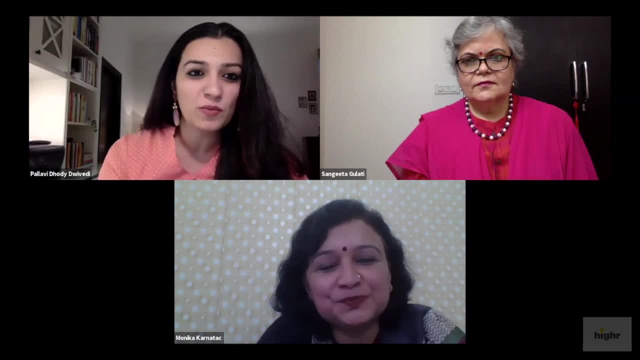 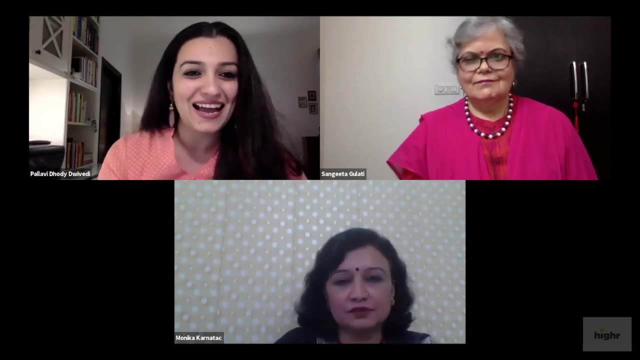 Understood. Okay, fantastic. Thank you so much for that, Monica, Moving on very quickly over back to where Sangeeta had left us and unfortunately she dropped off. So just if you could just get back to where she was, So over to you. 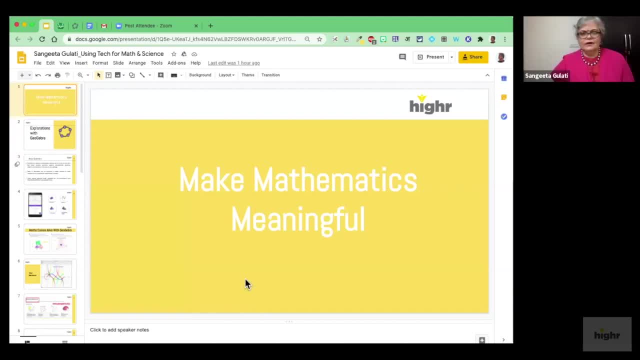 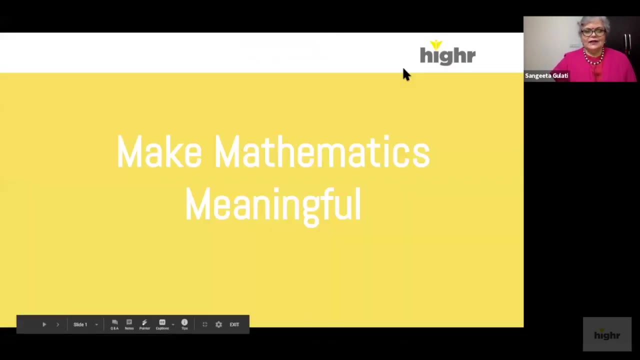 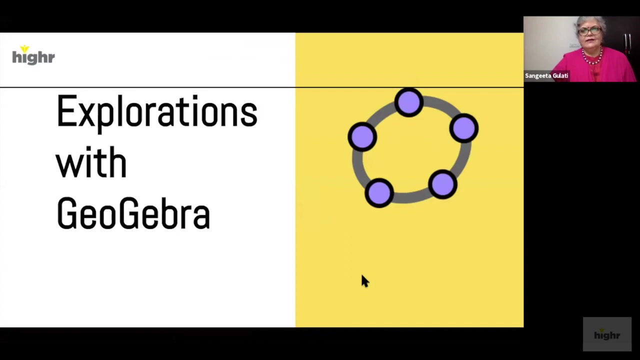 Yeah, sorry Again. technology always brings with it its positives as well. as you know, you have to have electricity to run technology. Yeah, Yeah, Technology. So that is why I had to kind of step out of the ball So very quickly, moving on to where I was. I had just started and, as I was talking about GeoGebra, which is one of the favorite and well-known app for maths, 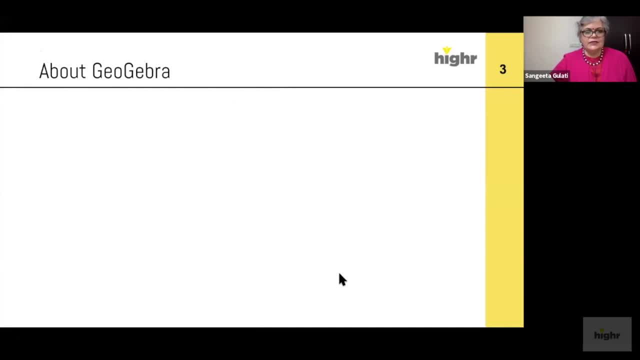 And, as I said, it really has changed the way that we teach and understand mathematics. So it's a dynamic mathematics software which goes very well for all levels of classes, as one look at it, whether it is school or higher education. It works for geometry, algebra, graphing, calculus, you name it. you can do wonders with it. 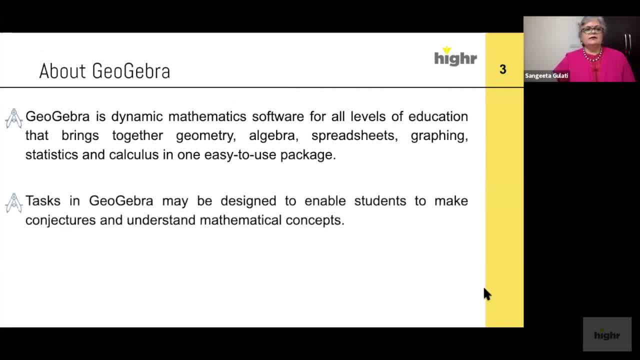 And what it also allows you to do is basically let you, as a teacher, create certain opportunities which would allow students to experience maths, make conjectures and also embrace maths in a different way. What we are also looking at is the greatest benefit of GeoGebra to be an open source software. 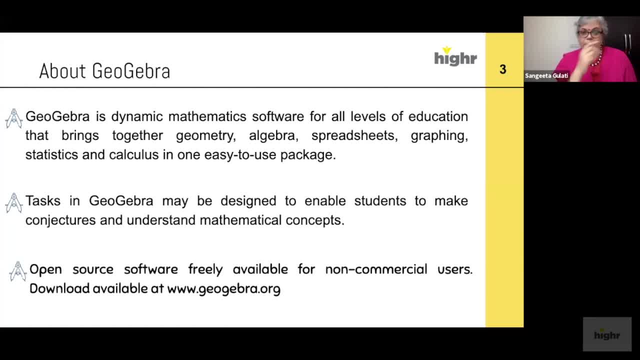 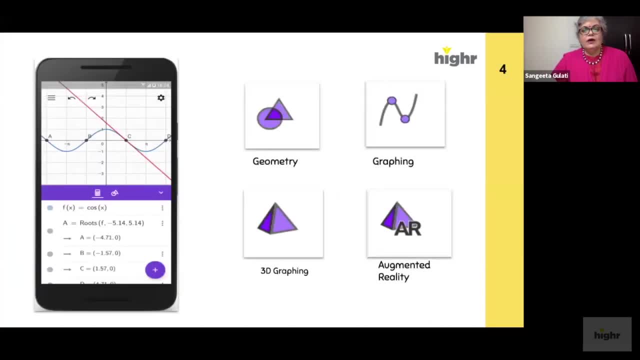 So you can download it, you can carry it in your- you know- pen drive, put it in multiple systems And, of course, the online version is equally powerful. Also, the mobile apps for GeoGebra are very powerful. They're very versatile. 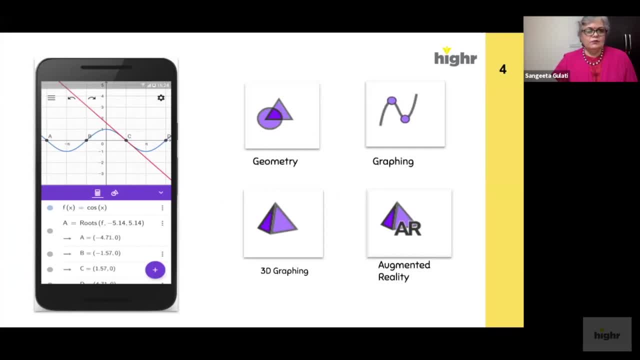 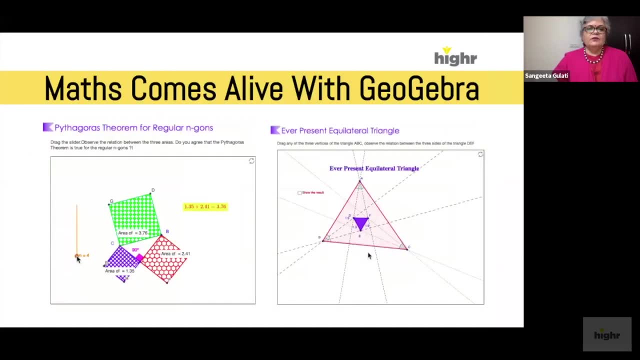 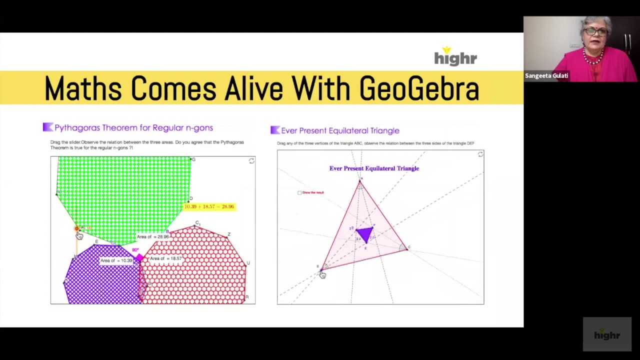 And therefore, you know anyone who, depending on where you are in the world, anyone who, depending on your need, can use it in whichever way works best for you. When I think of GeoGebra, then the only way that I can express as to what it can do is to say that it brings maths alive. 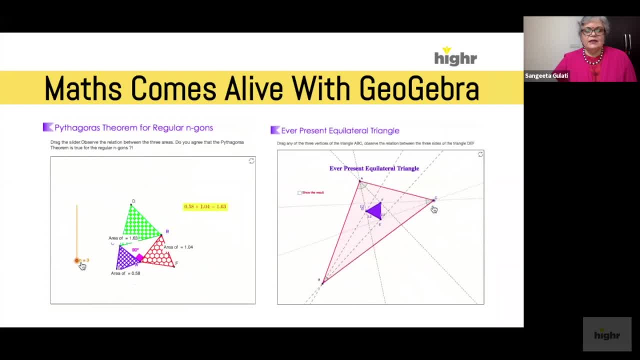 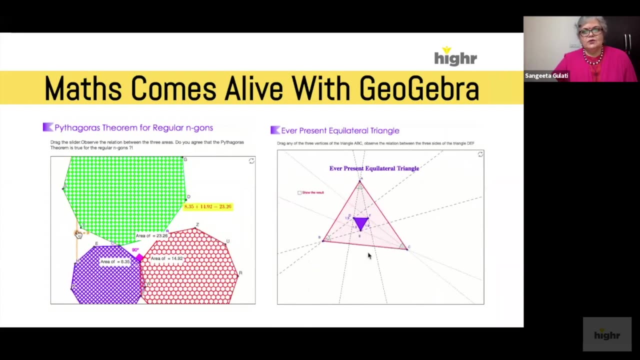 And, as you can see in these two short apps that have been added in, it really brings life to maths, So it allows you to look at Pythagoras theorem in a completely new direction. So Pythagoras theorem for regular n-gons is something which I could only explore or think about when I started using GeoGebra. 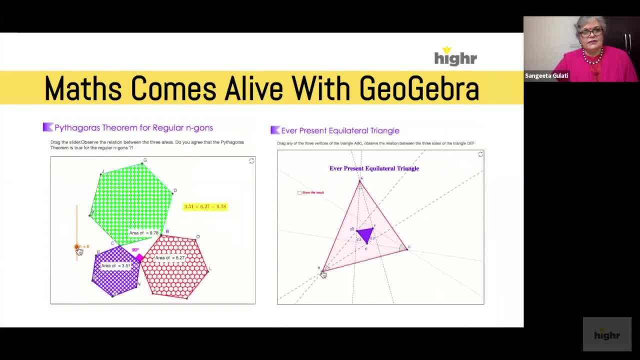 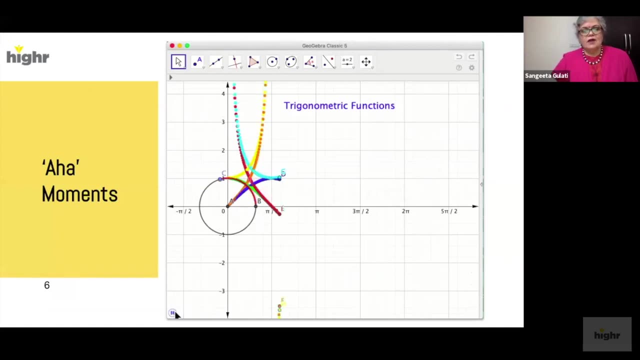 And also discovering those geometric wonders. But at the same time, everything that we teach at school level can be very well synced and can be used with GeoGebra. Teaching, in fact, pre-calculus and calculus is now so much of a joy. 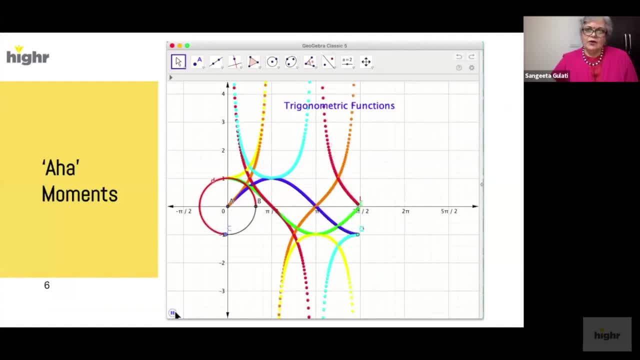 Because it lets me learn, Because it lets me take these abstract concepts and make them more visual And create those aha movements which each teacher looks forward to. So, when we think about GeoGebra, one thing that I need to say and show is that we need not be an expert or a master of GeoGebra. 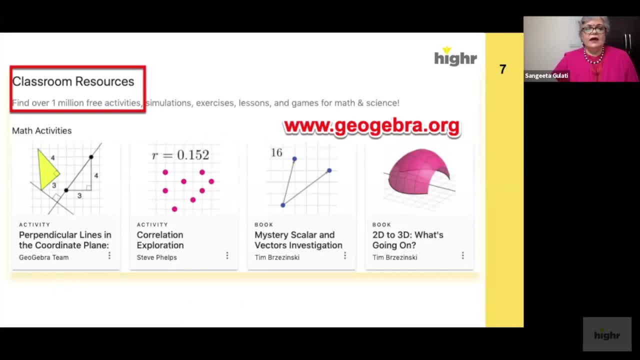 GeoGebra website itself has over 1 million free activities, exercises, games, simulations, which are free for you to use as they are, or you can even edit them and then use. You can download them as well And, in the last 15 days, considering the situation of remote learning, that we are looking all around the world. 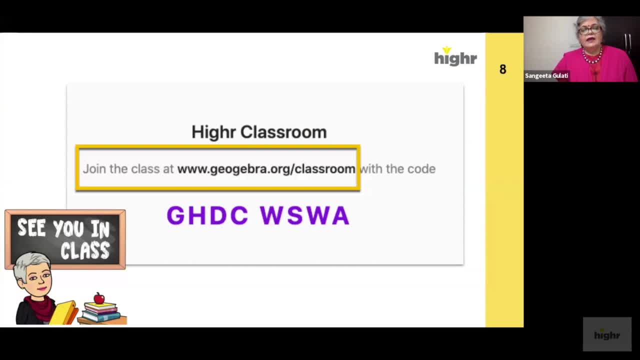 GeoGebra brought in a fantastic update, And they have brought in something known as GeoGebra Classroom, Which basically allows you to give the scores to which I am opening it right now, To the audience. Make a note of it quickly and go to this: wwwgeogebraorg. 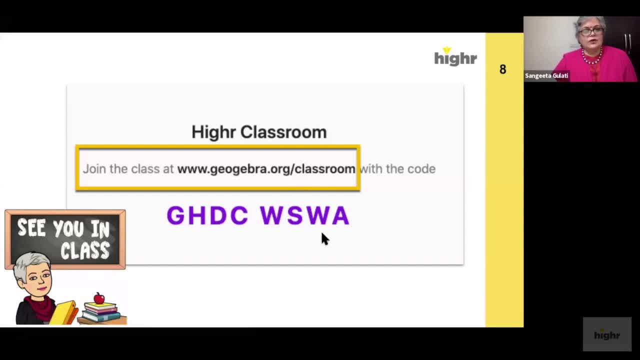 slash classroom and type in this code and you will be able to join in my classroom, which I have called All Credit to Pallavi Higher Classroom. So this is your classroom, where a task is assigned to you, And what this task basically could be is a mix of GeoGebra constructions, applets. 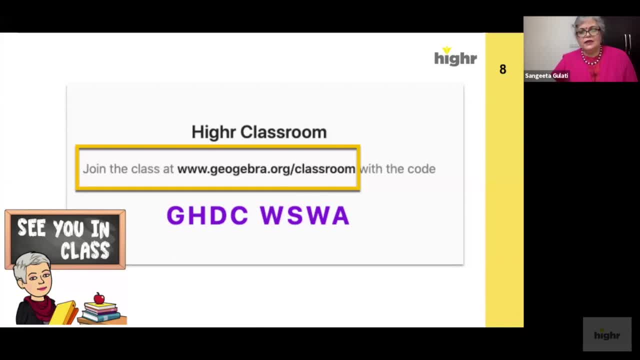 which are kind of self, very well self explained and also certain questions. So as you work on it as a student work on it, the teacher remotely will be able to get a live feel of it. So we don't have time to do that in the live mode. 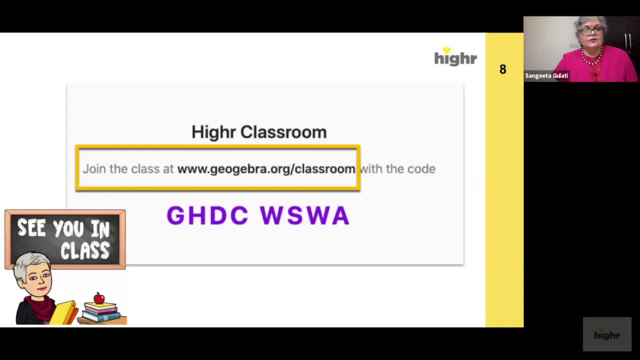 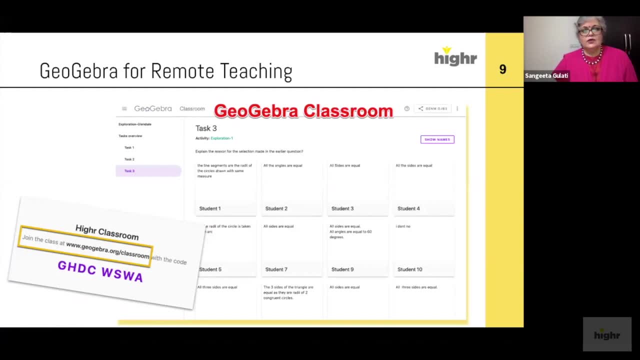 but this is open to you to try and get a feel of it. So what it allows me, as a teacher, to do is, as you join in, your tiles will start showing up on my screen On my screen, as it is doing right now here. 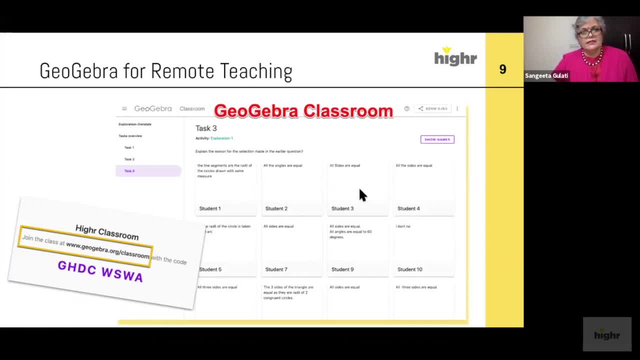 And I can actually follow the work of the student as they work along with me. I can discuss this work that is, coming up and do maths, I can teach maths and I can discuss maths, and I can also guide the students in a live mode. 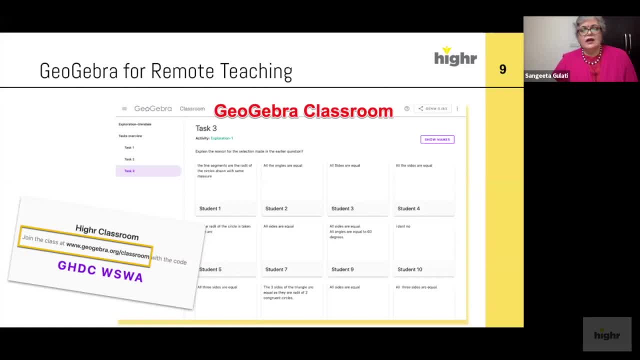 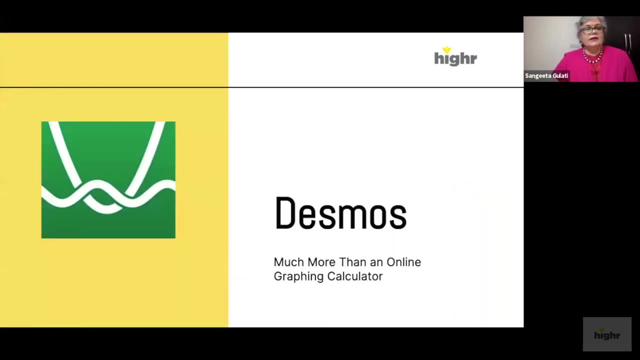 So this definitely was much asked for and much in the need of time And they have come up- absolutely awesome Time for us to use it. So this is something which you can definitely try using with as you go along in your lesson plans. Another software which I completely in love with is Desmos. 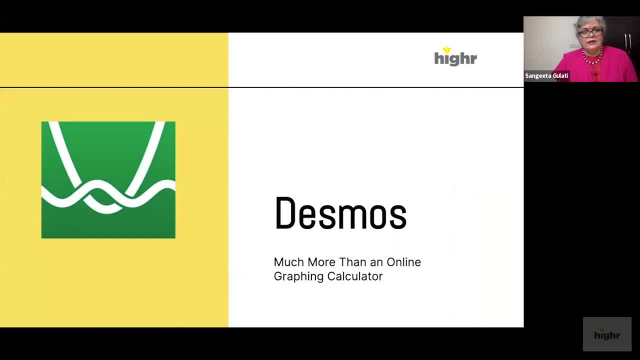 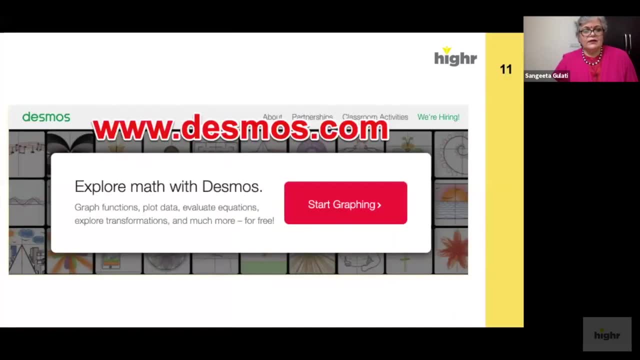 So Desmos was known and is understood to be an online graphing calculator, but it is much more than an online graphing calculator, So you'll find it at Desmoscom. So if you click on that big red button, then you can just simply start graphing. 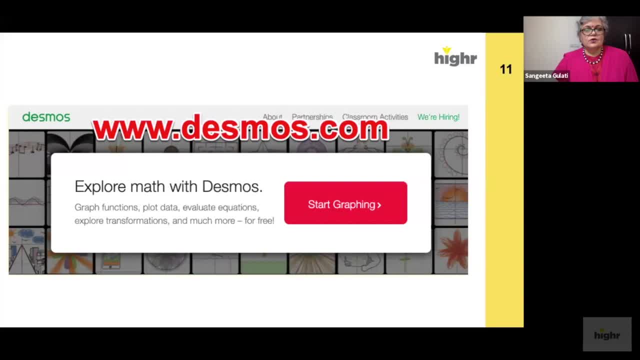 But it is much more than a calculator. So there are two wonderful things that one can look at when you look at Desmos. One is, of course, the graphing capability, And that graphing capability for me took the shape of for last several years. 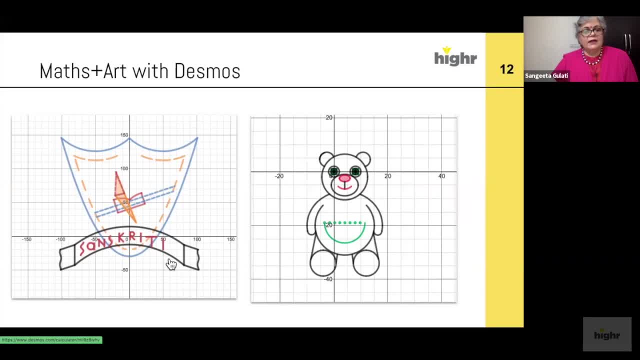 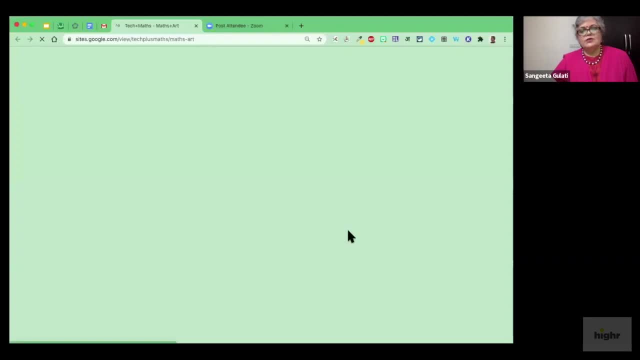 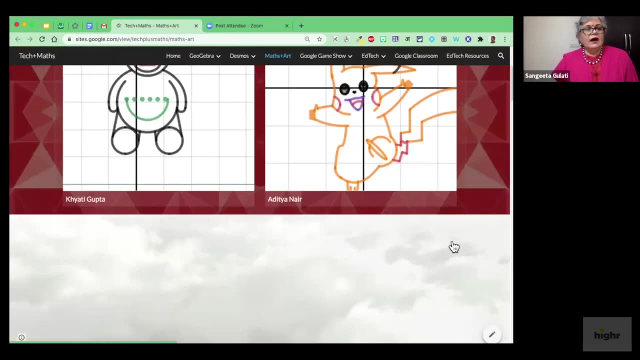 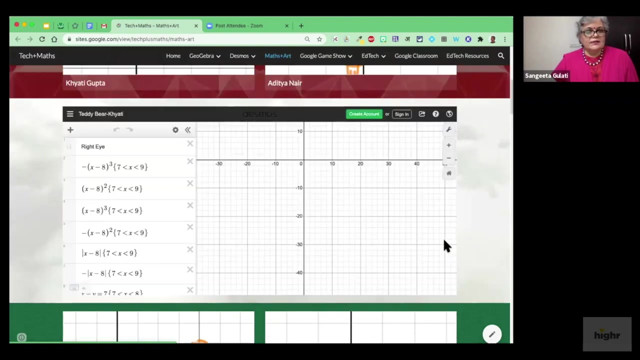 where my students turned that mathematical functions into beautiful graphs and artwork, which actually is nothing but complex. It is a composition of several functions put together. So, as you're looking at this, this is nothing but functions which are drawn and then also limited depending on the values of X and Y. 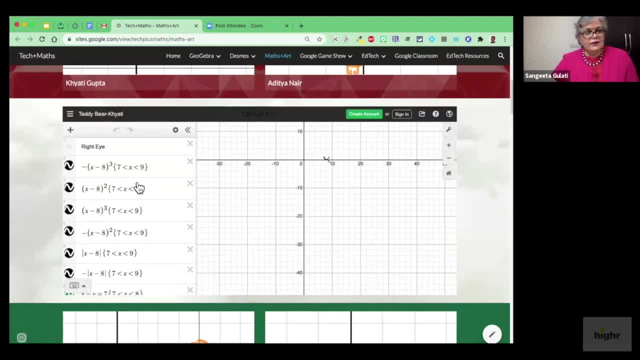 So just by restricting the domain and the range, as we call, of the function the students were able to create. each of these piece, as I'm putting my cursor on, is actually part of a graph. It would be a circle, It would be a line or it would be any other function that has been used by the children. 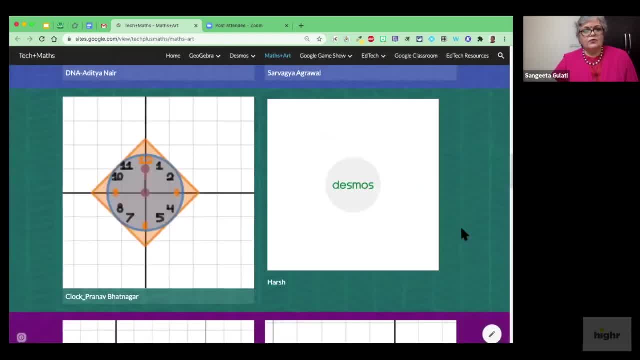 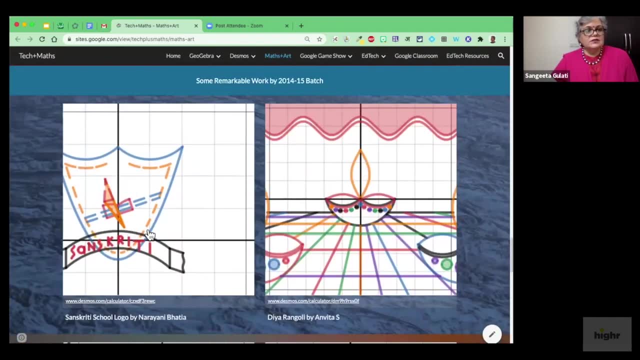 So, definitely, this is something which is very, very powerful, And this is what we are looking at when we want students to get engaged. So this, of course, is my school logo, which a student had made several years back, And I'm very, very proud of her and her work. 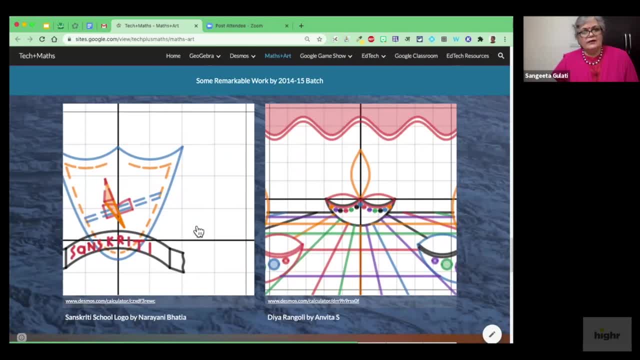 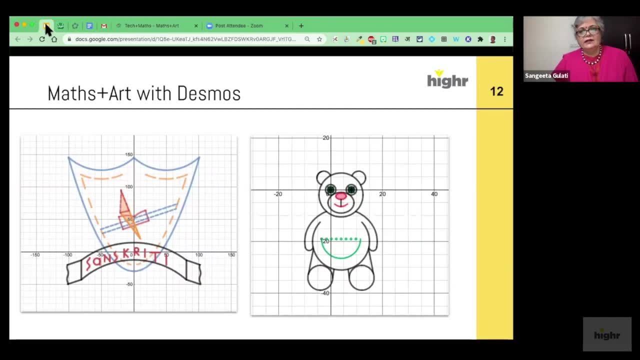 But the math that went behind this is amazing, The kind of understanding that just children have. that a child reflected because these functions at the grade 11 level were not even discussed or taught. At the same time, the children learn and grow with it. 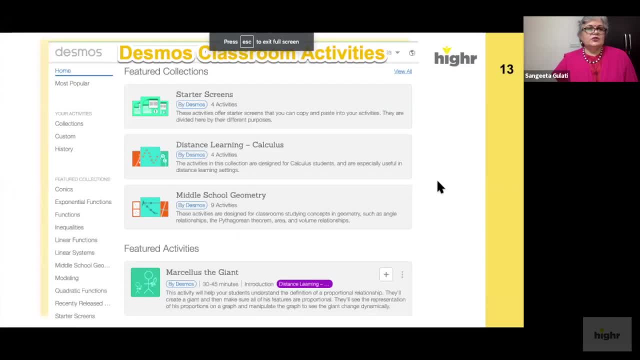 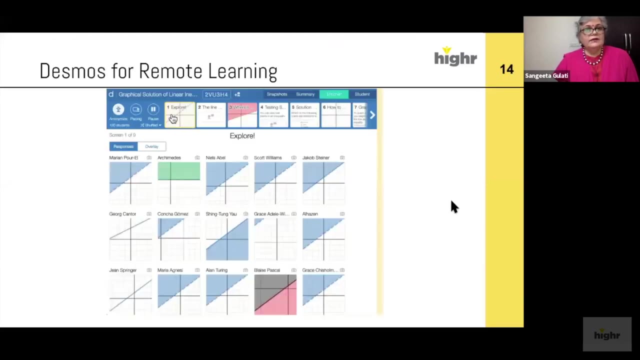 So when they reflect on what they have done, that shows their understanding. The second aspect of Desmos is Desmos classroom activities. So if you go to teacherdesmoscom, you would be able to find this And again. Desmos classroom activities are made of nothing but screens. 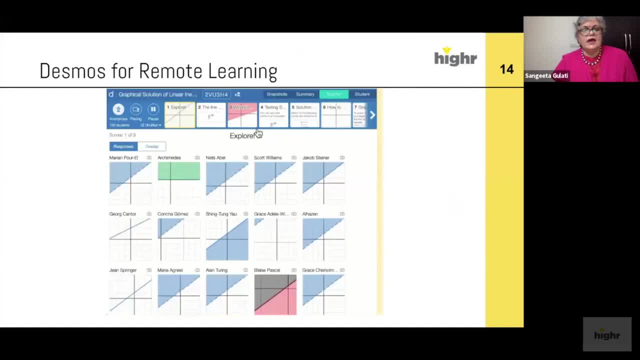 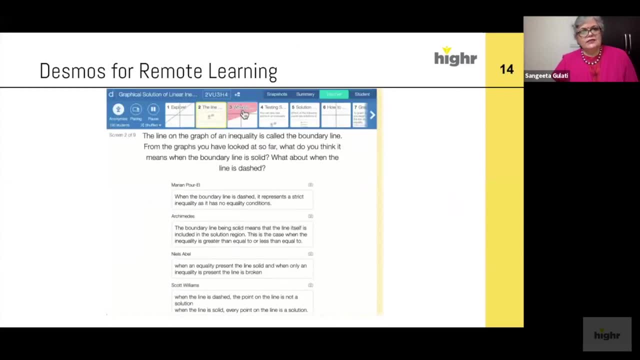 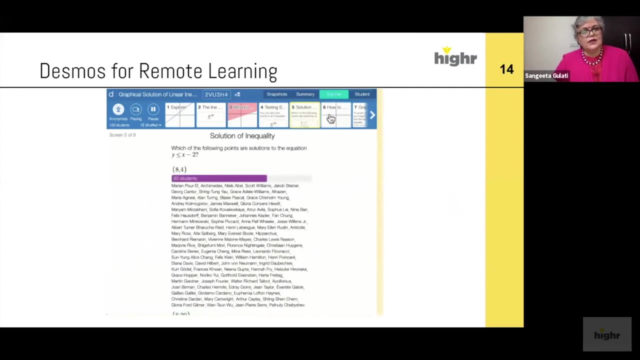 which bring in certain challenges for the students, And teachers can follow the work, So it can be a teacher-based or a student-based activity, And each of these tasks gives students a chance to think, to explore and also to visualize and also to create. 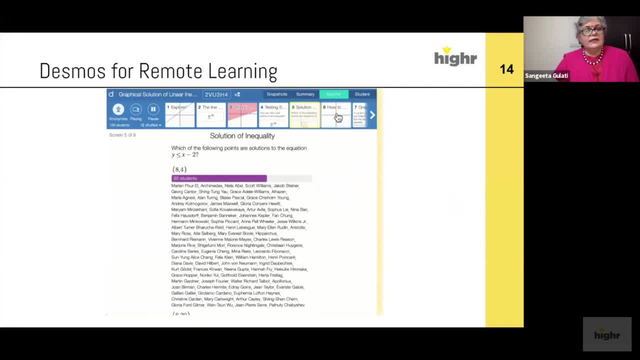 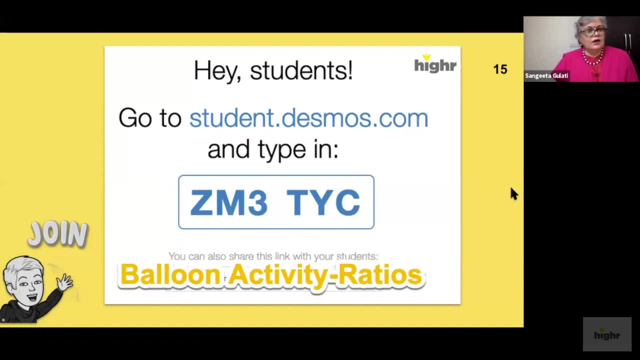 So all of that gets put together And these activities you can find on the teacherdesmoscom. At the same time, this is one of the activities which I'm opening to you to join in so that you can experience the joy of using Desmos. 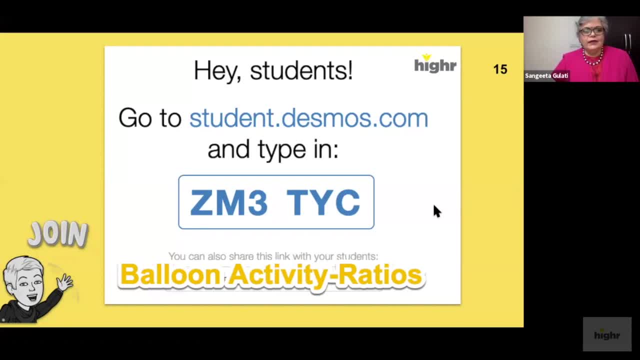 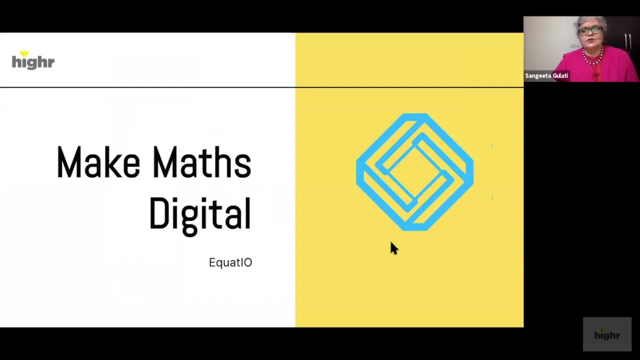 in a very, very different way. So, quickly, note down the code. So you will go to studentdesmoscom and this is the code which you can use And I will be able to follow the track as you work with it. So that is something definitely which you would be happy to explore. 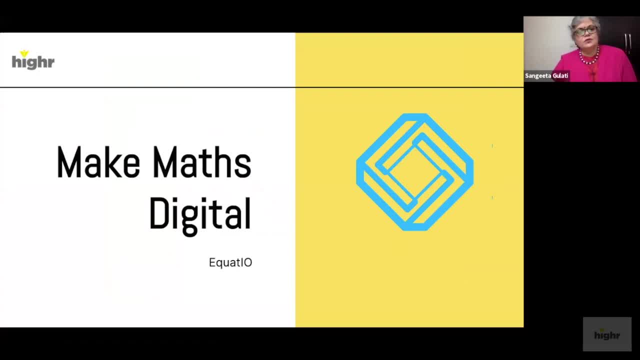 and then think about using And those activities. you can take them from the website directly or you, as a teacher, can also create them. The second thing which we all are looking at, other than, of course, creating these engagement movements for our students. 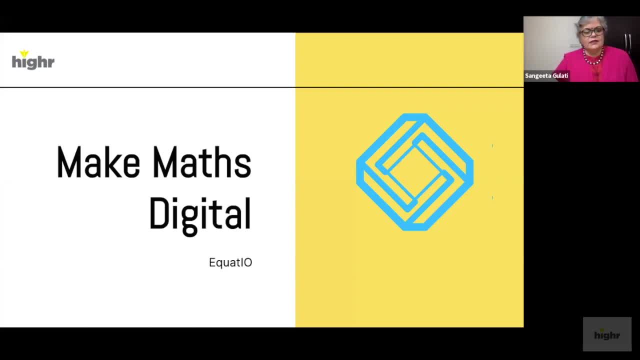 is also the struggle that maths teachers are facing: in writing maths, in typing maths. So there is a beautiful product. Just to clarify again: it is not a Google product. It's a product of a company known as Texthelp, And Texthelp is a company which creates a number of products. 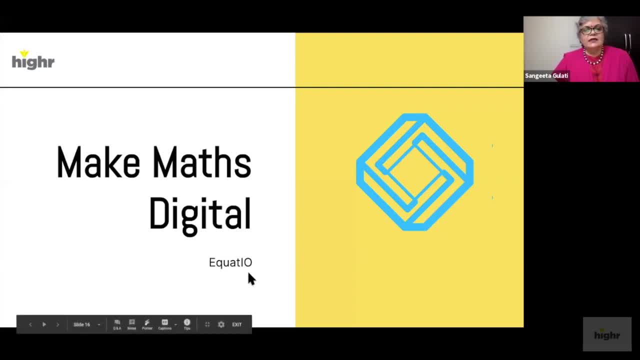 and EquatIO is their product for maths. It's a Chrome extension. It also has a number of other versions of it, So it works very well with Google apps, definitely, And what it does is it lets you make maths digital. 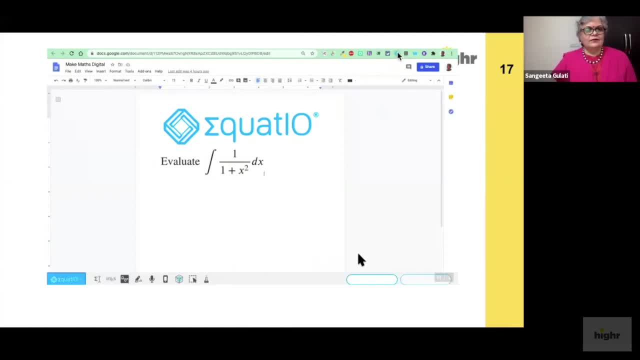 So this is just a short demo in the sense of: again, due to time restriction, we can't go into the live, but once you have added Chrome extension of EquatIO, then it's just a moment of you know, just open the extension. 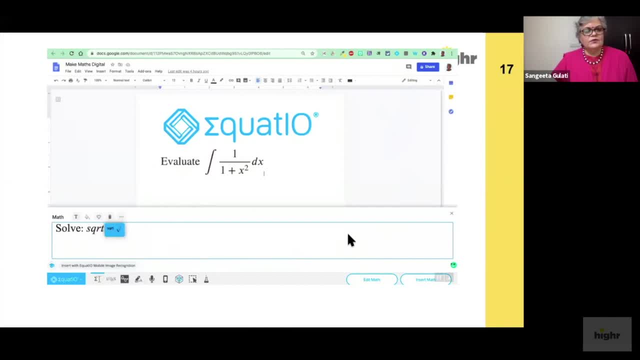 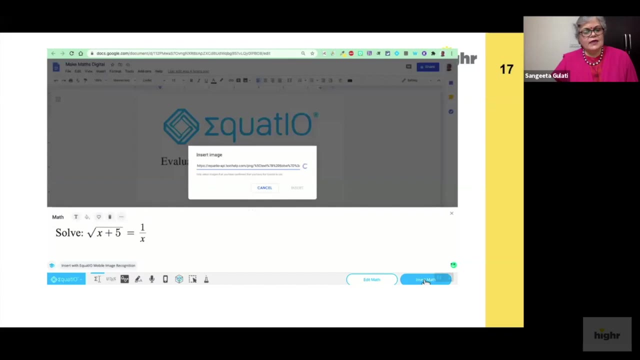 A small toolbar opens at the bottom of the screen and you can type in actual words. So to get the square root, I just have to write SQR and it will prompt as to what it is, What symbol I want, And it can be then added into the documents as an image. 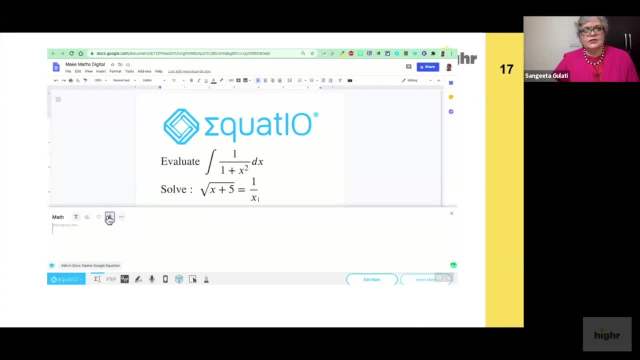 For Google Forms, because somebody had asked this in the questions Q&A. So for Google Forms it's a premium feature of EquatIO. But if your school is a registered school with the G Suite for Education, then or any other ID that is registered. 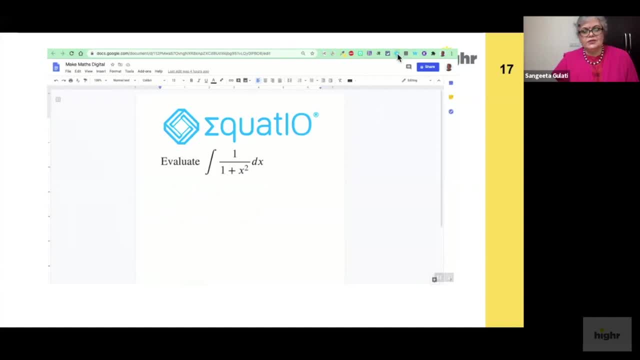 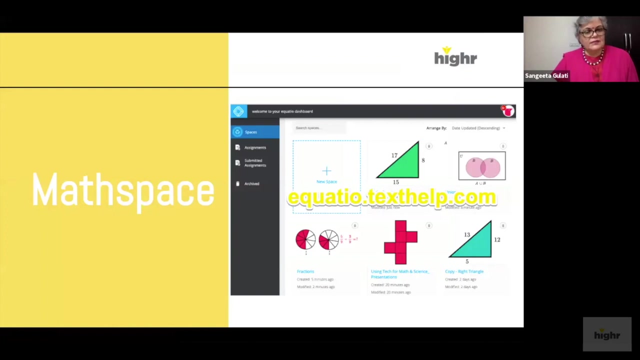 then that would allow you to get this premium feature. So definitely, EquatIO is the product to go forward. Along with making these typing easy for us, what EquatIO also has is something called as MathSpace, And MathSpace is again an opportunity for us. 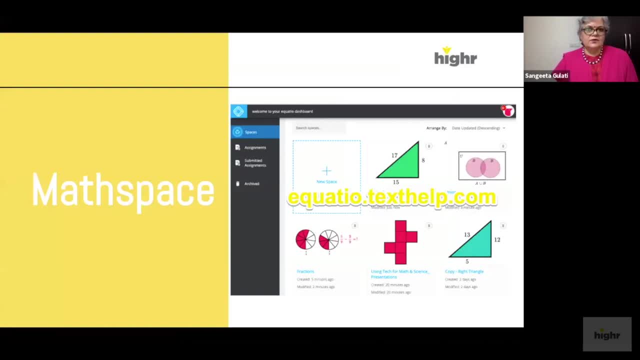 to create interactive tasks for the students, And it is also integrated with Google Classroom, So any task that is created here can be assigned to the students. And in fact I did not mention GeoGebra- is also very well integrated with Google Classroom. 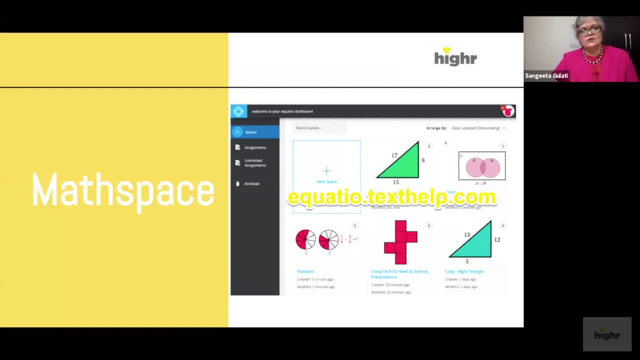 So you can assign these tasks through Google Classroom so that students work can be assessed, and you can also guide students, give them the feedback and take the learning forward. So definitely these are the tools that we can explore and see how your teaching and learning. 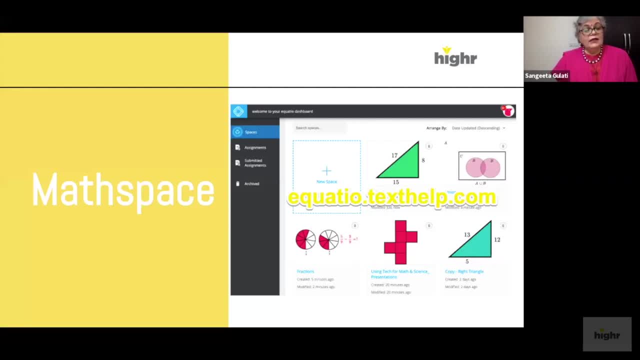 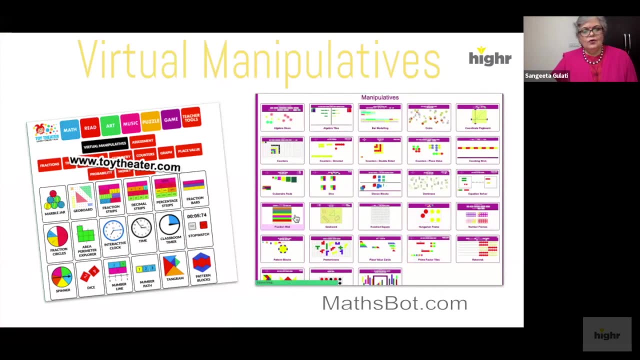 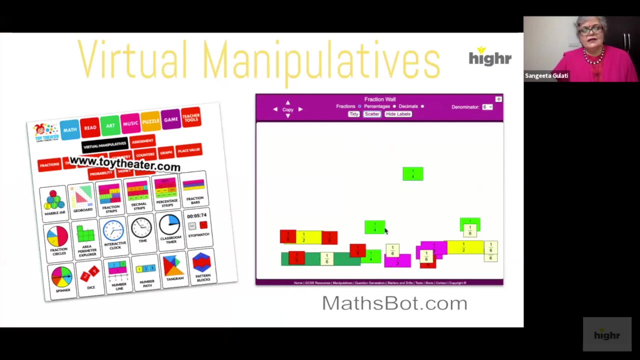 in Math's classroom changes. But if you are one of those teachers who is missing those manipulatives that you have all over the room when you are teaching- and especially the younger ones- then there are two websites that I would like to recommend. 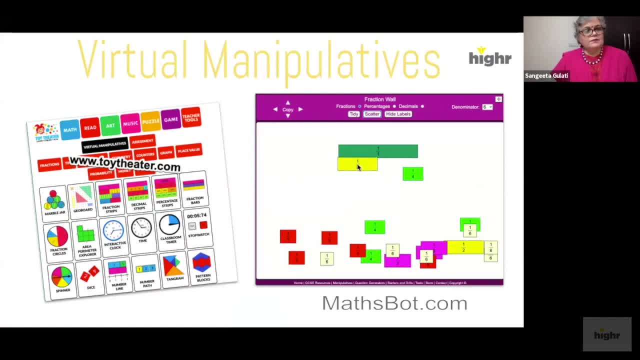 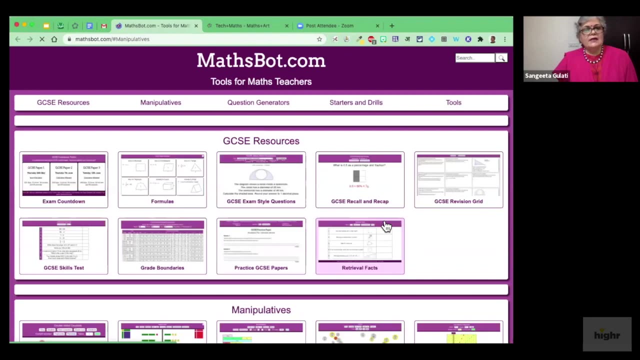 There are a number of websites around us, but two websites which I definitely would like to recommend. One is toytheatrecom, So definitely go and check that out, And the other is mathsbotcom, So mathsbotcom has more than manipulatives. 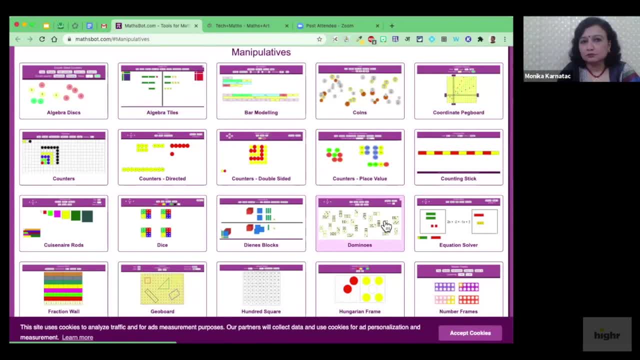 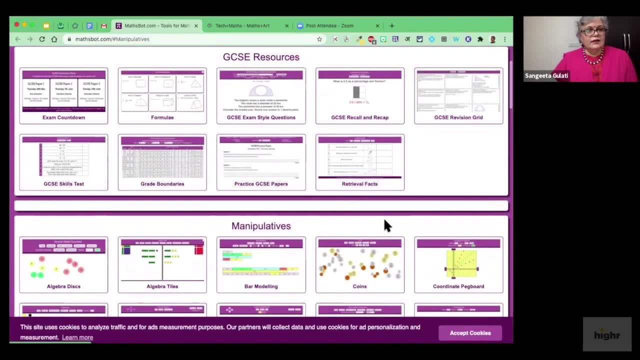 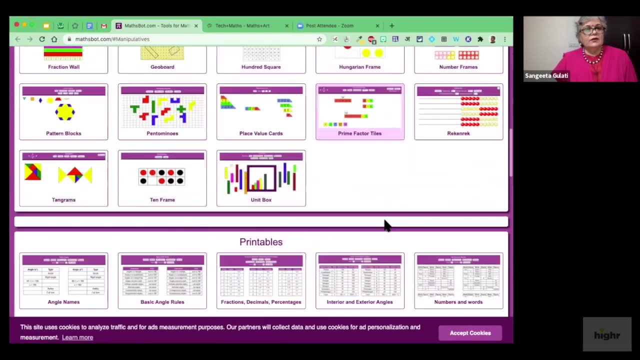 It has such a wealth of resources, which each one of you will be able to find useful, So you can use them in your online classes. as we are looking at, you know, the next few months, perhaps for us And you can make these demonstrations come to life. 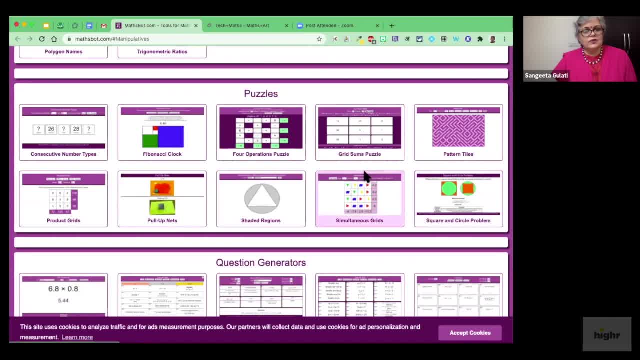 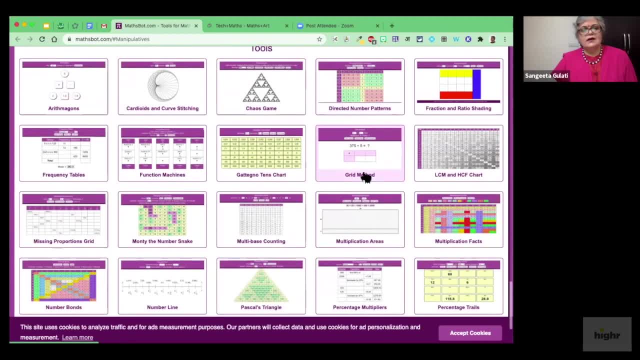 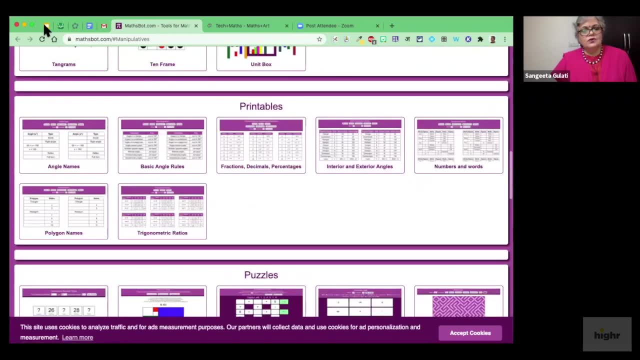 Also give certain puzzles to the students to do, so you can share the links from here. There are lots of brilliant ideas for each and every maths teacher to take something from here and make use of, So definitely this is something which I guess you would be able to. 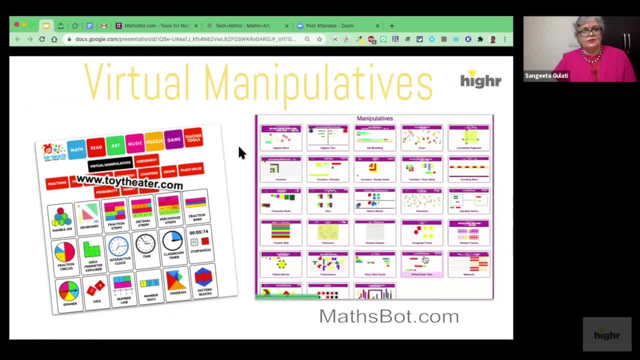 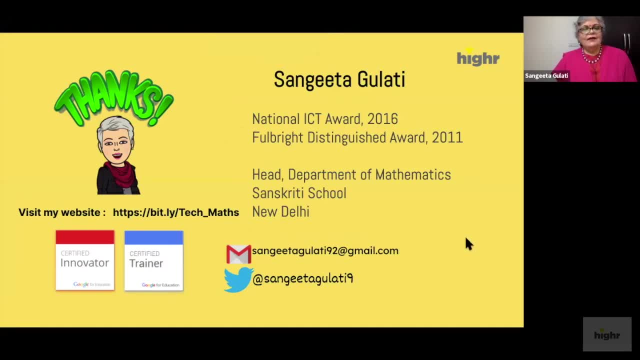 make use of and take forward from here. So I am not too sure of how much time I have taken. So I'm going to stop here And let you explore these And I hope if you have joined both the GeoGebra classroom and if you have noted the code for Desmos. 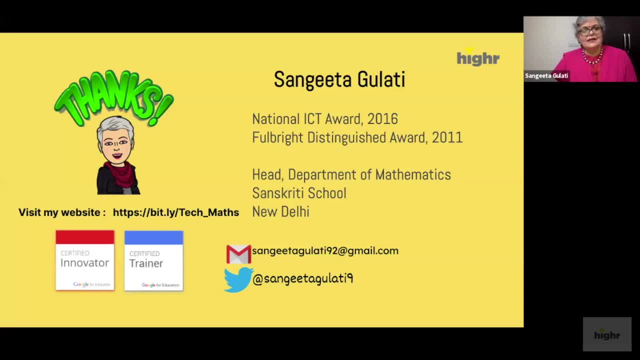 and have started with it. I'm going to just open that out and see if you have made any progress or not. And yes, do visit my website. My website name actually is techplusmaths, So this is the short link for that. 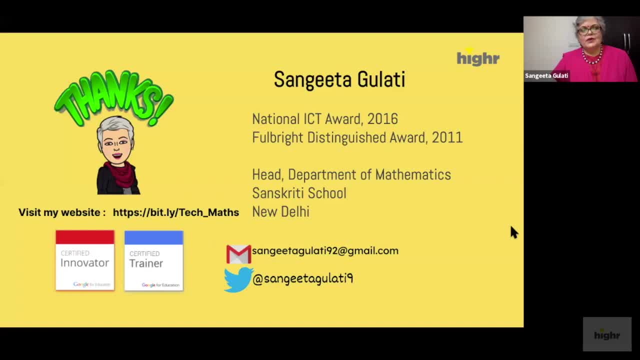 And you will find more on GeoGebra, Desmos and more edtech tools on my website. So thank you, Pallavi, Over back to you. Thank you so much for that, Sangeeta, I think, given the number of questions, 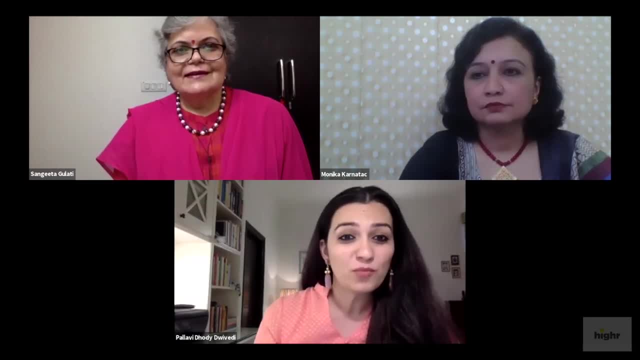 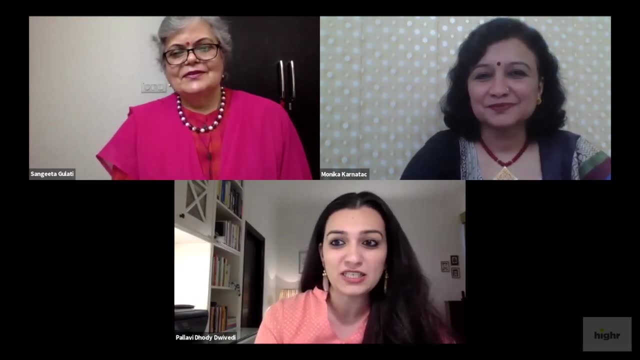 that are coming in. you're going to see a lot of people trying out both GeoGebra and Desmos. I know that I will certainly be trying it out and looking at what are the different options and opportunities. There are some absolutely fantastic activities. 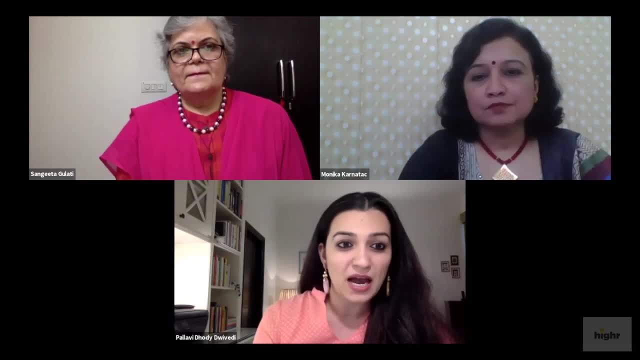 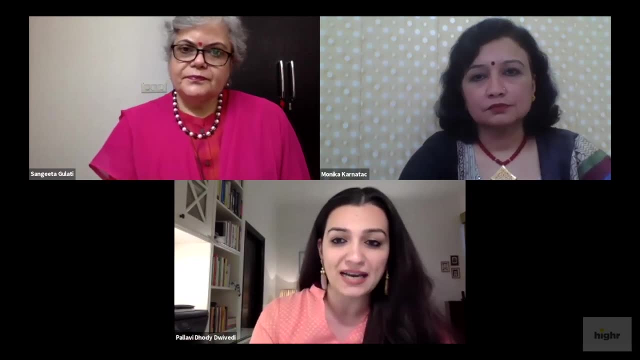 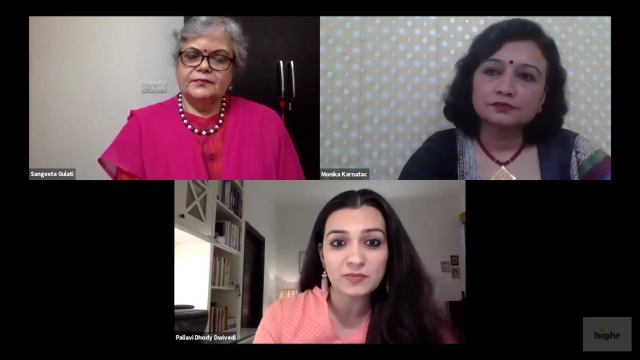 that you can try with GeoGebra and Desmos, both of which Sangeeta was mentioning. there is a pretty large repository of different activities, both for online, of course, for online as well as for blended learning, that you can try using GeoGebra and Desmos. 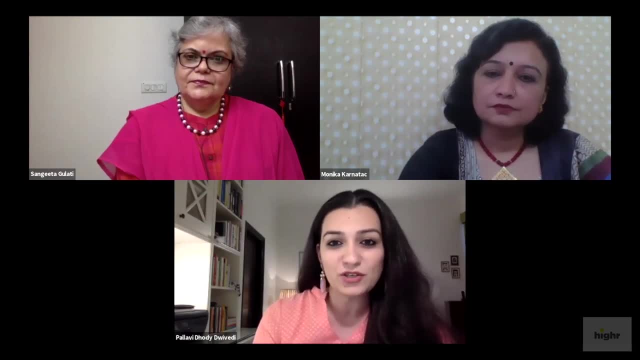 on their websites as well. So for those of you who are looking for some interesting activities to try out and get started, if you're unfamiliar with the tool, these activities will also help you get a head start in using the tool and trying them on. 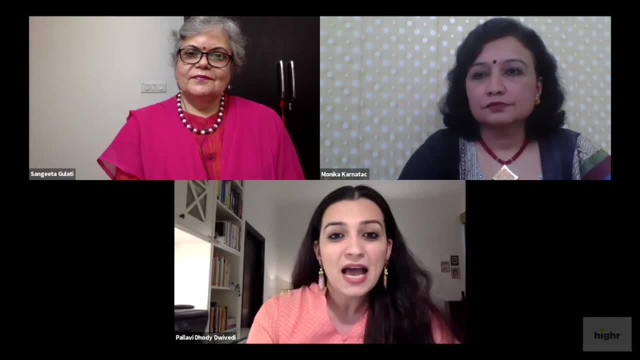 So here's hoping that you'll go out there and explore some of these. There was a question, Sangeeta from Parvez, who wanted to know if you did have a few examples of the kinds of activities that you've built in to the use of these tools. 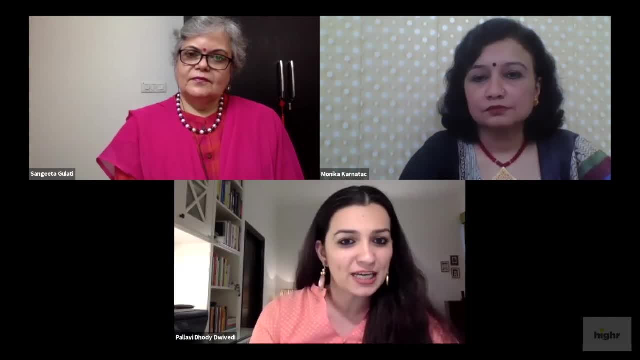 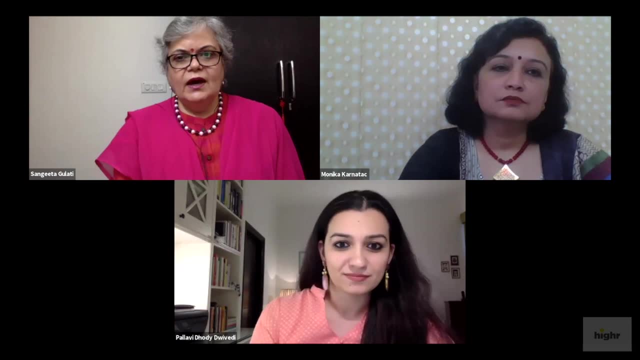 to try and increase student interaction and engagement, If you could talk a little bit about that. Yeah, sure, There are. again, as you said, both the websites, both GeoGebra and Desmos. they have ready-to-use activities. 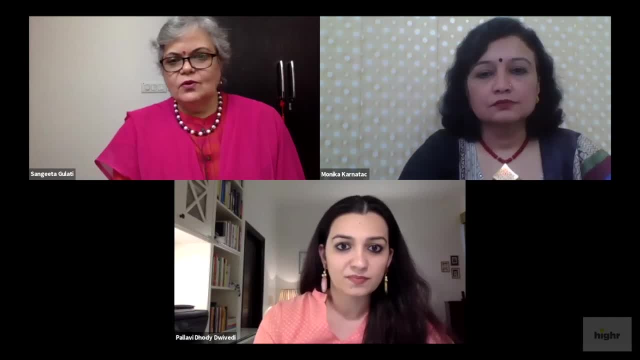 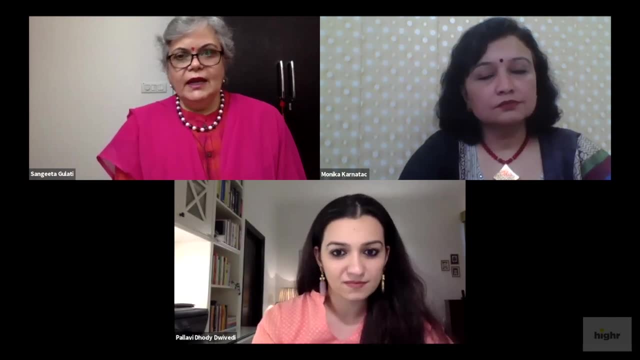 which you can go and explore on your own. You can customize as well. So both Desmos activities as well. some of them- not all, but some of them- you can edit and you can add more screens to it, add more challenges or simplify. 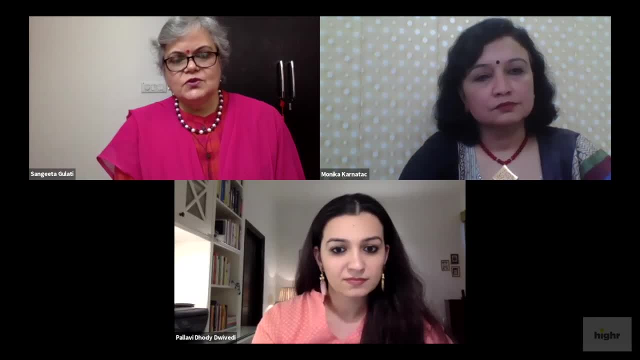 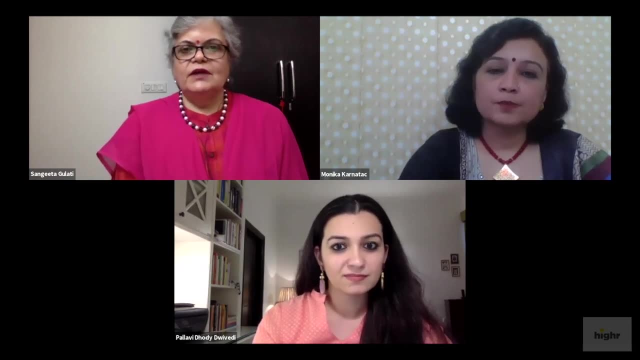 You know both ways it goes. Same goes for GeoGebra, So you will definitely have them there, And if you want to see more examples which are in sync with what we are teaching in our school, then my website also has some of those applets. 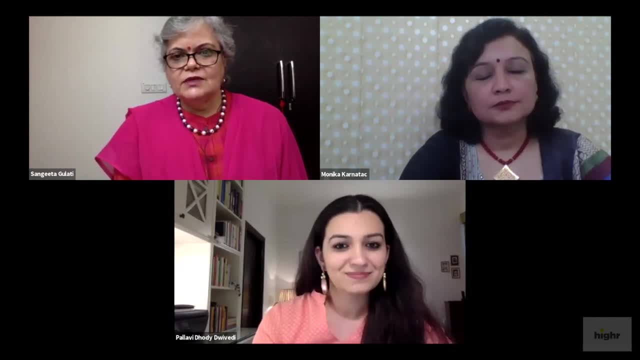 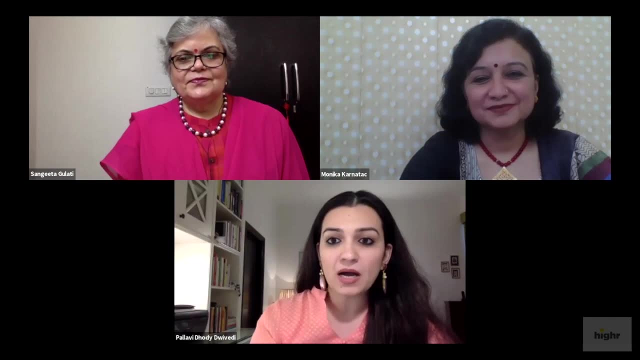 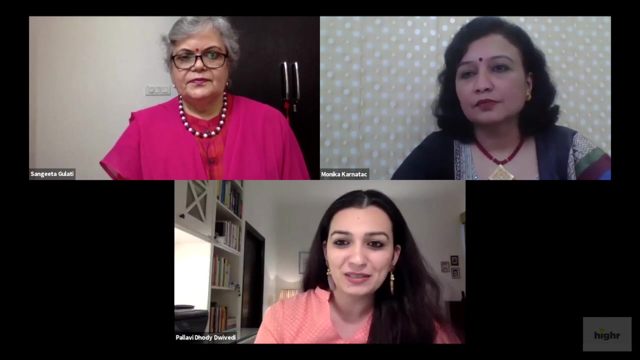 which you can check out from there. So there's no doubt of resources around us. Absolutely Fantastic. Thank you so much, Monica. would you like to add any other activities that you have used in particular, which others can look at for inspiration? 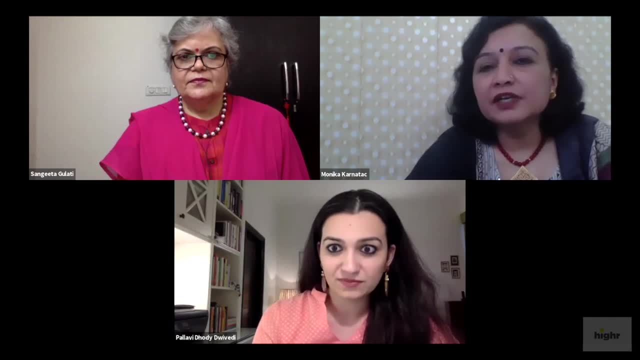 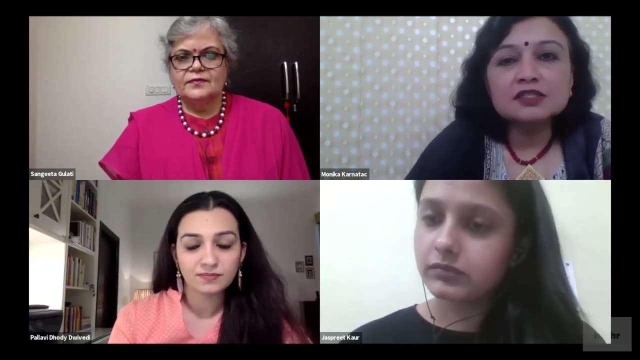 I have used GeoGebra to create different types of parabolas. Just show it to the students in the class. Just by one click I can change the equation and just see the effect of the equation change and the shape of the parabola. 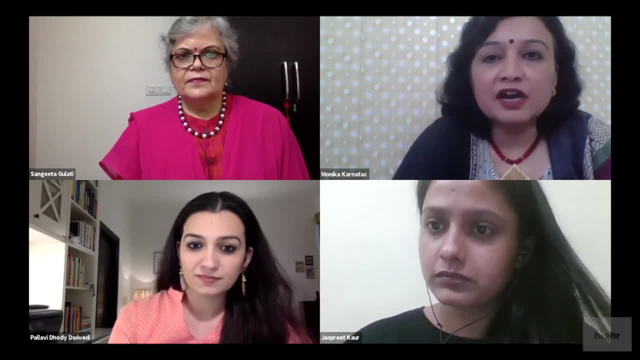 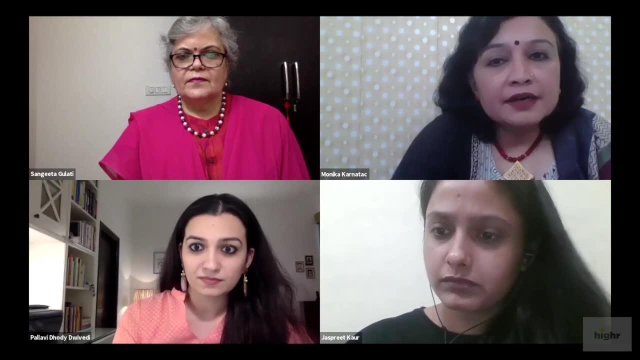 So it is very helpful. Students can see that, what graphical effect we are getting when we are changing the equation with parabolas, ellipse sign graph with modulus function, everything. I used to attend Sangeeta ma'am's workshop and every time I post a video in my YouTube channel. 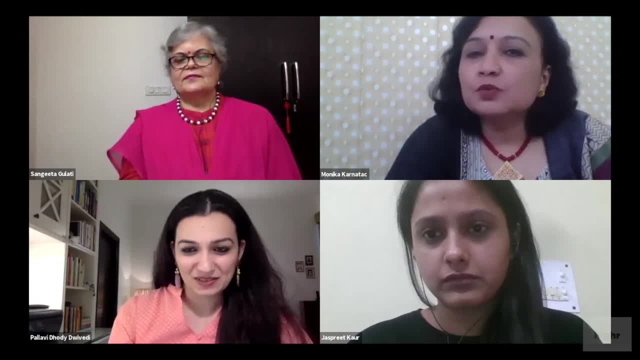 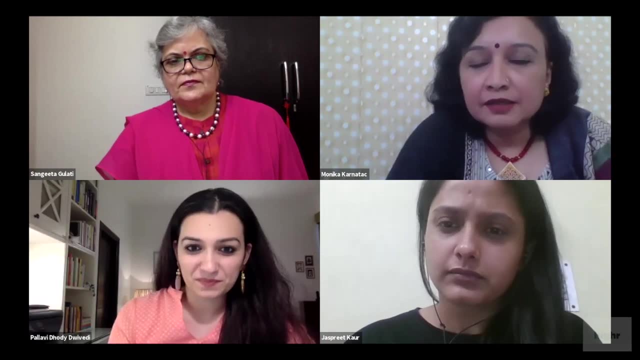 So it's very useful. GeoGebra: I have worked on GeoGebra and it's very useful And showing it to students it just gives the thing that they start thinking That if we are moving, if we are changing the equation like this, 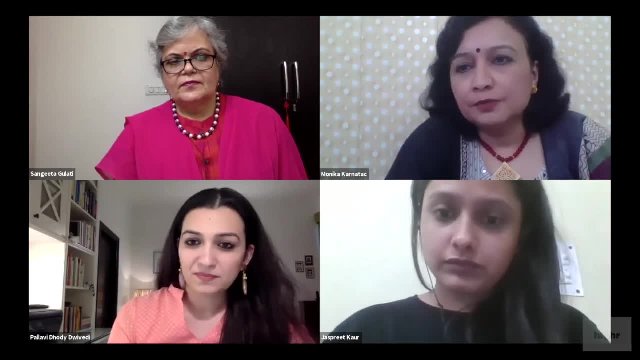 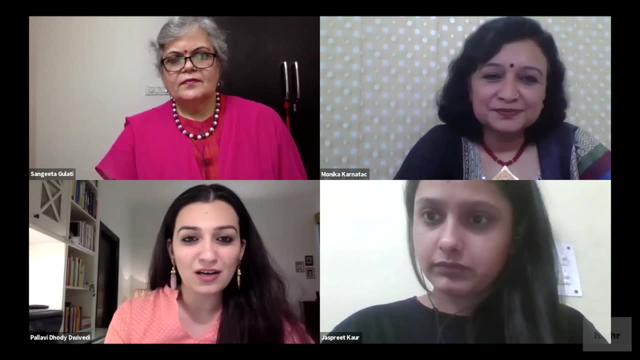 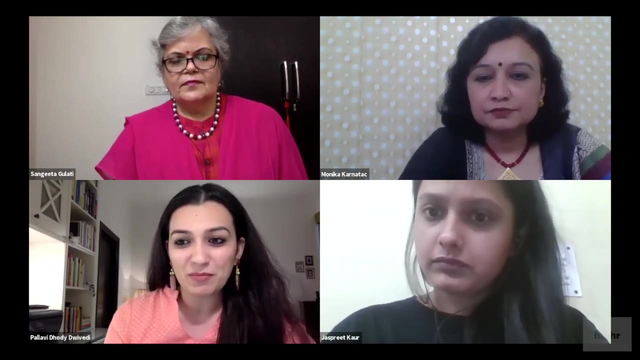 what is the effect on the graph. So it's very useful. Fantastic, All right, Thank you so much for that, Monica. I'd now like to move on to the science part of today's presentation, And I know that there have already been a couple of questions. 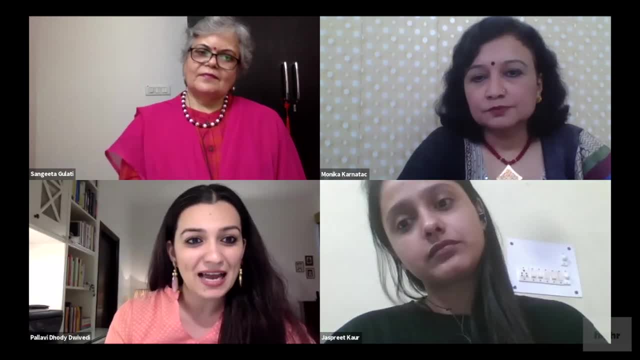 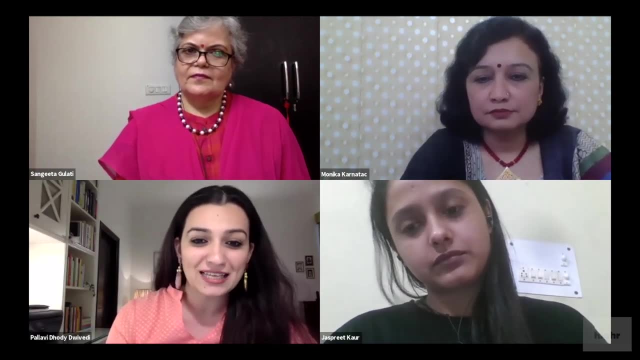 that have started coming in for science. So I'd now like to hand over to Juliana to take us over some of the interesting things that she's been doing in her classes. She's been doing in her class for science. Thank you so much. 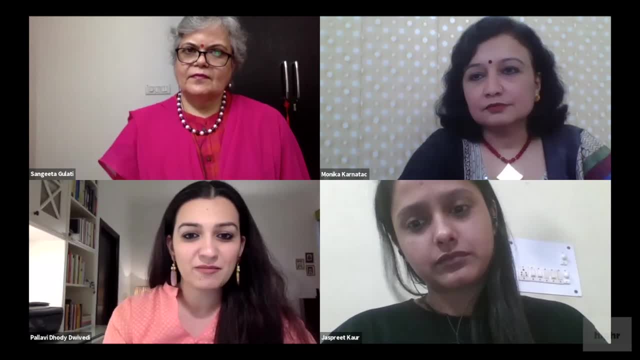 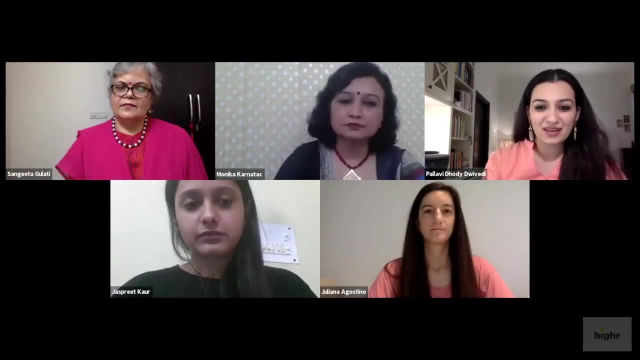 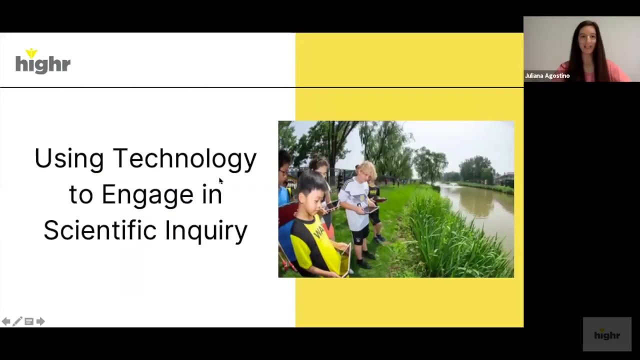 Is it possible to turn on my video? Yes, just give me a quick moment, Thank you. There you go. Thank you so much. Okay, Hi everyone. My name is Juliana and I've been teaching mostly IV science and biology courses for the past 12 years. 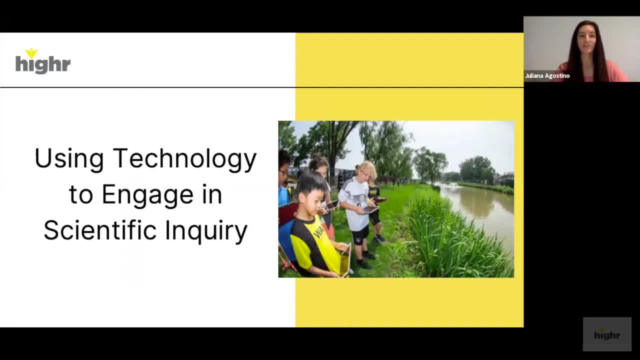 And, as mentioned, I currently work at the Western Academy of Beijing, which actually closed very early in the pandemic. So we've spent the last 19 weeks almost entirely online with many of our student and faculty population all over the globe. So I'm here today to talk to you about 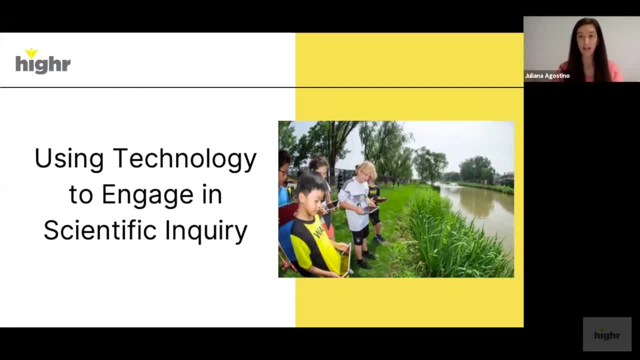 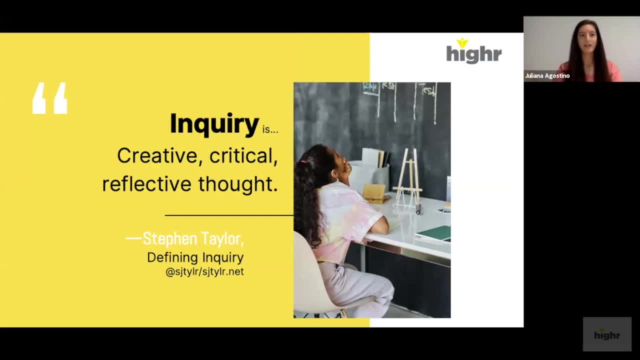 how you can still engage your students in scientific inquiry, even while we're online. So when we talk about scientific inquiry, we often think of students engaged in some kind of investigation. Right, It's an active process. They're thinking critically, They're thinking creatively. 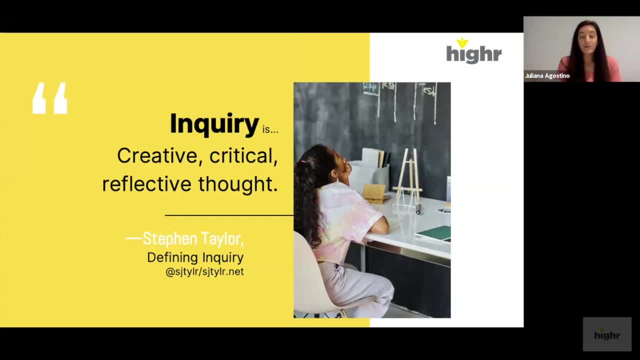 all about the world around them. In the classroom we might get students to get excited by having them explore through a hands-on experiment or a demonstration, But in our current climate we might not be able to physically be with our students or have them in a traditional science lab. 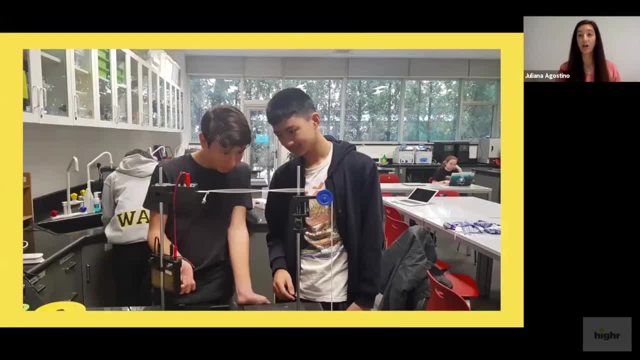 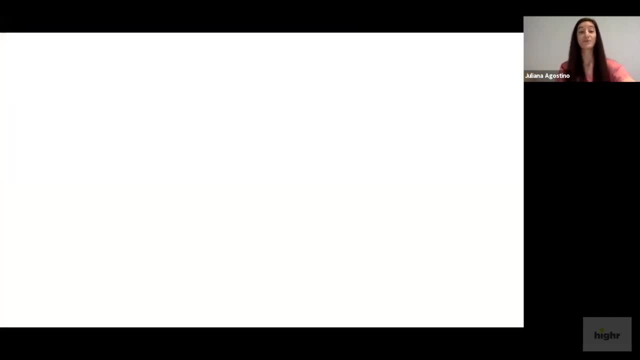 But we still have the power to ignite their curiosity and their interest in how the world works, And we can do that by leveraging the power of technology. So the online environment provides students with simulations, virtual labs, games, apps and more. That being said, 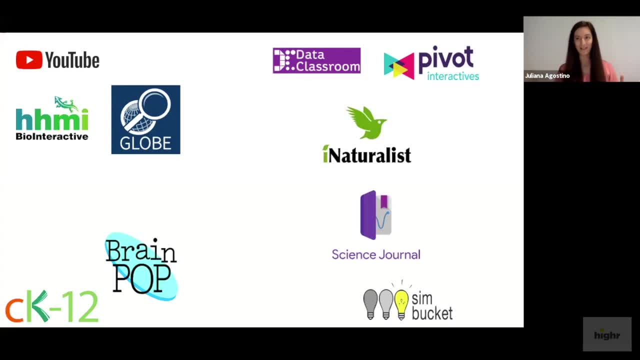 10 minutes is not really a lot of time to go through all of these things and it would be very overwhelming, So I'm going to focus the rest of my talk on a few key examples. The rest you can actually find in a Google Doc. 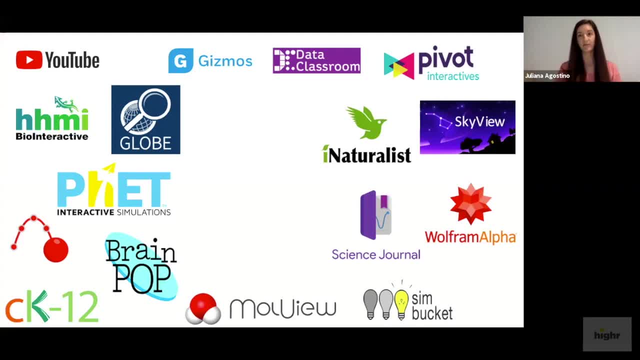 in a link at the end of this presentation that will be available for you. So what we have to keep in mind, however, as we go through this presentation, is that it's really not about the technology, It's about the pedagogy. 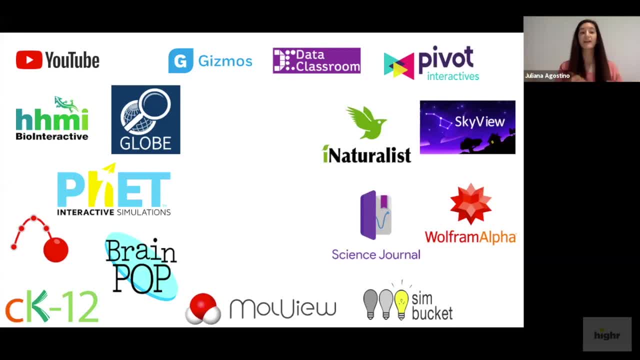 And we're trying to figure out what tool is out there that can support what it is that we want to do. So even though we've had to make a shift to learning in the online environment, that doesn't mean we can't still connect our students. 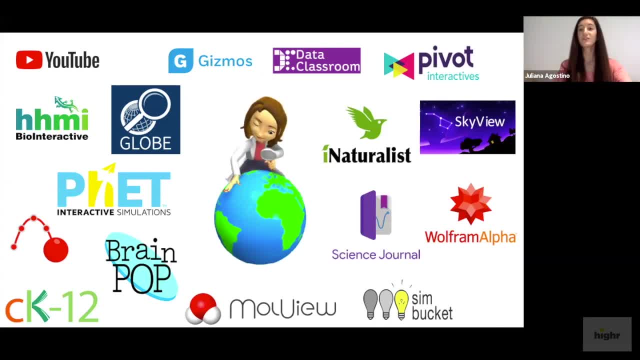 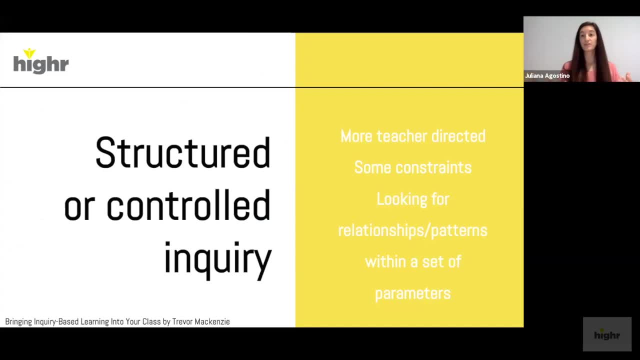 to real-world scientific inquiry. So let's look at a couple of scenarios. So in scenario number one, let's say you want your students to do some kind of structured or controlled inquiry where it's a little bit more directed by you in that you have a certain goal. 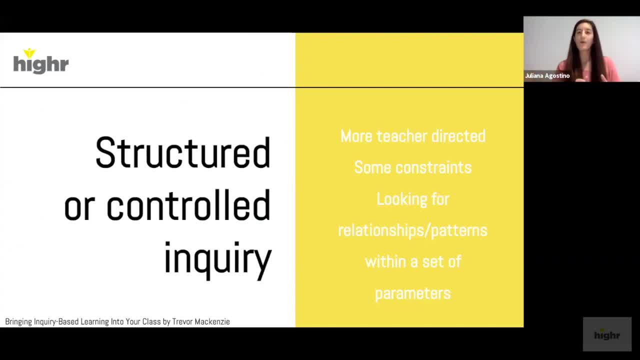 of what you'd like your students to learn about. You want them to be able to play with virtual lab equipment or make some observations, look for some relationships or patterns, but within a given set of parameters, Like, for example, you're doing a photosynthesis exploration. 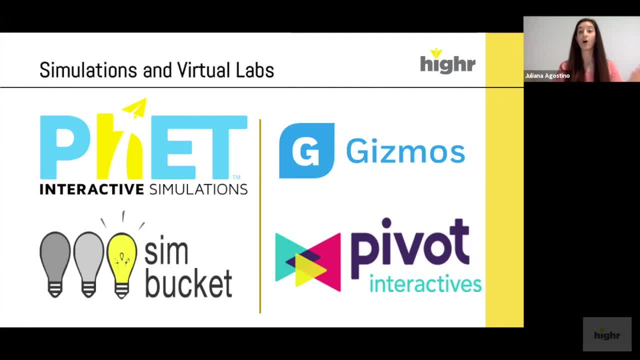 So in this type of scenario, I highly recommend online simulations and virtual labs, And I've put a few key examples that I use on this slide, but specifically in this presentation, I'm going to talk about my favourite one, which is PhET. 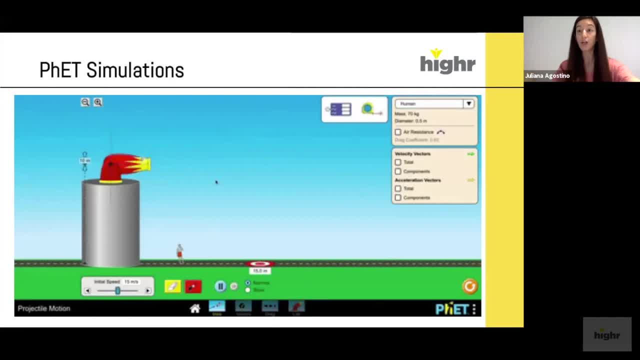 So PhET is an award-winning website full of free math and science simulations that cover a huge variety of topics. I use these simulations a lot when I'm teaching concepts like motion or chemistry, topics where it's impossible for students to otherwise visualize something that's happening. 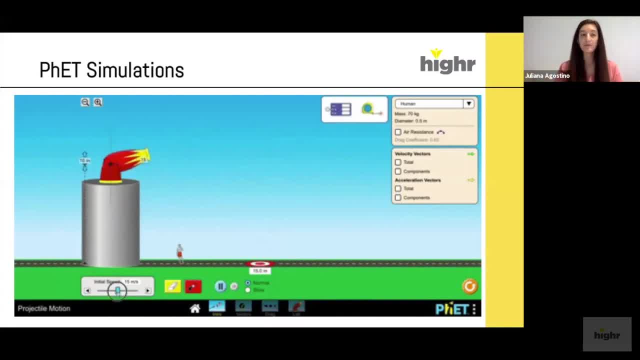 at the atomic or molecular level. So these simulations are amazing because they allow students to interact. They can click and drag and slide things and that changes the parameters in the simulation. They then get immediate feedback of the effect of the changes that they made. 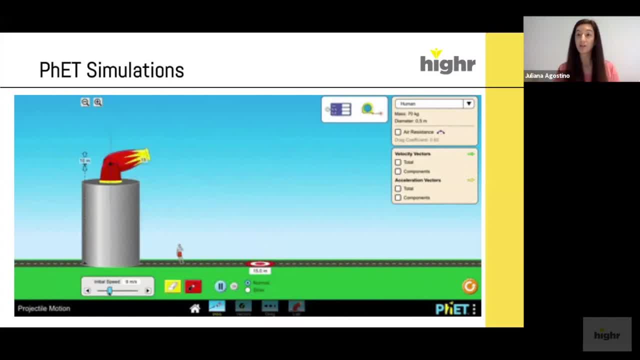 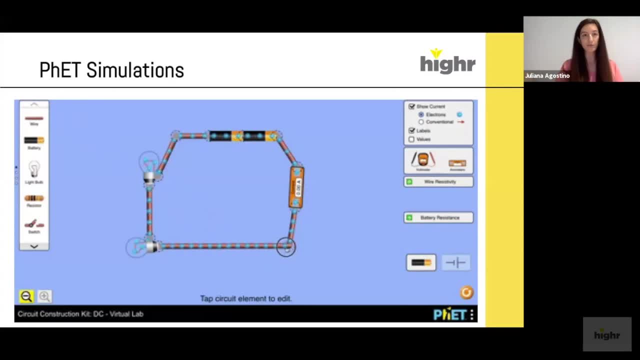 So it's really easy for them to see relationships between different variables. They can also take measurements using real equipment that you would use in an actual lab. You can even use some of these simulations with elementary school students, and you can very easily share the HTML5 simulations. 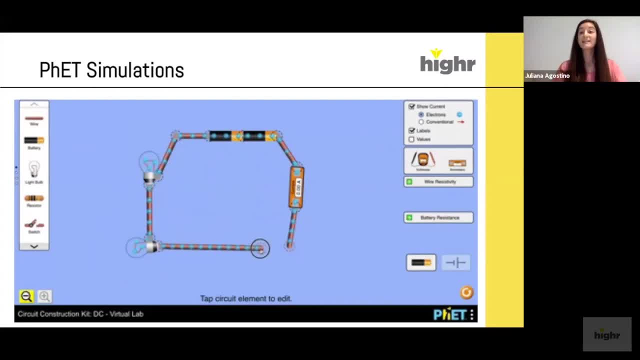 in Google Classroom. What makes these sims so great is that they don't actually have any instructions directly in the sim, so it allows for students to just go straight in and they can play, and they can come up with their own questions and make predictions and find their own answers. 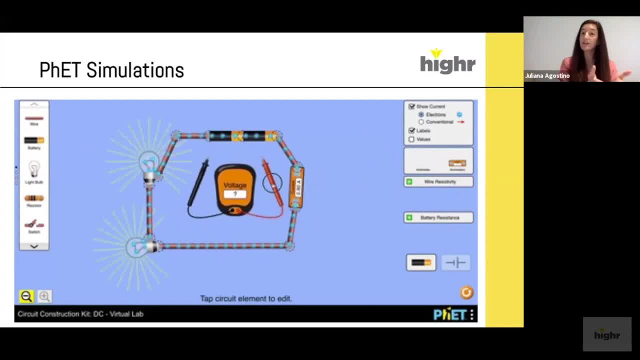 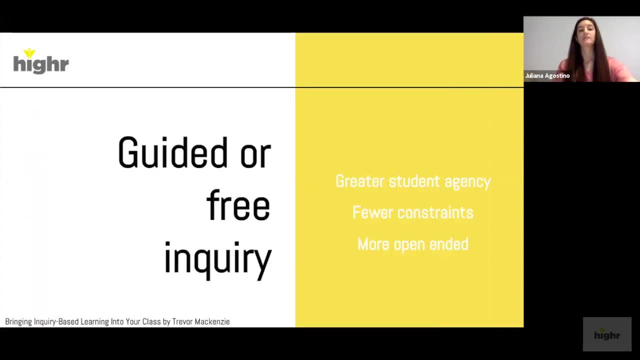 So it can allow for some very structured inquiry if you want to take the lead, or it can allow for some very open-ended investigations. Let's look at scenario number two. Let's say you want your students to do more guided or free inquiry. 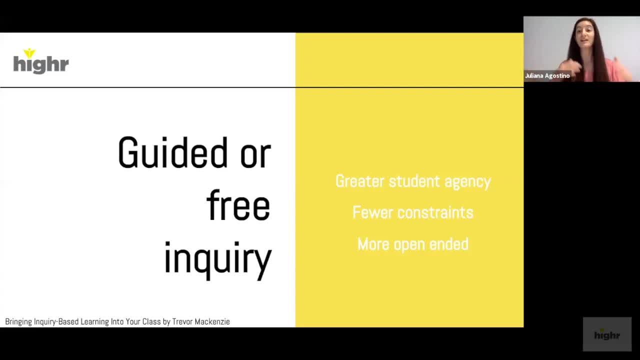 where they're the ones out collecting the data and they're doing entirely open-ended, student-driven investigation. In this part I'll highlight a couple of apps that I really like. So the first one is called iNetwork. It's an app that you can use. 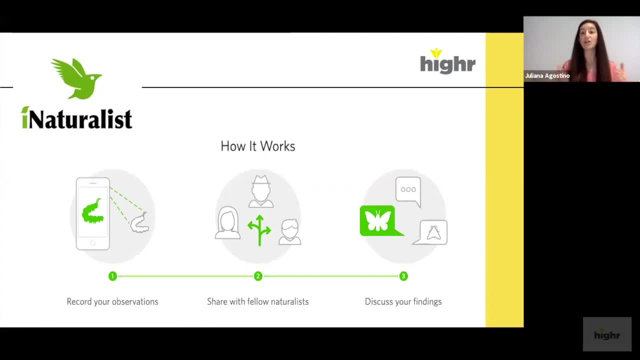 if you're a naturalist, and this is a wonderful app if you are doing a science unit that has an ecology or environmental science focus. It's a very popular app that allows you to identify plants and animals all around you, and it also connects you with a community. 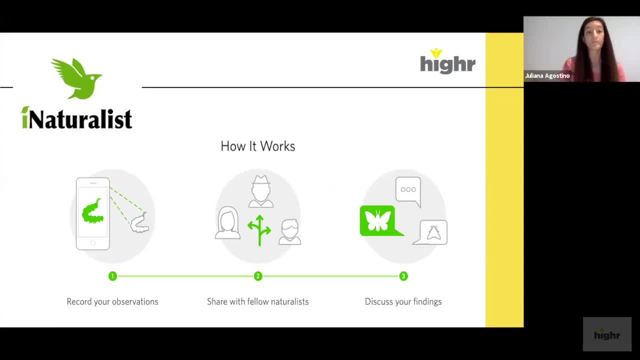 of over a million scientists and naturalists all over the world to help your students learn more. The really amazing thing about this tool is that by having students recording and sharing observations, they're not only learning more about the world around them, but they're actually contributing research quality data. 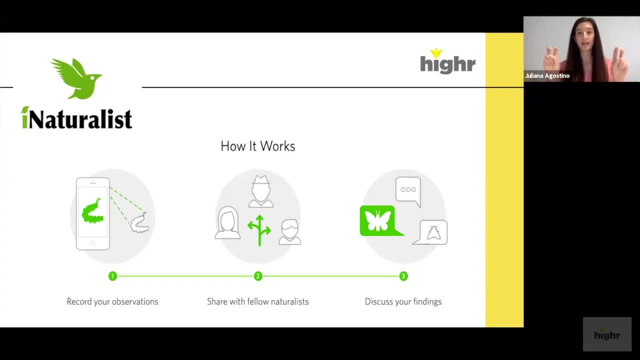 to the scientific community or engaging in what we call citizen science. So this brings a lot of authenticity to what you're doing in your classroom. right, There's more student buy-in because what they're doing really actually matters. So, as you can see on this slide, 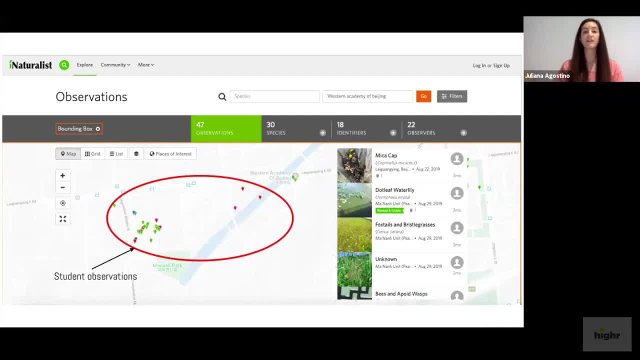 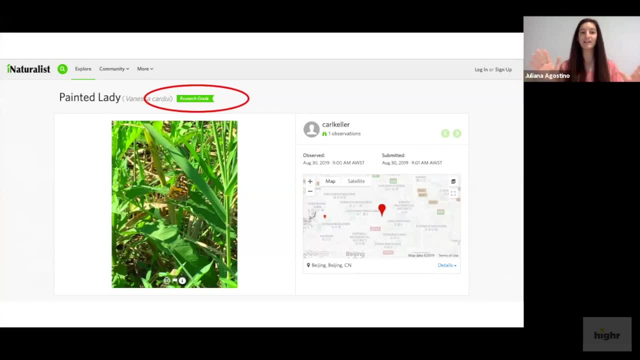 these pins on the map are observations and identifications made by a few of my students this year. Some of them were even verified by experts in the app. so they get a little badge that says research grade and that makes the students really excited. 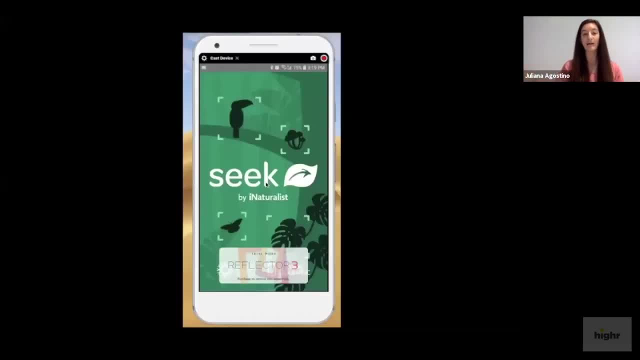 So you can find this app in the Google Play Store or in the App Store, and it's free to make an account. The website is full of video tutorials on how to use it, and there's even a teacher's guide. What they recommend is that you download this app. 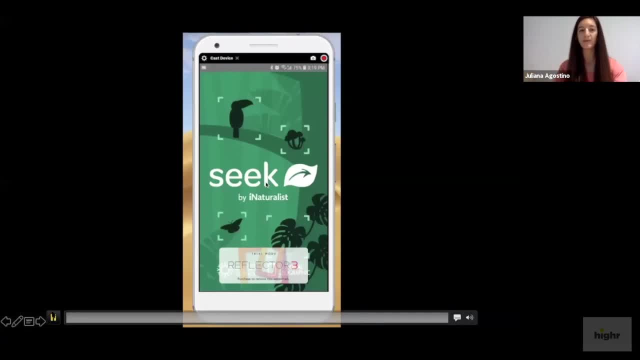 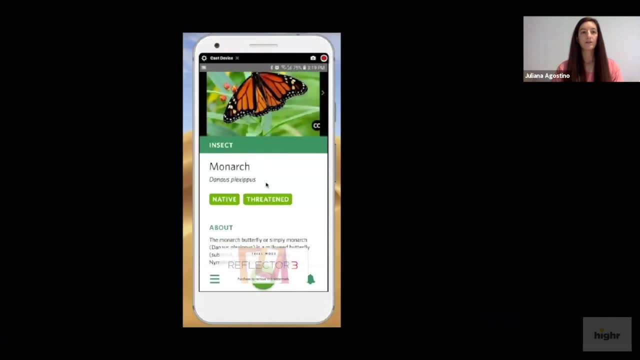 which is called. it's like a more junior version of the app. It's called Seek and it can even be used by primary students. It's so easy. Once you download the app, it automatically gives you some information about local species you should be able to find. 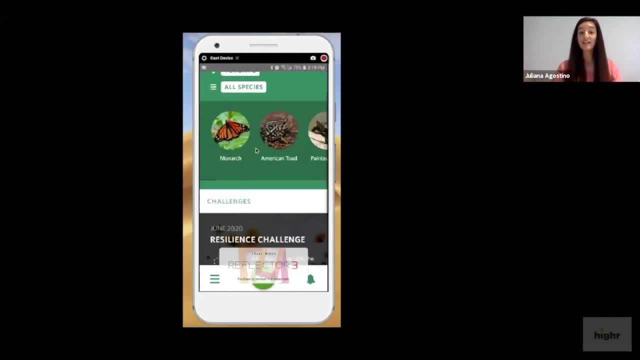 And the really fun thing is that you can earn badges and participate in challenges, So it makes it really, really fun when you're out identifying plants and animals. So, as a teacher, you could really scaffold how you use this app, depending on what level of inquiry you want. 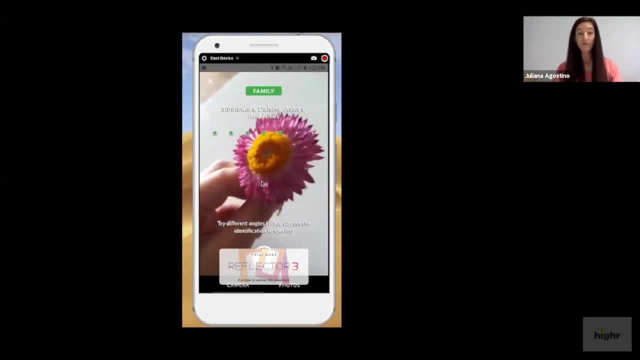 So maybe for younger students you could set up like a scavenger hunt for them to go out and find things. Or if you have older students and you're studying maybe the health of the local ecosystem, you could have them look for indicator species or invasive species. 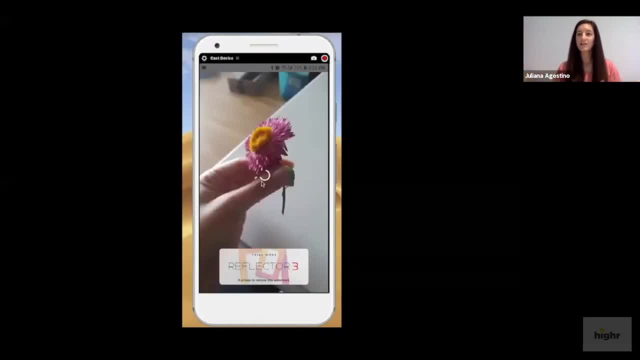 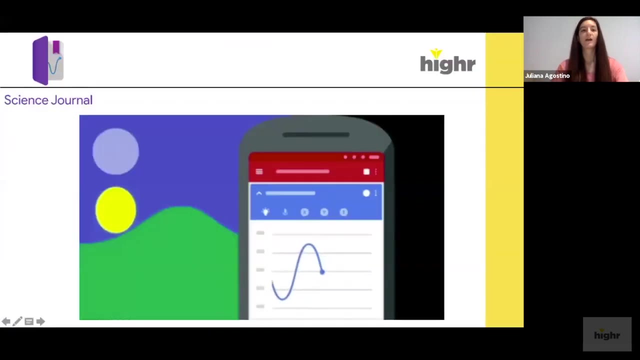 or set up some quadrats and transects and look for the relationship between species distribution and an abiotic factor. Whatever you want to do, it's a wonderful app for getting students out and engaged with their local environment and with nature. My other favorite app is Google Science Journal. 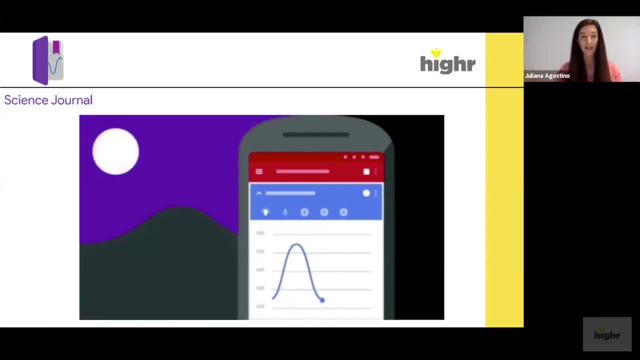 So this app basically turns your phone into a portable science lab, And it takes advantage of all the sensors that are already built into your smartphone. It's again completely free and compatible with multiple platforms And basically students can take their phones and collect data about things like sound intensity. 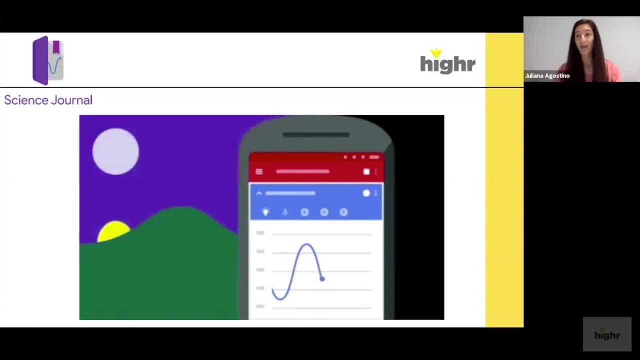 and pitch, light intensity, air pressure, magnetic fields and motion. And again, depending on what level of inquiry you're working with, you can either use one of the 70 or so pre-made experiments on their website or you can have the students designing. 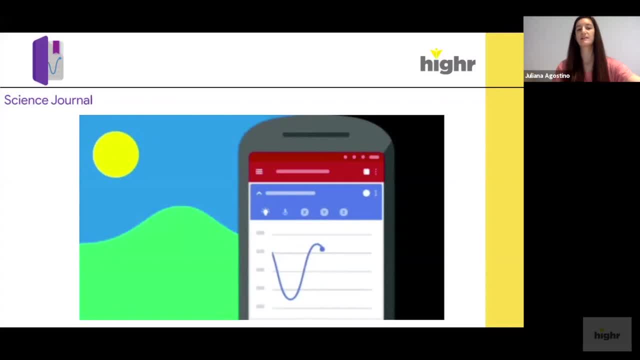 their own investigations. There's so many different possibilities. For example, this year our grade 10 students normally do a model rocket lab, but since we didn't have access to any of our equipment, we completely opened up our final investigation of the year. 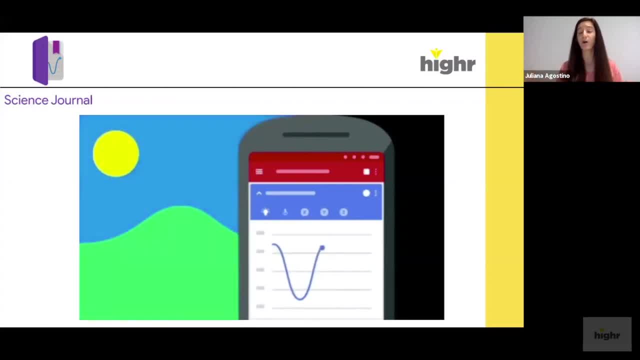 and told them to investigate any aspect of motion that they wanted. So we had kids doing very simple but things that were interesting to them like: can I throw a ball faster with my right hand or my left hand? Is my acceleration different when I run uphill versus downhill? 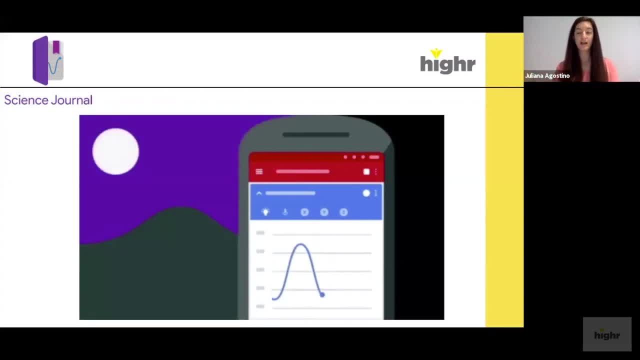 And they were able to collect that data using Google Science Journal and another app which I've made available in my Google Doc called Vernier Video Analysis. All right, so at the end of the day, let's say that your students maybe don't have access. 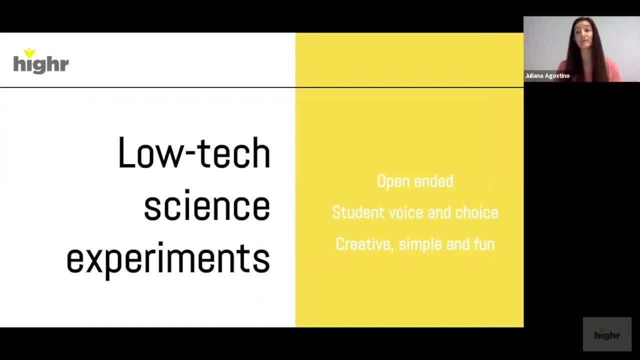 to all these simulations and apps. It's just not going to be possible for everybody And, as mentioned before, equality is key here. So let's talk about some low-tech science stuff that kids can do at home, Just because they don't have all the bells and whistles. 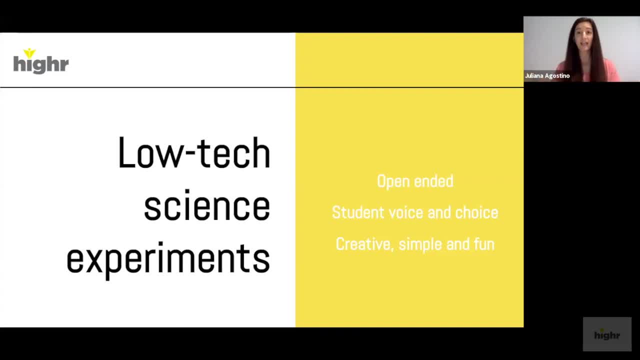 of the newest tool doesn't mean that your students can't engage in some meaningful scientific inquiry on their own. There are plenty of ways we can spark their curiosity. The key is to incorporate as much student voice and choice as you can and make connections to their own personal experiences. 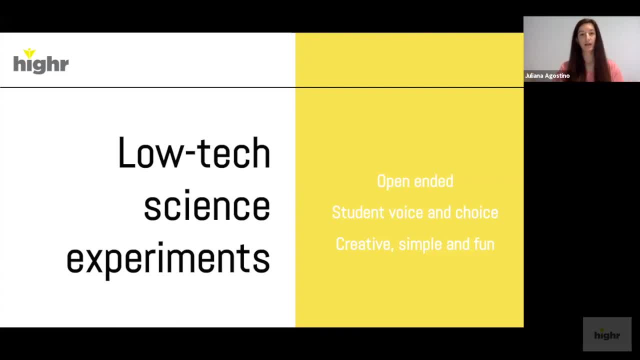 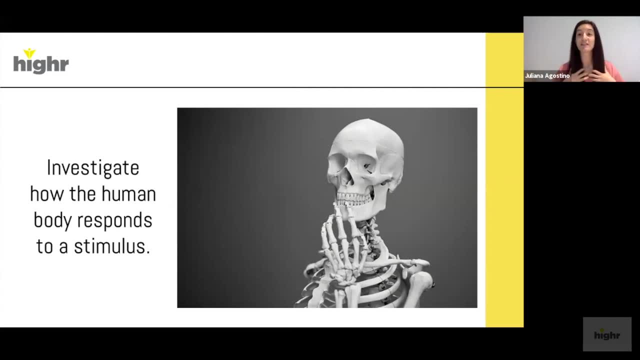 in the real world. So here we can get really creative. So, for example, we modified our Grade 9 biology unit this year and made it about how the students experience their own bodies on a day-to-day basis: I'm hungry, I'm tired, I'm feeling sleepy. 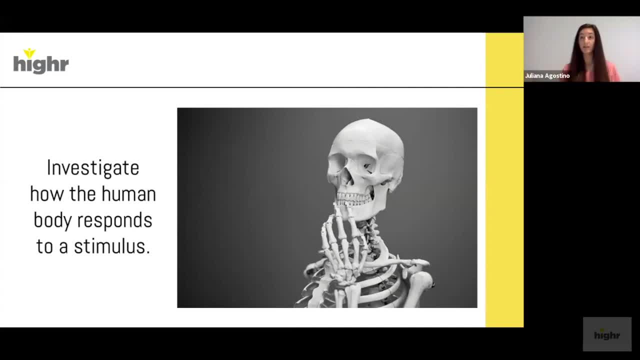 I'm feeling cold. What are the different stimuli that are causing their bodies to respond this way? So we had students investigate anything that had to do with a stimulus and a response in any part of the human body. So they looked at the effects of caffeine sleep. 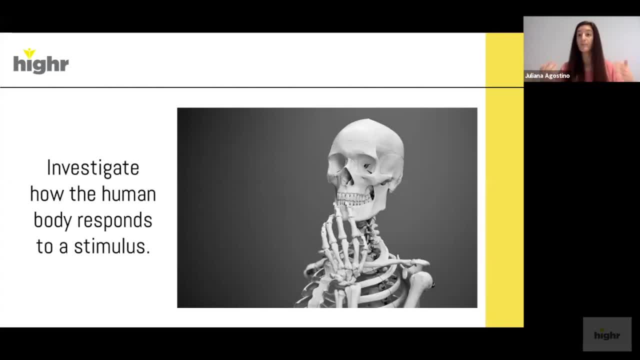 exercise. they looked at variables like heart rate, blood pressure, body temperature, reaction time. I had one student design an entire investigation from research question all the way to evaluation, and all she needed was her sister and a paperclip And she was able to use the two-point discrimination test. 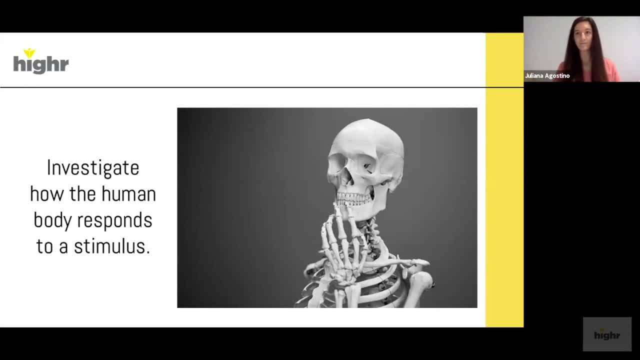 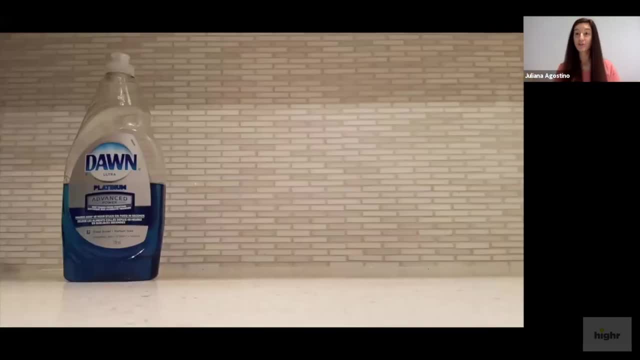 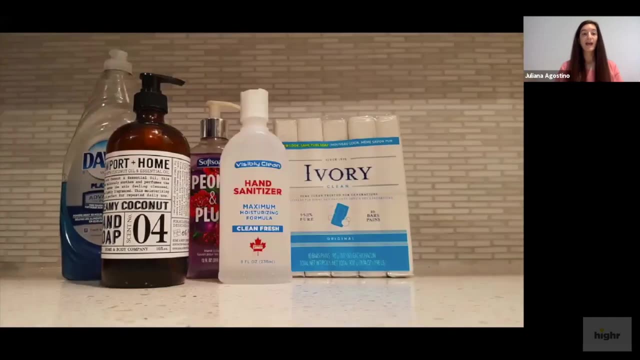 to learn about sensory neuron receptive fields, and she didn't need any crazy equipment. In our chemistry unit we took advantage of another student experience, which is the current global pandemic. So we modeled for students a very simple experiment where we had them test the effectiveness of soap. 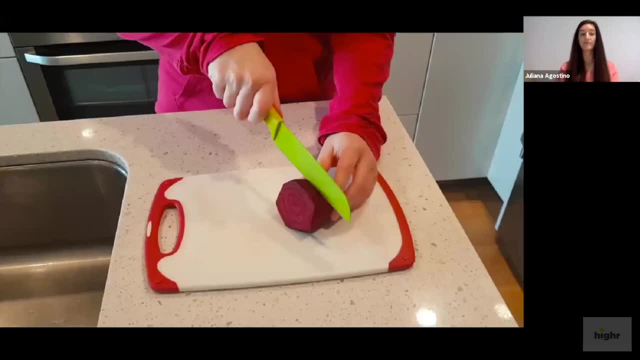 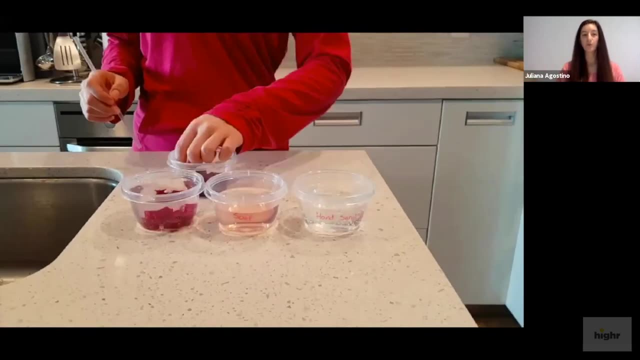 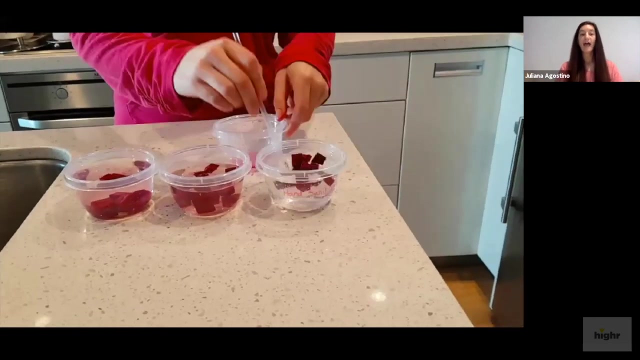 versus hand sanitizer. on the SARS-CoV-2 virus envelope, We used beet cells to model the viruses and we placed them in different solutions, using water as a control. Students were able to then qualitatively detect the level of cell membrane disruption based on how much of the pigment. 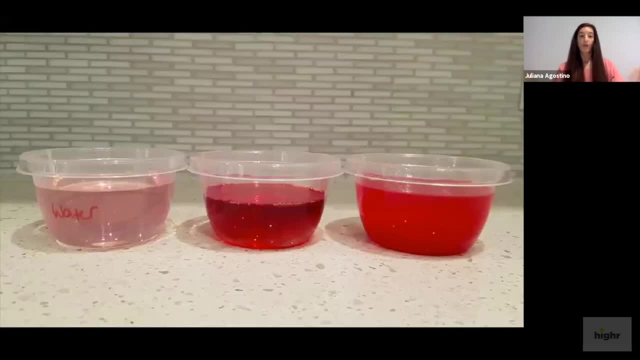 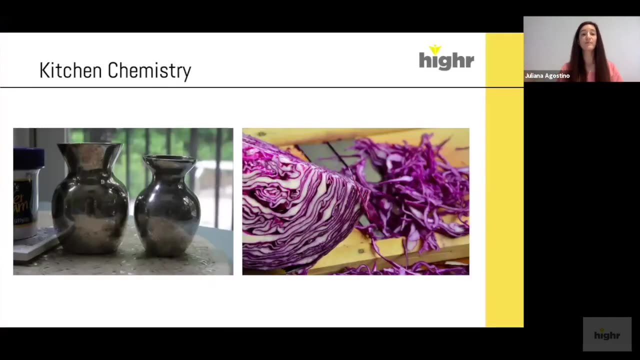 was leaking out of the beet cell vacuoles. So, again, this led students to design their own investment investigations into chemistry of everyday products. One thing you could do would be give your kids a challenge. Can they take a harmful household substance like a cleaning agent? 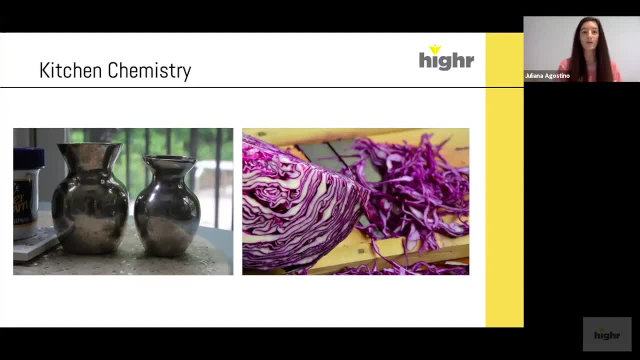 and figure out the chemistry behind something that would be a little bit less harmful, like polishing silver with baking soda and aluminum instead of a toxic chemical? Or could they create their own pH indicators? All they need is a little bit of red cabbage, and then they can go. 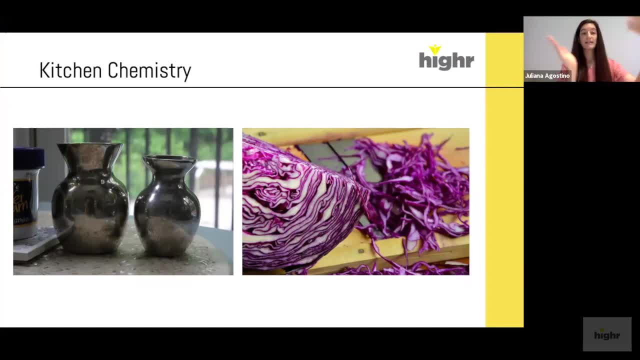 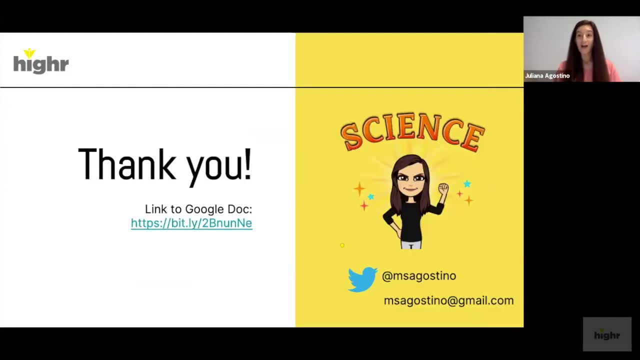 around their house testing different chemicals And right there they've learned about single displacement reactions from the silver acids and bases from the red cabbage. So that was a lot. I'm sorry if I talk too fast. Everything I just said is in this Google Doc, all the links to the apps. 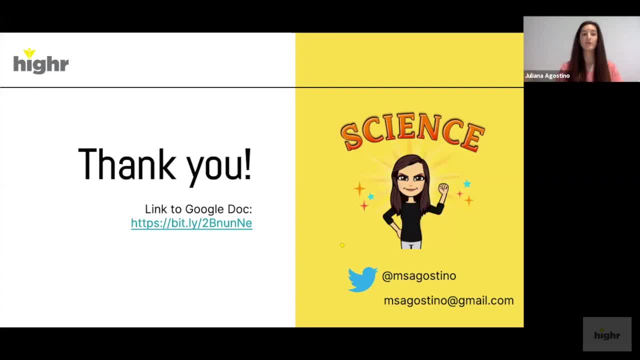 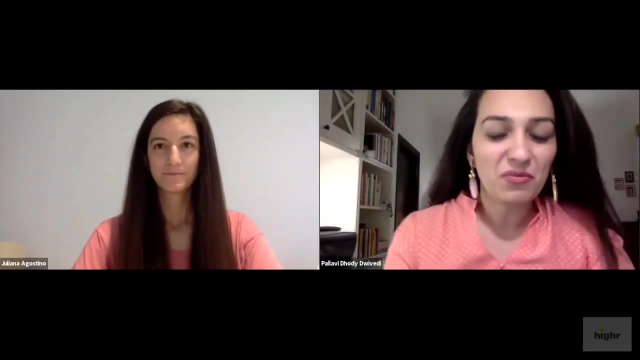 and tools that I use, and more. So feel free to visit that page or get in touch with me through email or Twitter if you have any questions. Thank you very much, Juliana. wow, I think I have to say that I was absolutely floored with all of those. 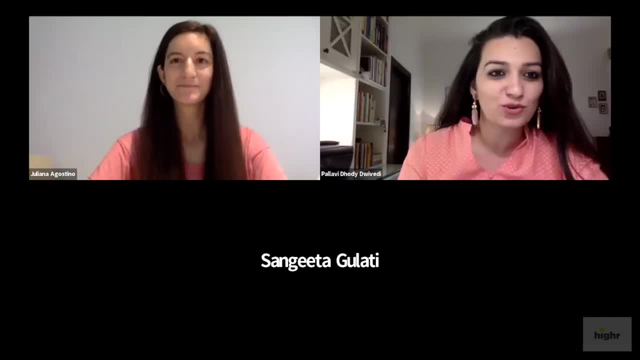 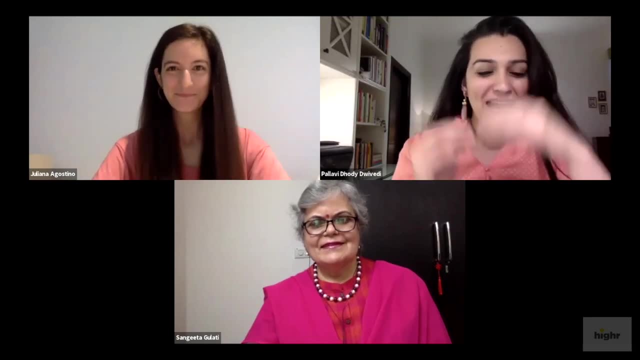 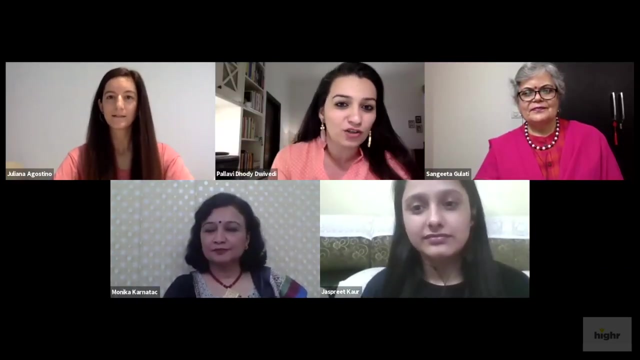 amazing kitchen experiments that you showed us how to do. I almost want to actually run down and get myself a beat and try that activity afterwards now. So much fun And I'm sure so much fun for the kids as well. Something to do at home in a lab-like setup. 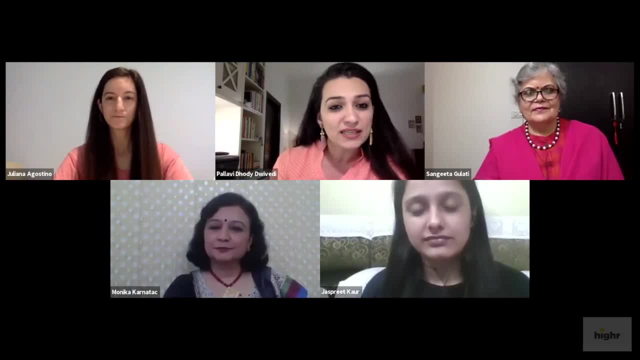 So what an amazing idea, And really all of the different things that you talked about in terms of getting students to actually eat, Students to actually engage with science through activities that mean something to them, Like which of the balls, which of the hands can I use to throw a ball? 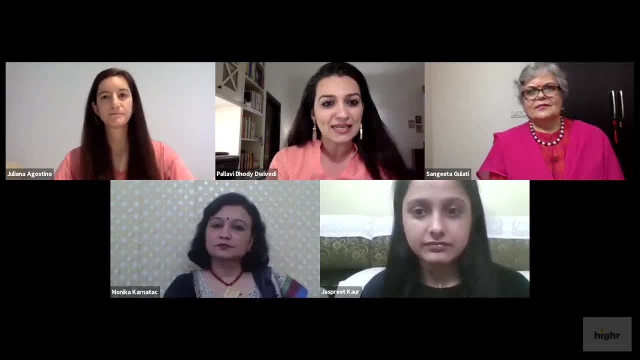 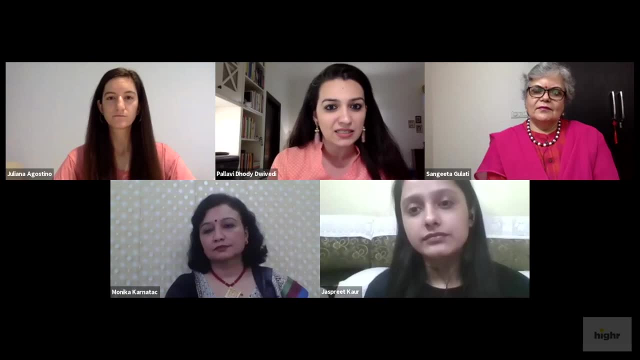 that would go faster, And those are exactly the kind of real-world connections, as well as inquiry-based activities, that you know we really want to build into our teaching And, like you said very rightly, we don't require any kinds of fancy tech. 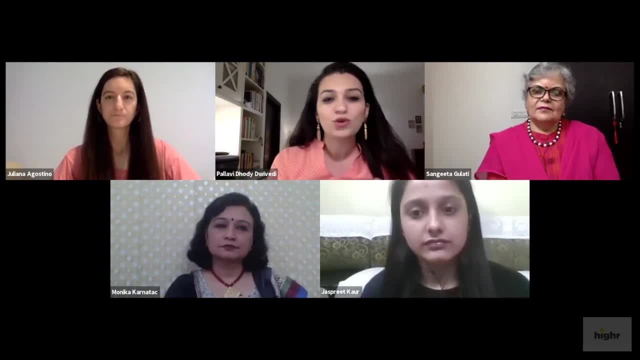 to do a lot of the stuff that we just want to do to get better. We just want to do what we want to do to get kids engaged and involved and thinking about the world around them. So thank you so much. Some fantastic ideas in there. 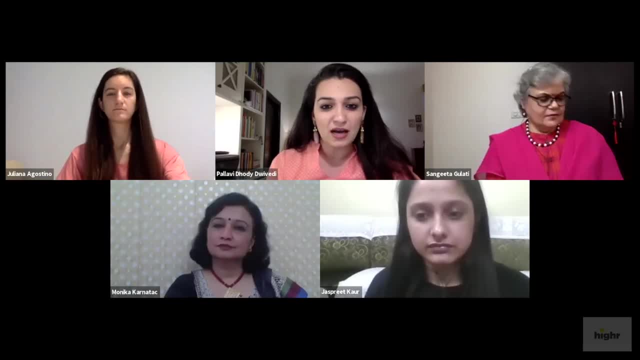 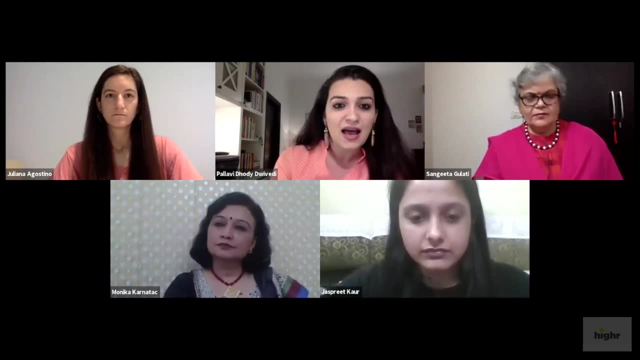 Great stuff. A couple of questions that came in which I thought I could just throw out there for all of you. There was something, there was one particular one about assessments, And how is it that- and I'll open this out to both math and science. 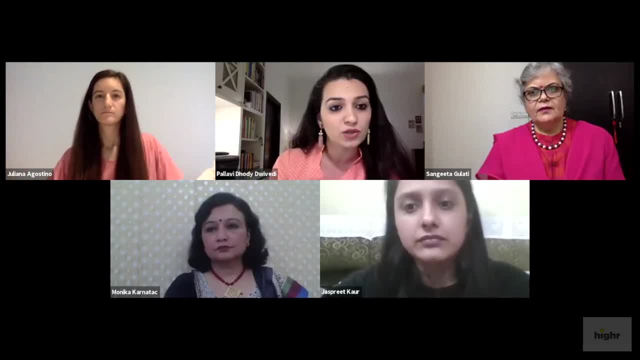 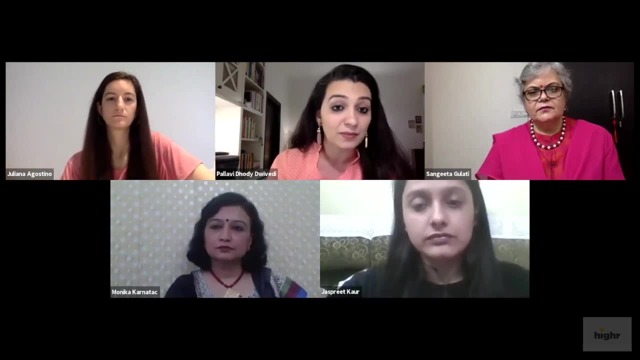 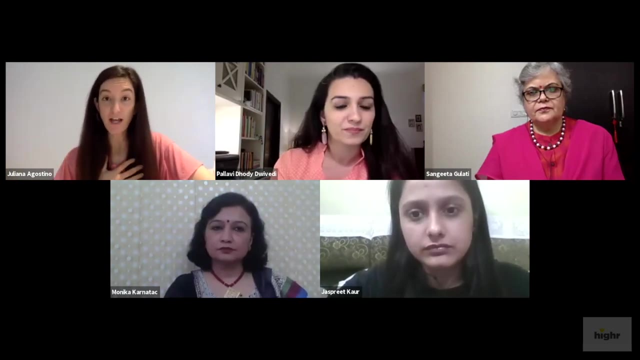 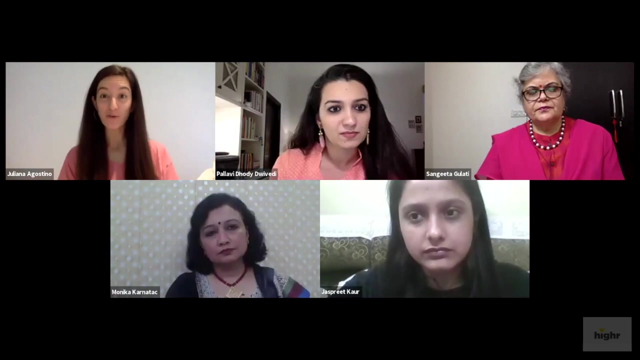 faculties on the panel. But I'll start with you talking a little bit about how are you getting students to undertake any kinds of assessments online, particularly for science- Sorry, for science. So we had to kind of modify our assessments this year, So we decided as a school that we would make all of our assessments open. 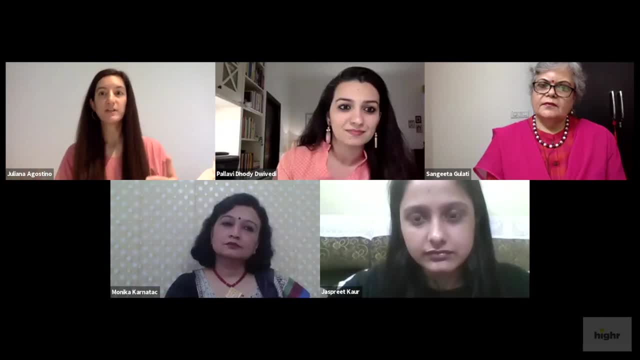 books, So we didn't have to worry about. are students going to be cheating by using their notes? Are they going to? is the technology not going to work? Do I have to do? we have to find some kind of program that will lock their 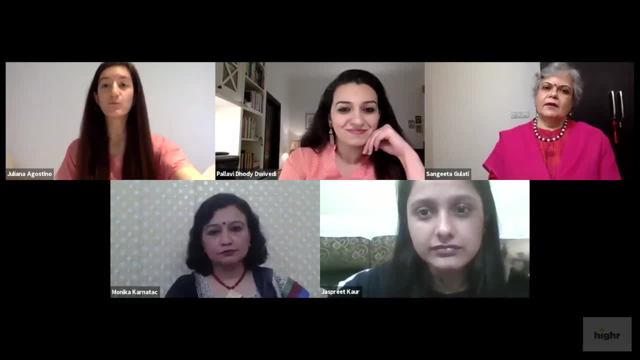 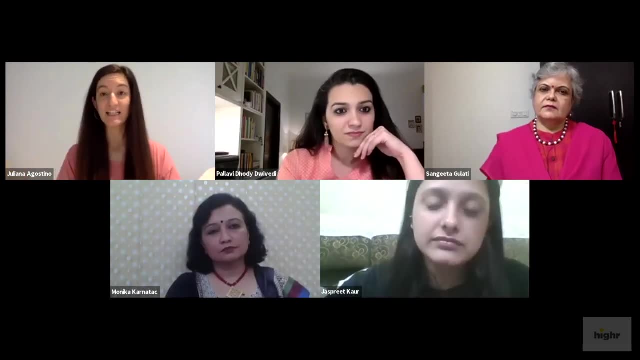 computer so they can't cheat. So we actually just moved away from tests this year and moved to more open-ended assessments. So for example, in our grade 10 science this year we did case studies Right So students could use all of the notes that they had. 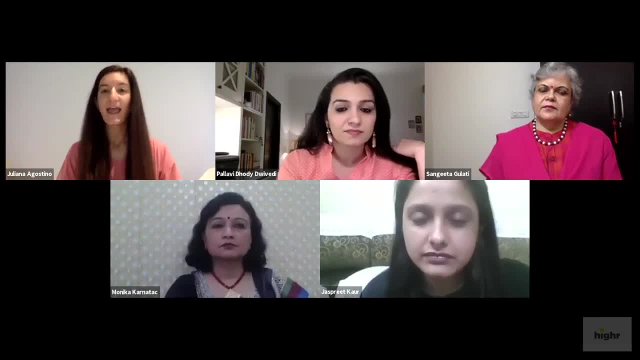 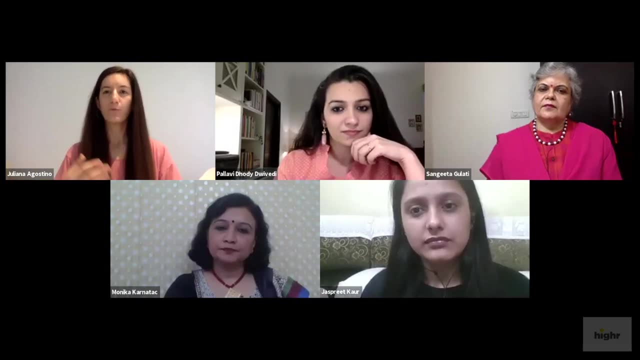 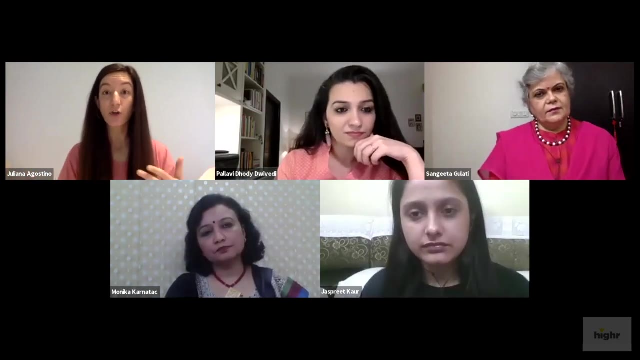 They could use the notes that they had created through the online semester And we gave them a case study that they'd never seen before And they had to work through that case study. One of them was about evolution. One of them was about actually blood type and your risk of getting 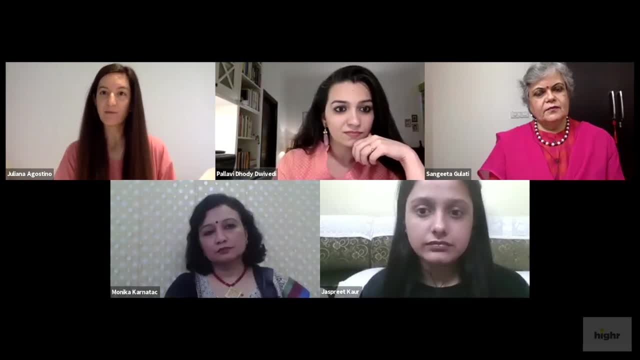 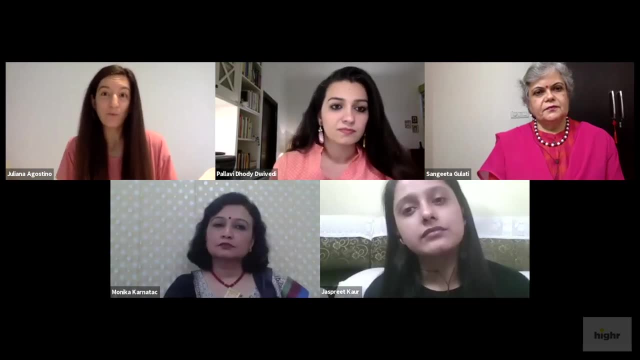 SARS-CoV-2.. So we just we switched to a different type of assessment for a different type of environment. We just didn't feel like writing a test is really what works in this scenario. So we did a lot of case studies. 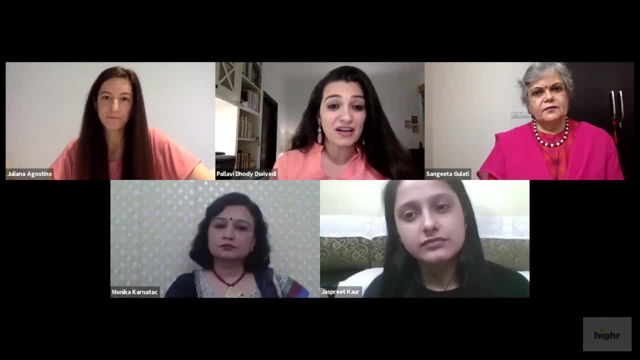 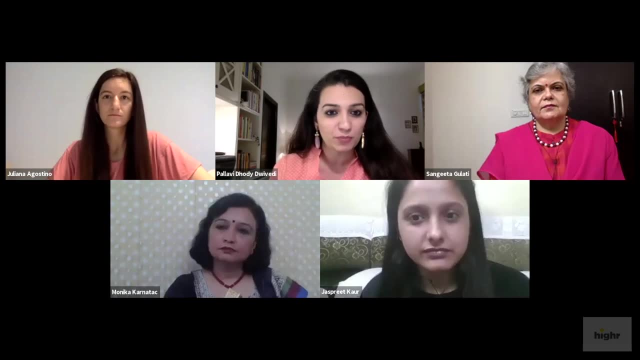 I did that for all of my classes this year. Okay, Fantastic idea To move away from pen and paper tests and exams to more open-ended projects that are focusing more on measuring student learning more than anything else and more engagement with a particular activity. 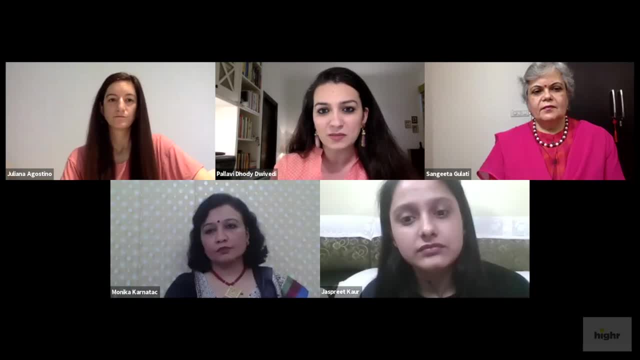 Sangeeta, would you like to talk to us a little bit about math assessments, Especially the issue around how do I know if the kid, if it's actually the child, who solved the entire problem themselves? Yeah, that, of course, is the question that, in fact, all the school leaders. 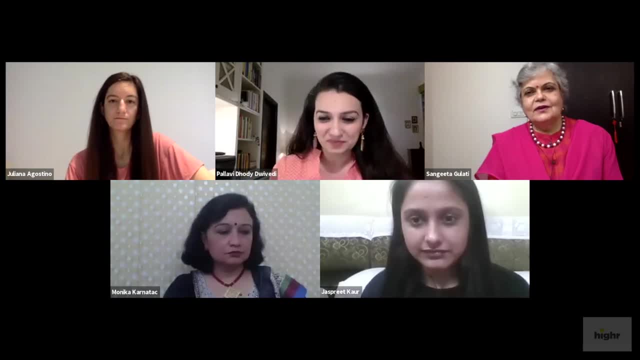 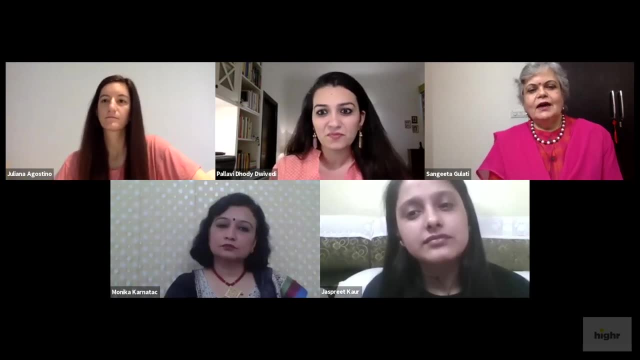 and concerned. you know stakeholders are asking and thinking about, But we'll have to trust our children First of all. we'll have to make an effort to give them an opportunity to feel that they are responsible for themselves, And we have done that. 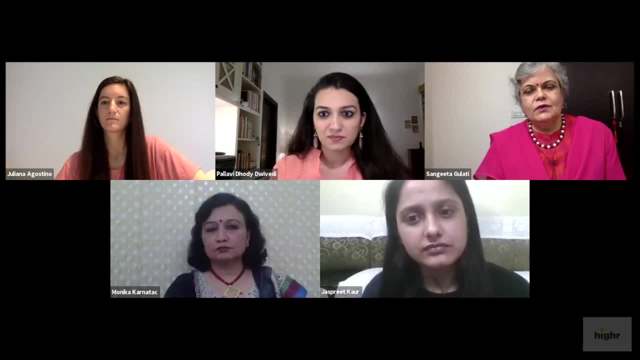 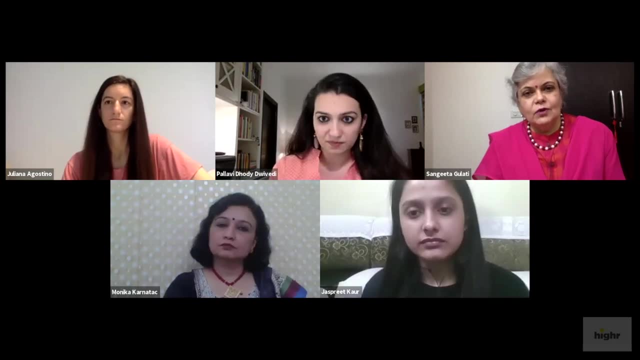 So we definitely, you know, one. in terms of the formative assessments and in terms of self-assessment, we've been depending heavily on Google Forms, But we did have- for our grade 10 and 12, we had a round of practice test. 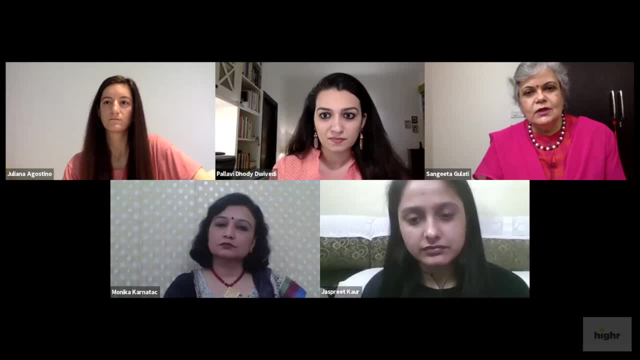 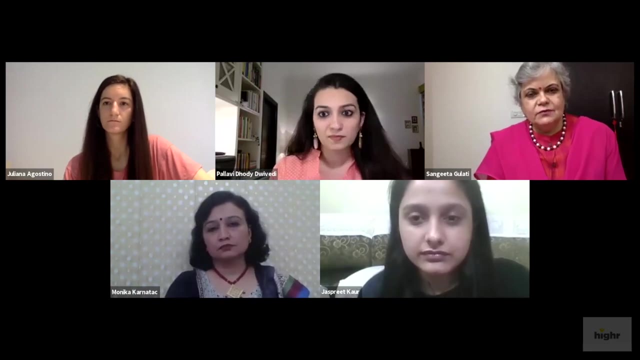 slash unit test kind of thing, through Google Classroom And we made them join a meet session, We opened the paper exam, We assigned the exam at that particular time And they had to submit the scanned copies within those 40, 45 minutes. 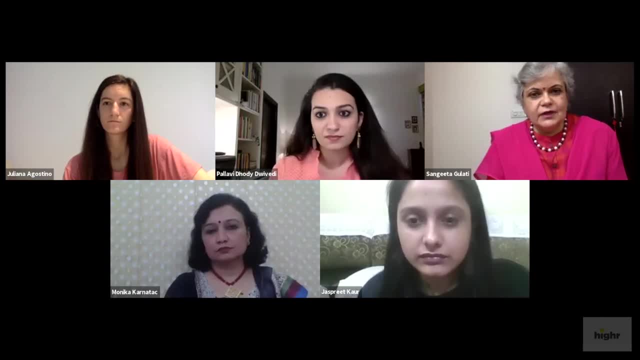 But they were not sitting in front of the camera, So their cameras are off. We are not supervising them, But surprisingly- or rather happily, they surprised us. None of them actually seems to have copied the solution from somewhere. They've all submitted a very genuine work. 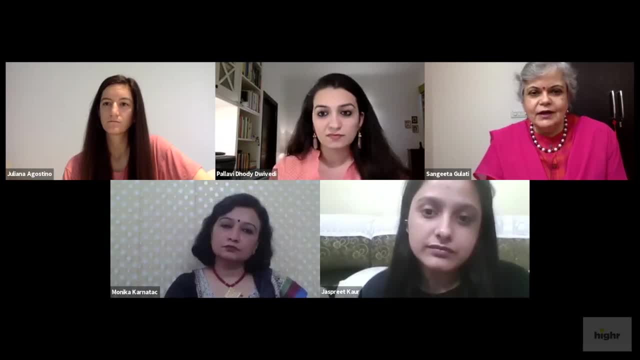 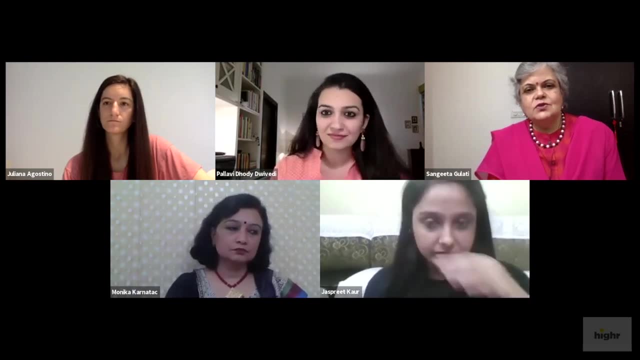 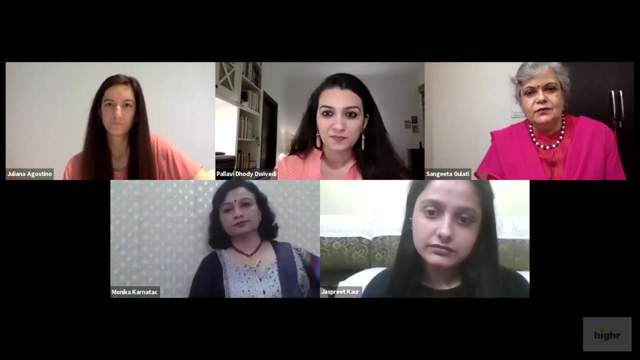 And so not everybody has bought our, you know, 40 on 40 kind of a score. They all have done exceedingly well, just as they would otherwise. So I think it's time for us to trust the children And, at the same time, what Juliana has said is something that we all around have to bring in. 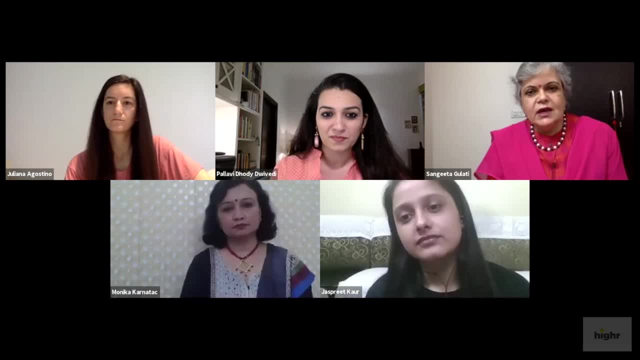 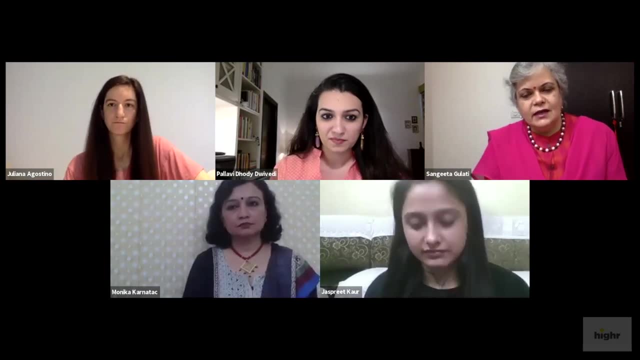 We have to change the way we teach and the change the way we assess. Both the things go hand in hand. I cannot just open a case study at the end of the year when I have not taught them that way, So I can't do that. 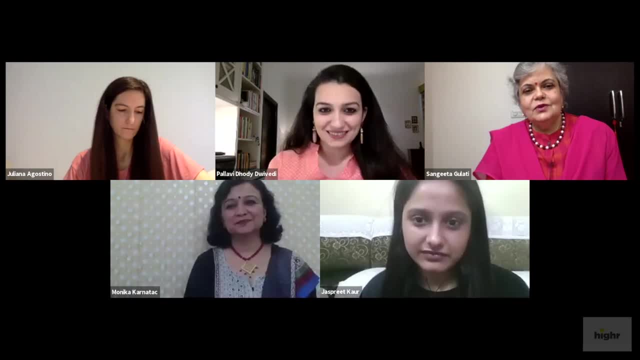 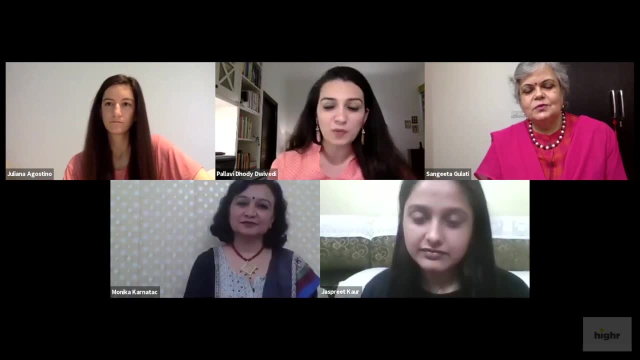 So we'll have to change the way we teach, And then only we can change the way that we assess. So our lesson was, you know, we found them to be Yeah, So they really, our children, had really proved, you know. 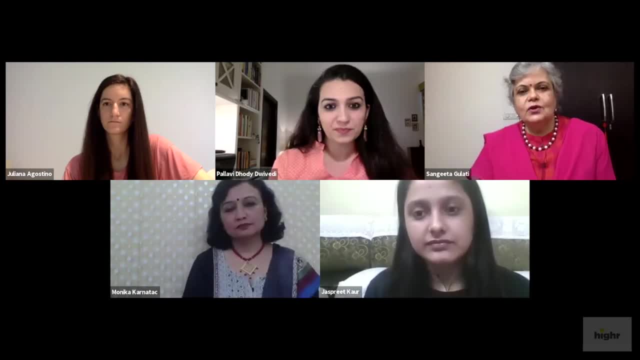 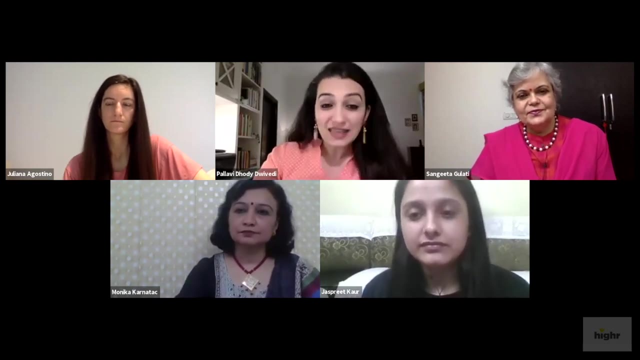 that they can be trusted and they would not cheat as so. So we are trying. you know different ways, But this is Somehow something that did work for us in the month of May, that we then we did it Wonderful. Thank you so much for that. 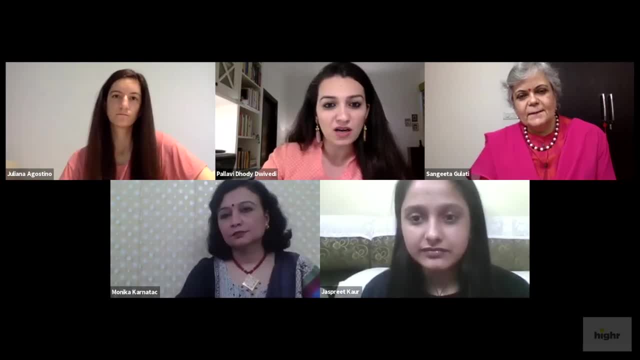 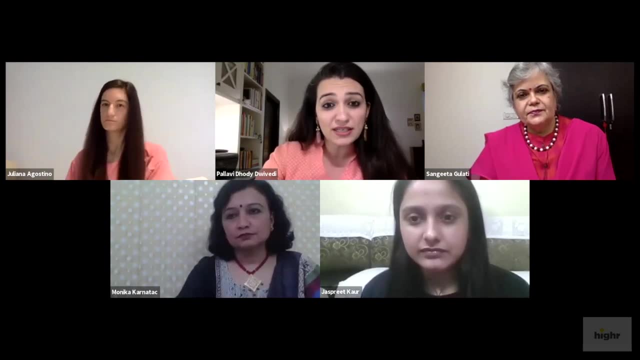 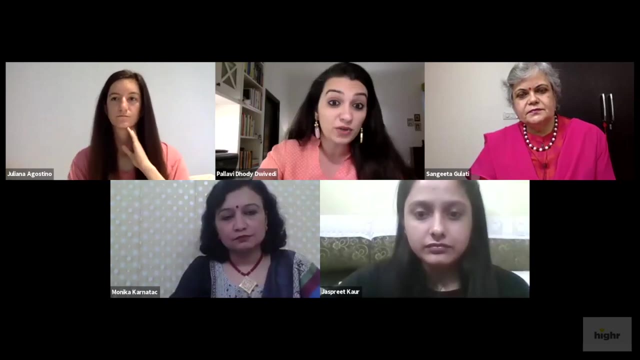 And a very important lesson there, also about- And I think also something that Monica mentioned earlier on in the session- about, you know, grace over greed. really, You know, do we? do we really just want to hammer down on assessing students in ways that were previous, that we were doing previously? 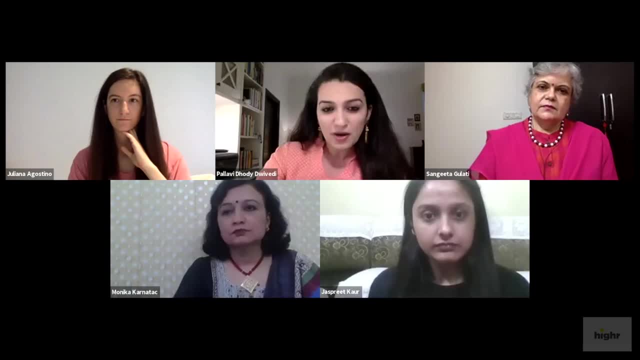 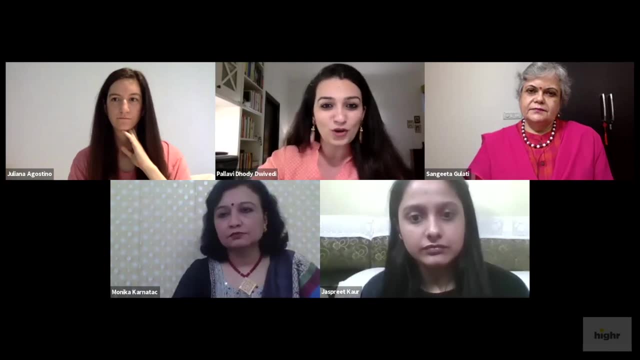 So maybe, if we change some of the ways in which we teach, we might also be able to change some of the ways in which we assess. So, on that note, moving on to our last panelist for today, Jaspreet, Jaspreet, thank you for joining us. 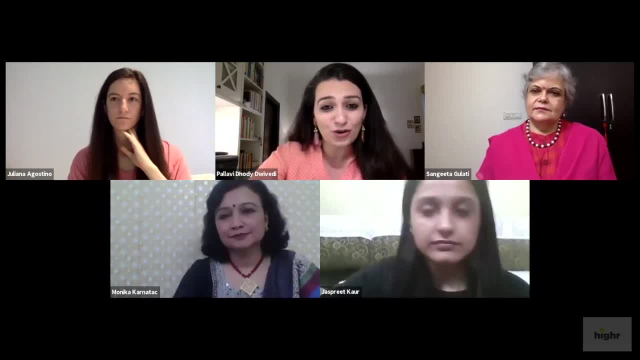 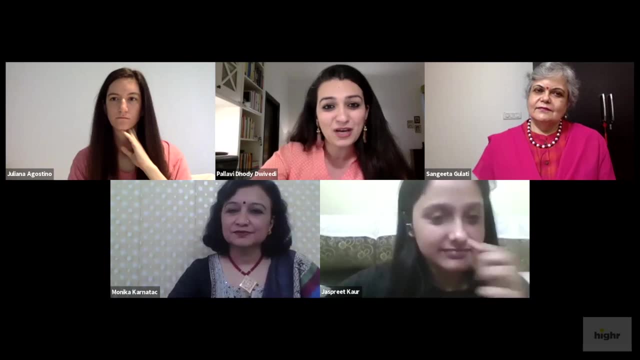 And thank you especially for joining us, Given that you're quite unwell today. Thank you for taking the time to be with us and to share your insights. That's so, so generous and magnanimous of you. Thank you very much. 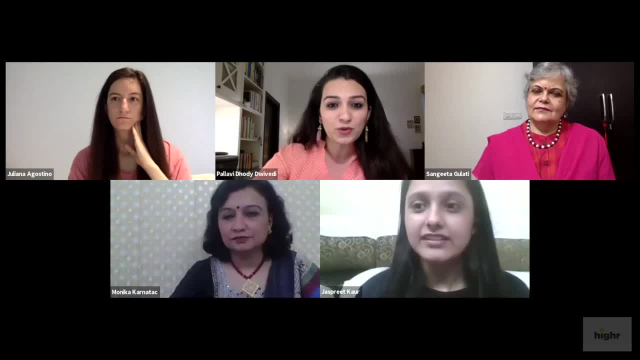 So over to you, Jaspreet, to talk to us a little bit about what you've been doing with your primary work. So over to you, Jaspreet, to talk to us a little bit about what you've been doing with your primary school students. 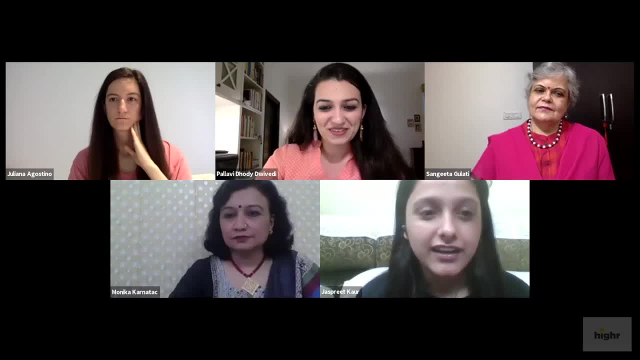 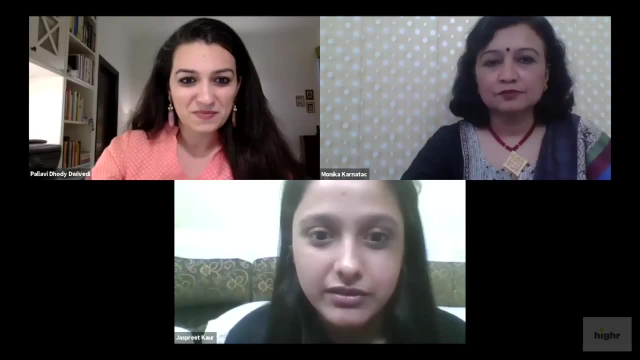 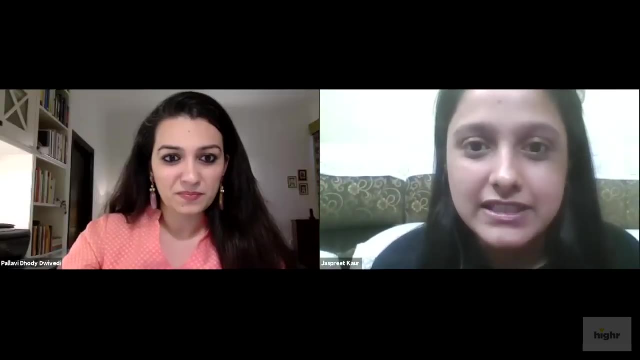 Thanks, Pallavi, for inviting, and I mean it was really hard to join, But then I really wanted to share the insights on primary years with you all. So I think to your question, which was open to the entire group, like how assessments can be done. 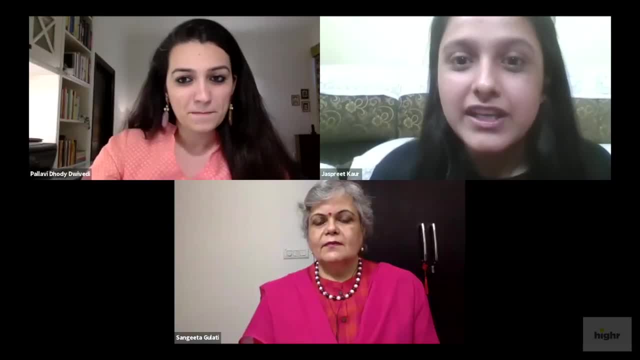 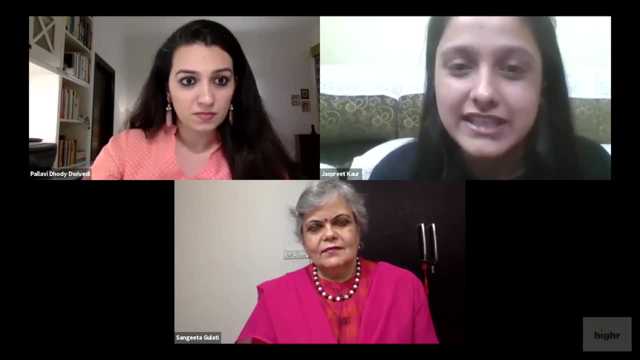 So definitely, as Sangeeta ma'am said, that we need to trust our children number one And we need to actually give children the taste of what they're going to get in future. So if we're saying that it's going to be an open ended project, then the teaching has to be in the similar way: that they get an insight into how it is and all the steps of doing it. 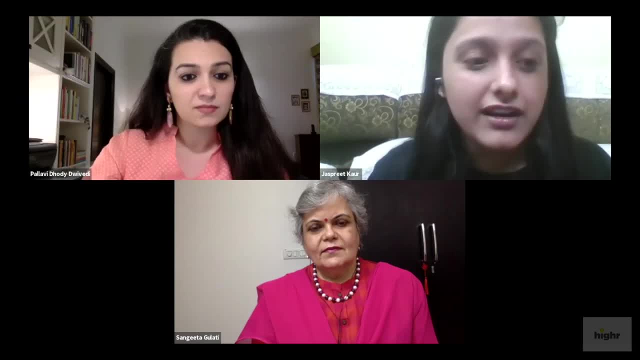 So that children feel prepared and they feel supported when they are being assessed. The other thing that we've used recently with the children is to have an oral test with them where the teacher just has to call the children away and be prepared with two to three MCQ questions. 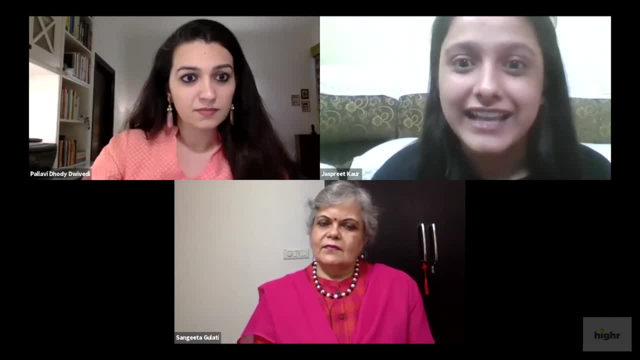 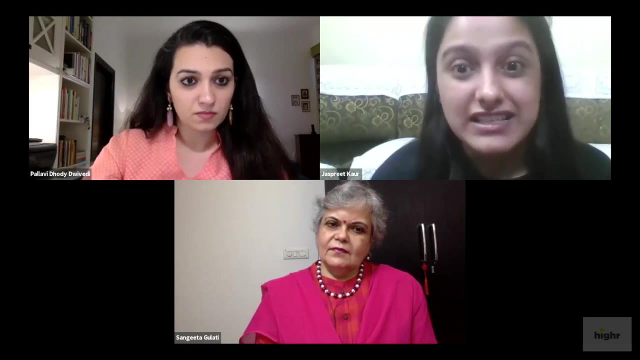 The child is supposed to solve that in front of the teacher And that actually reduces the risk of failure. And that actually reduces the risk of failure. And we know with Sangeeta that counting down is an expensive process And that the child does have an SEO model where the teacher just Explained from disagreeing with students, which will make them more curious about the course and what it's all about. 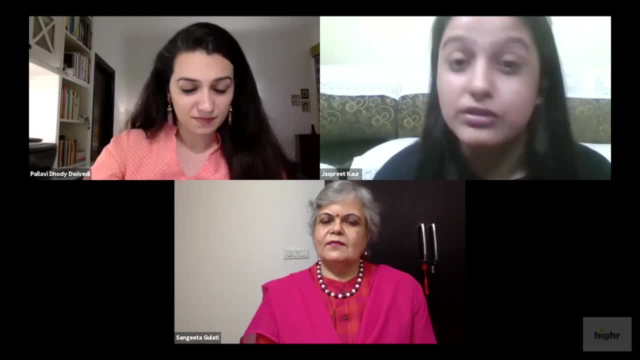 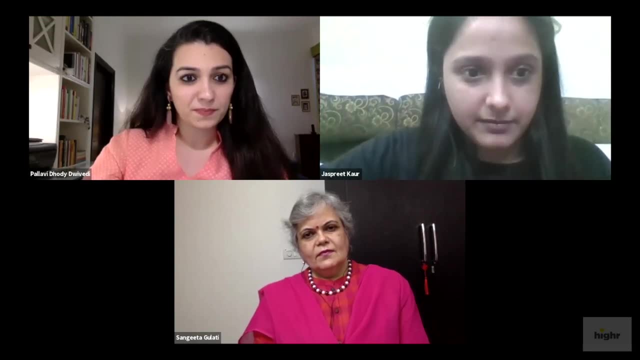 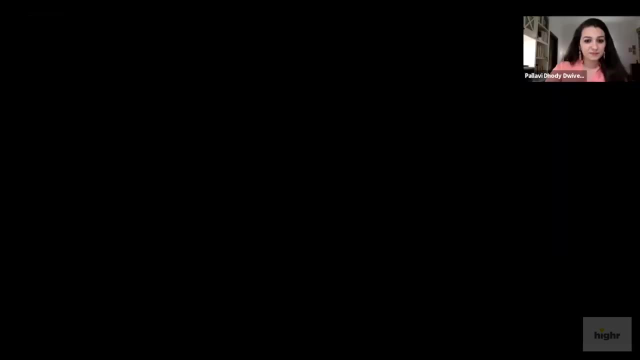 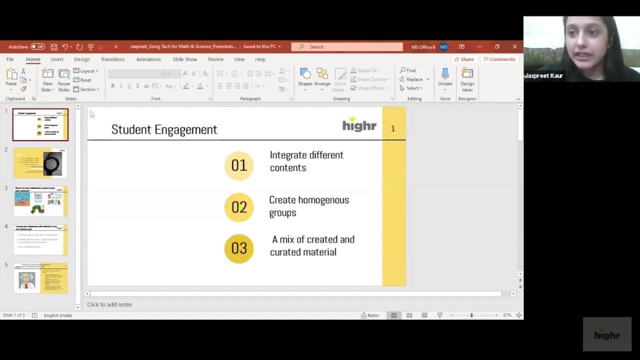 teacher to be informed and know what exactly they should they do next. all right, let me know if you all can see my screen. is that visible? yes, it is, thank you. so I'll quickly take you through different parts of engaging children during this COVID time. given that it's a sudden- it's a sudden change for a 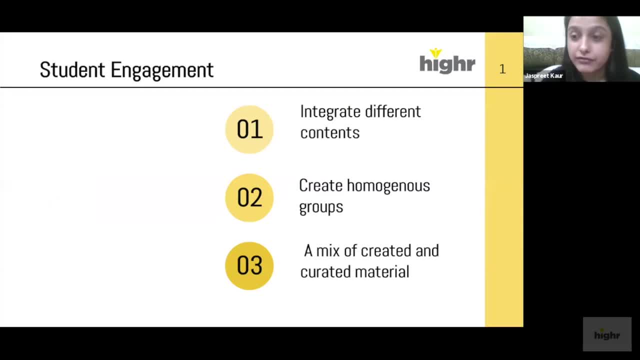 lot of sectors so, specifically for the sector that I've come from, I work with underprivileged children. it is really hard to make sure that you know the first-generation learners, or probably second-generation learners, are actually engaged when their parents are looking for bread and butter and the simplest of 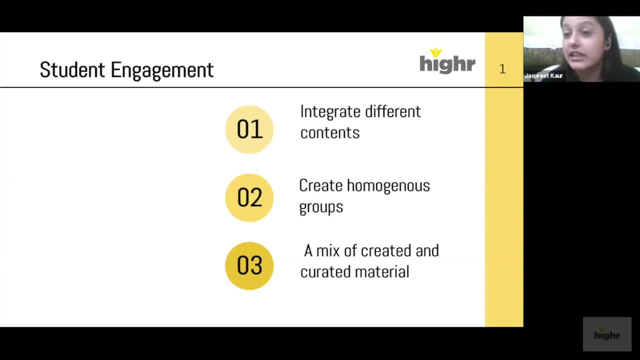 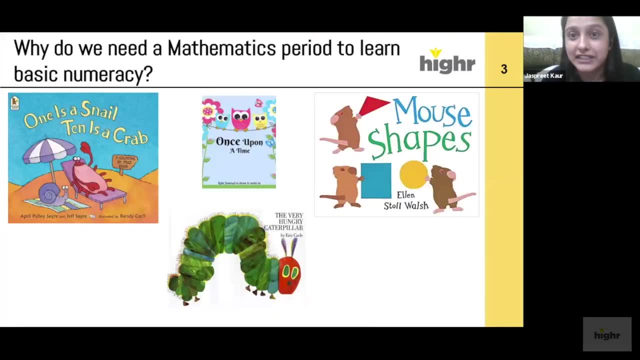 the solutions, which is already there in the air, is to integrate different content areas. so why do I actually need to, you know, have a mathematics period to learn basic numeracy or to learn about shapes, when it can be simply done with a lot of stories around us? so when we talk about children, we have to, you know, like the 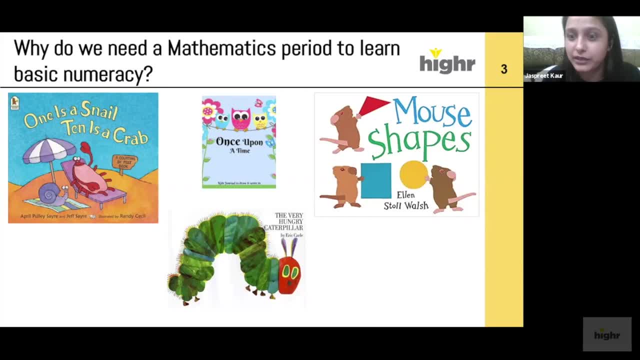 spark in for that curiosity what these numbers are. I don't have to teach them that, it can easily be taught with different subjects and, you know, while we are developing language, we can give equal importance to, to inquiry, to numbers, to science around us, environment around us. so I think that 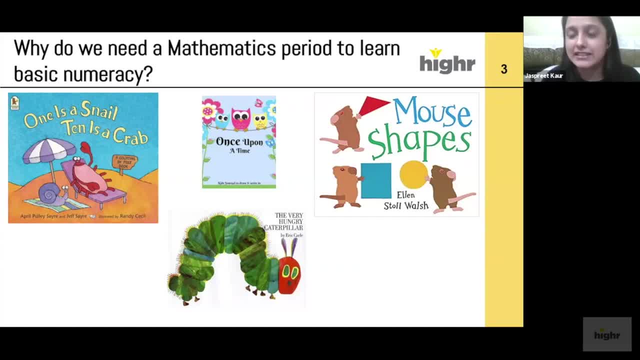 there is no need to have a particular mathematics time and say, you know now, now we're going to learn about numbers, or now is the time to learn about shapes. now it can actually be done with other content areas and then, slowly, that fear of learning science and maths goes down, where it gets replaced by inquiry, by 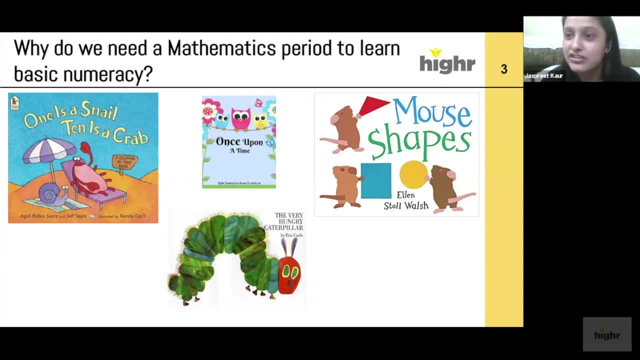 curiosity by creativity and still. you know I was mentioned in the last lecture- There are different ways of doing it and once children get a sense of that they can achieve, they can find out various solutions. they will definitely have an interest in the subject. So I think it needs to be integrated with other content areas. 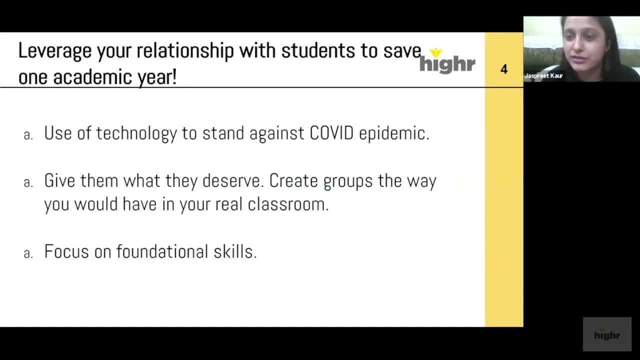 The second thing: you know, while everybody is figuring out different types of technologies, Samita ma'am has given tools that everybody is appreciating, and we actually need such tools for children to practice things at home. I, particularly for primary years, feel that we need to leverage our relationship for our 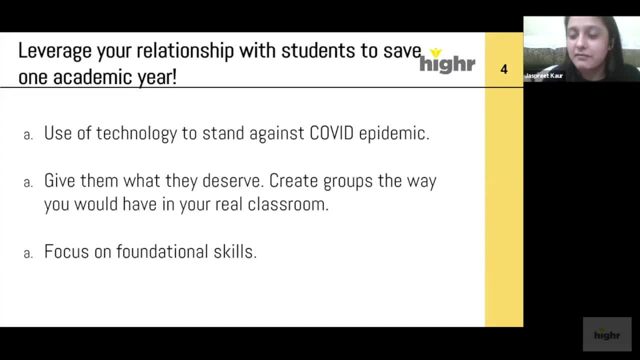 children to be, you know, be ready with, and be ready with all the knowledge that they need to have to be able to jump to the next academic session. So a few months have gone out of this academic session and we're still figuring out which. 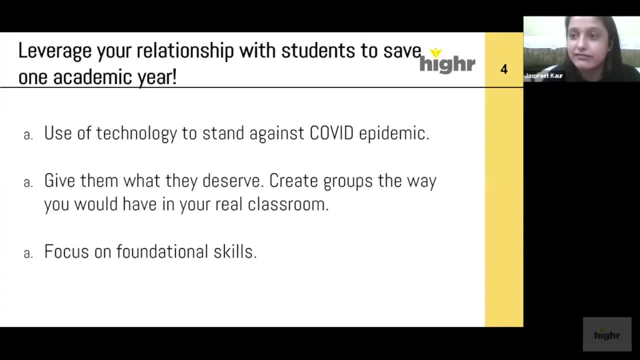 technology is the best and the best part is that everybody's you know. figuring that out, finding that out- Okay, There are different things available online. The thing that probably we need to figure out and everybody can you know, think about. 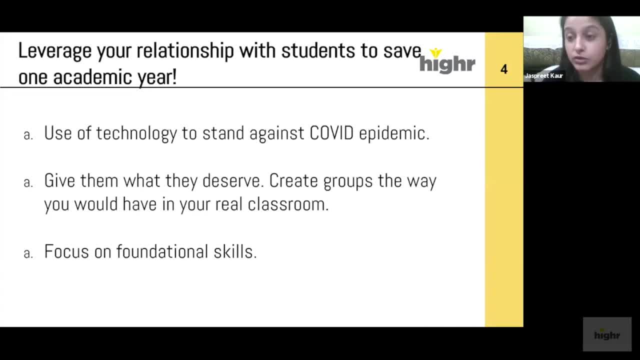 this, am I giving what my children need? So the tools that we're talking about right now here on the session are the tools that cater to one kind of learner. So am I thinking about different kinds of learners that I have in my class? 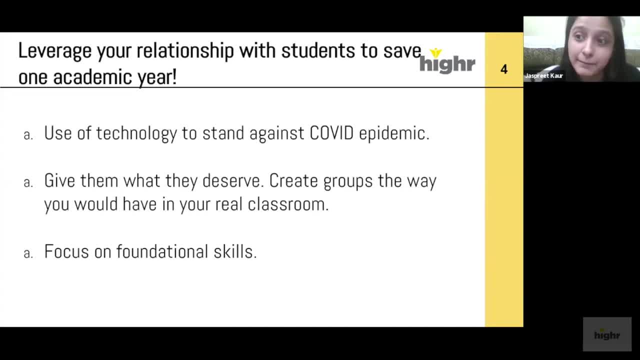 Maybe some children are kinesthetic learners. what do I do with them? Maybe some children who are audio learners, so they learn by listening. so is the teacher, is the school actually worrying about them, or are we still teaching the average? So, just like we do in the classrooms, I feel that different kinds of tools should be used. 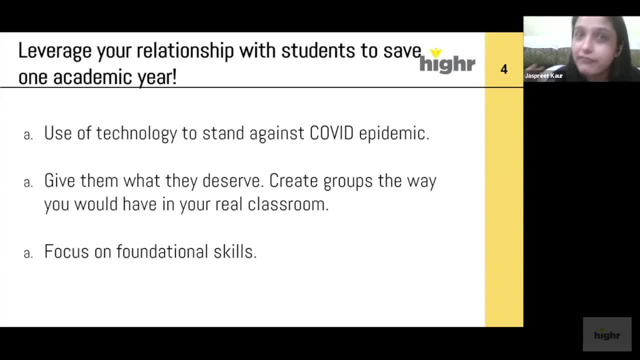 for different children. So if my children is fine with one kind of tool that the school or the teacher has chosen, the teacher certainly needs to also find out if my child is actually learning the right way, because that's what we do as teachers inside the classroom. 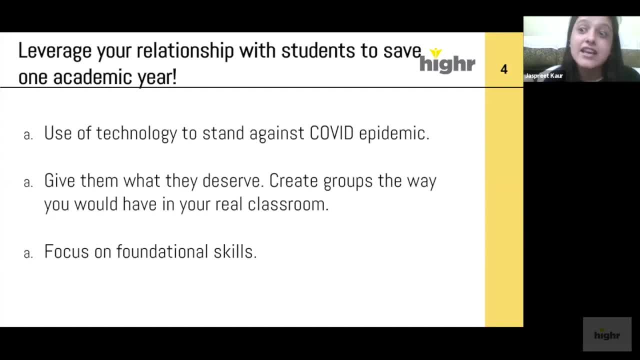 We cater to their needs. we try to find out the ways the child you know is able to learn. So I would say that's another missing step that we need to plug in to bridge the gap. And the last thing that I want everybody to think about is the foundational skills, like 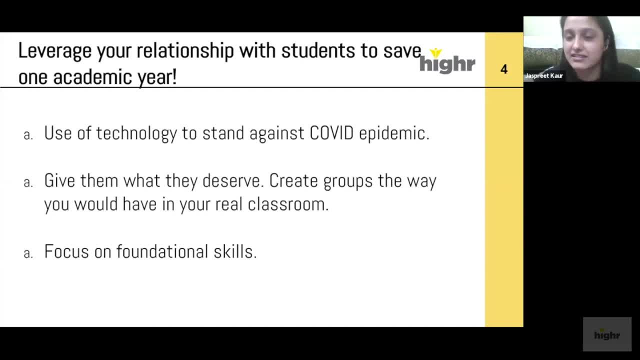 what's the hurry? I do understand that children have to jump to next level, but if you're moving to the next level, how are we making sure that the foundation is clear? How are we making sure that the foundation is clear? How do we make sure that the children's skills are still there? 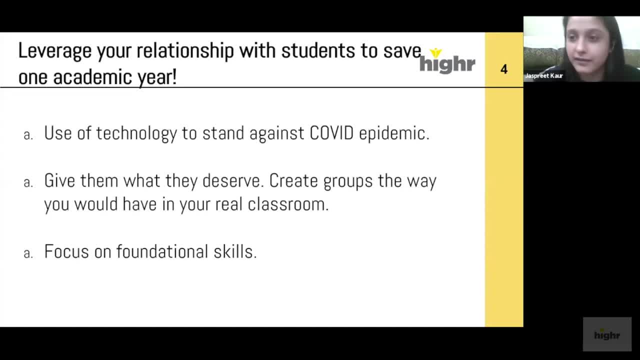 Because there has been a gap and there are children around us- if I talk about both privileged and underprivileged sector- who probably would have missed on a lot of skills during this pandemic or might have actually forgotten about a few contents. And you know, just because we're in a hurry and we ourselves are finding we all are in. 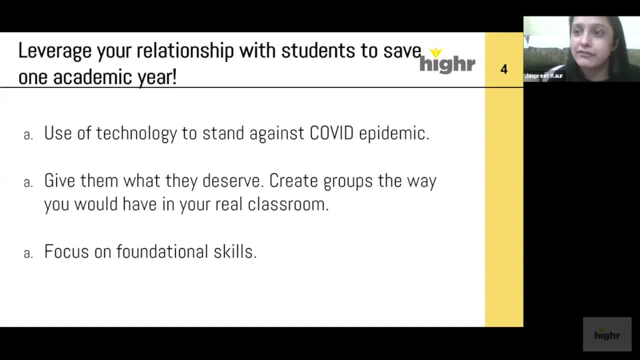 a scenario where we're thinking about what next? how do I prepare myself? We are facing many challenges And we are all in a situation where we are thinking about what next as we are forgetting about the foundational skills, like if we're talking about our time. how? 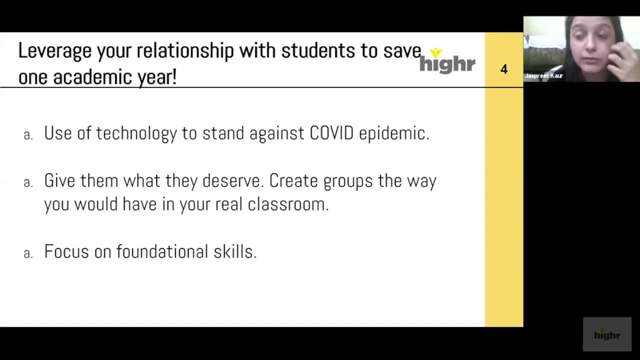 how did we actually start about with time, or if i mean, i'm talking about measurement and um, how and why was measurement needed? so all these foundations are actually necessary, which we might forget on the way. so let's just keep that another, keep that in our focus. 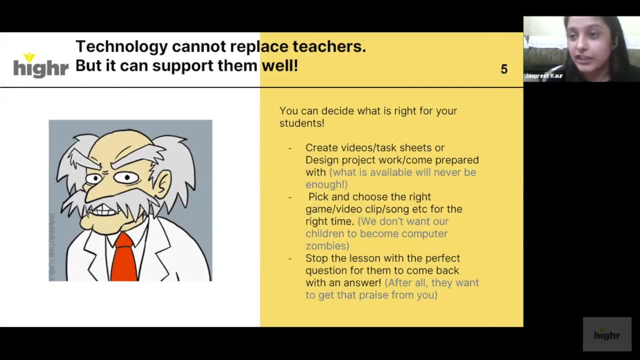 definitely, technology cannot replace, uh, the teachers, but it can support, and all these panelists that who are here have, you know, given us a lot of tools, the applications that are freely available, paid applications, tools that can help, but, uh, i feel, when we talk about primary years, 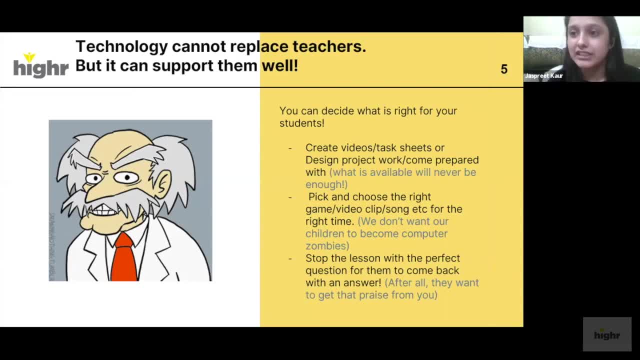 it's the relationship that the teacher builds with the children. it's also the right kind of mix that the the teacher needs to have, and so i think that's something that we need to have. so she needs to pick and choose: at what point should i give them this video, or at what 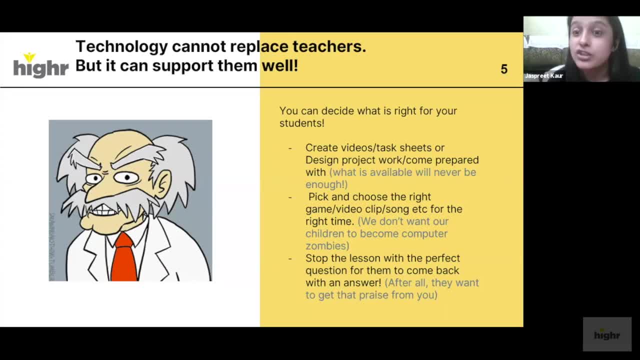 time do i ask them to open up this application. so if that choosing and picking up is not happening, you're probably not doing justice to our children. so their needs are different, so we have to pick and choose and look for resources that uh fits well with their needs and their understanding. the 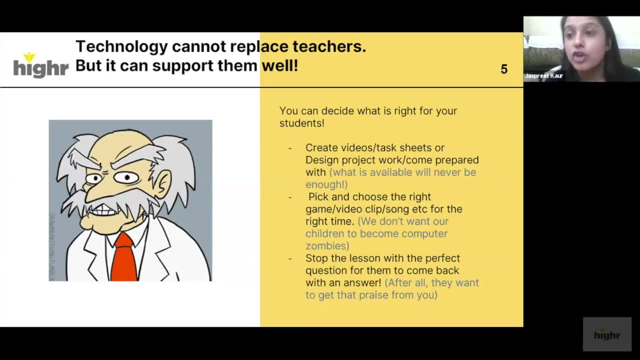 way they learn, uh, to talk about the curiosity and to talk about, you know, sparking the light in children. uh, that's another thing that we use at our school: to leave our lesson with a question, just like we do in language development or while doing a story. we leave at the right point for them. 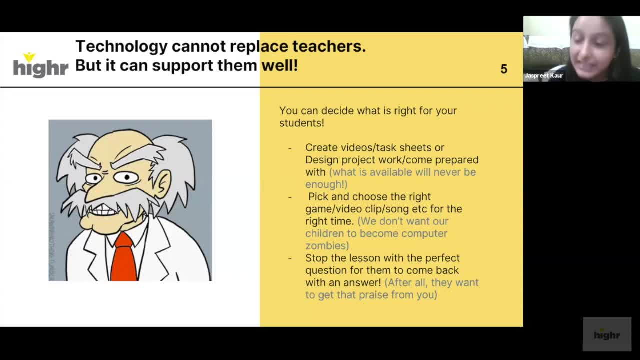 to go back, think about and then come back to classroom and give us different answers from their you know, from their fantasy world, or from their the way they think you know from the world that we may not have even touched. so similarly for mathematics, and i would say: let's leave them at the. 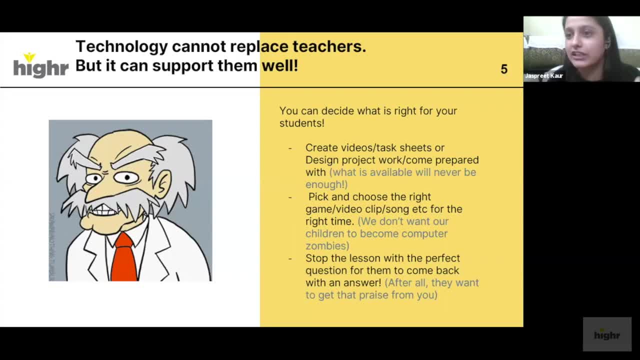 right time. so, for example: um, if we are talking about time, we have taught them: you know, this is the hour hand, this is a minute hand, uh, and we leave them. you know what? when the time is 4- 45, where do you see the shorthand? and when children actually see that time on a clock, they see that. 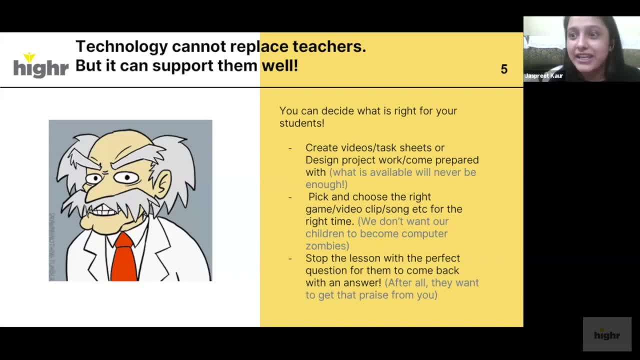 it's neither on four nor on five, so it's in between, and then they come back to classroom and tell us: no, ma'am, this is what i saw, and that's how you use your google classrooms or different kinds of assessment tools to know if my child is actually interested in what we're doing and if the 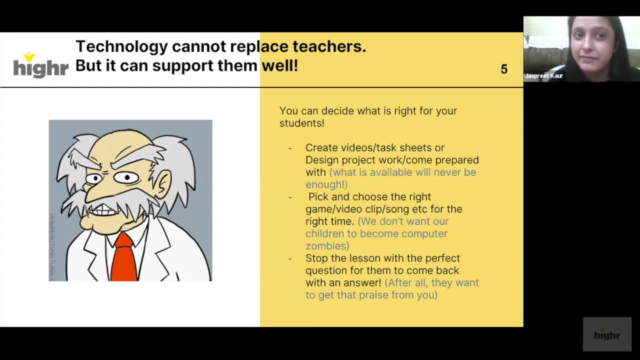 child is actually thinking about it non-stop and continuously. so, yeah, use what is available, but then don't think about the basic human features of children, that they need that soft touch. they still need, uh, the teachers to prepare for their needs and the way they learn. um, yeah, that's. 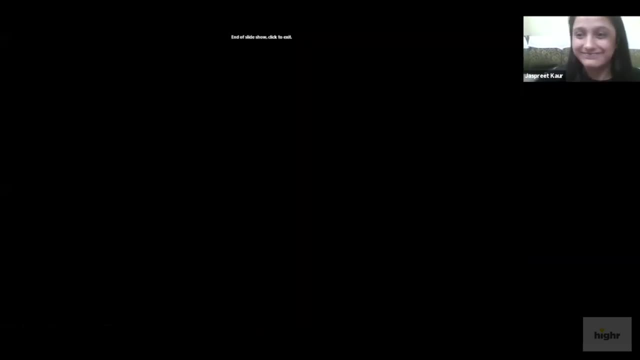 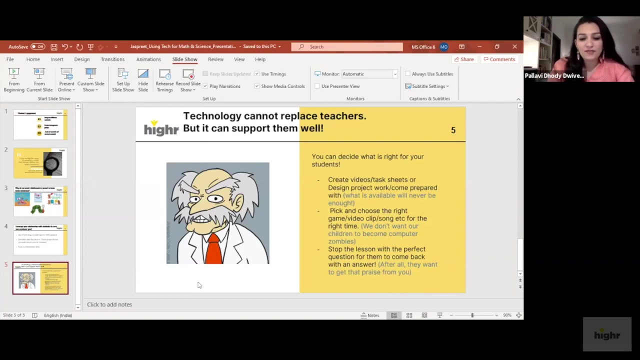 essentially what i had to uh uh share with the group. thank you so much for all of that wonderful insight and on, and thank you especially, just great uh uh. to end on that wonderful note about how uh students expect that we, as educators uh will respond to their needs, and much of that response is uh based on how well we understand. 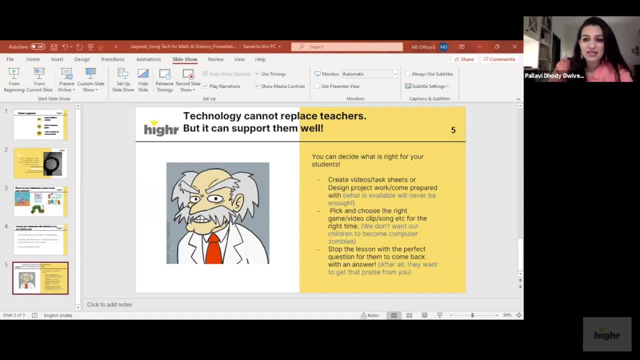 our students uh, and how well we're able to gauge their needs and, very importantly, at point in time when uh their known sources of comfort and uh their known sources of um, of understanding and of of sharing uh and knowing have been disrupted uh, because all of the uh all the schools are closed. they don't 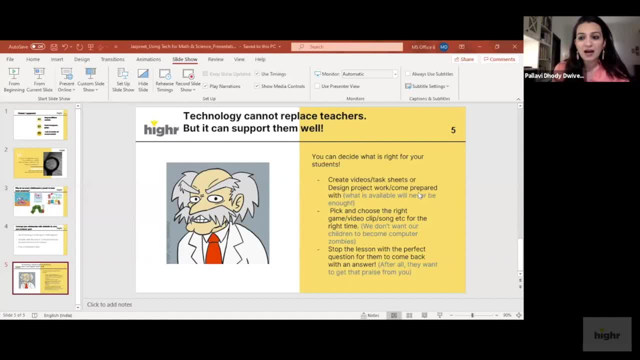 have access to you directly. it becomes particularly important at this point in time um to reach out to our students and try and understand what their needs are, and this becomes particularly true for some of the the younger talks and in the primary classes. so thank you so much for all of those. 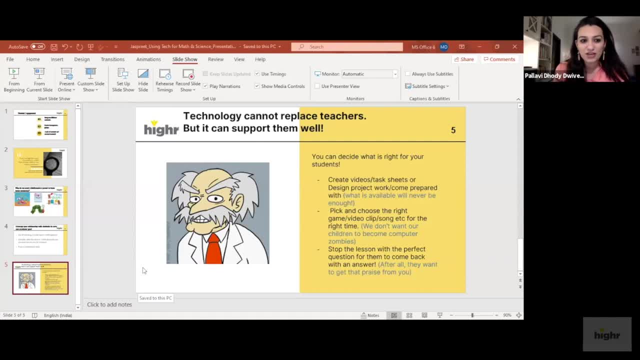 wonderful insights. just breathe, and thank you very, very much for sharing um some of these lovely uh math stories uh that we can use in primary classrooms. so thanks a lot for that. um, there were a couple of questions that did come in, which i thought we'll take one or two of these before. 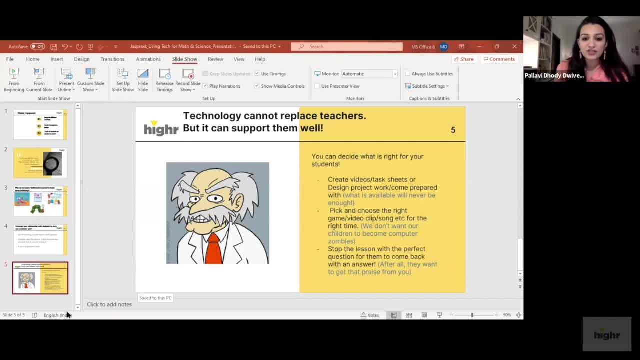 we sign off for today. um, there was a question around, uh, which was about what is the relationship resources that you could use for audio. this is something that you had suggested. just keep that. are there any other, any sites or any tools that you can use for differentiated instruction when? 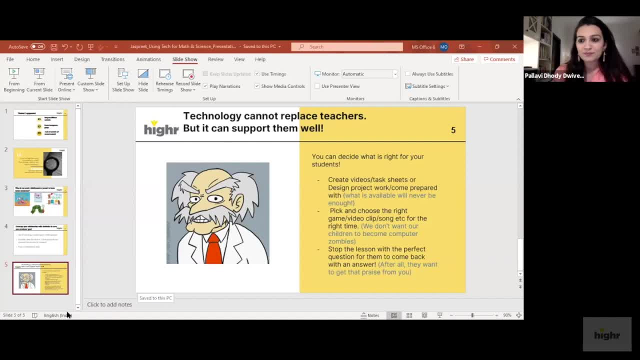 it comes to auditory learners. so the easiest that I use for my school and my children is a Microsoft PPT where there's an option of voiceovers is available. you just need to have one picture and keep talking behind it and share. make a short clip and share it with children. so that's the. 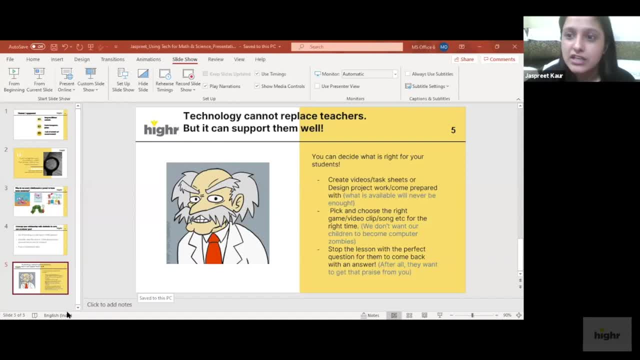 easiest that we use. there are tools like audacity to change the more the mode, the way the character talk. so these tools are available. you just have to google them and you get them. so the easiest: if you want to differentiate for your children, just go with Microsoft PPT. easiest to do very 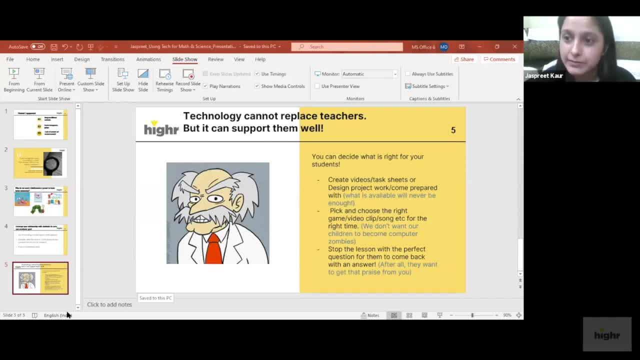 little training required and voiceover sender clip as per the need of the children. absolutely, absolutely wonderful. thank you so much for that. there's also some lovely audio books out there that you can share for free. a lot of audio books are now available on kindle for free. they've particularly 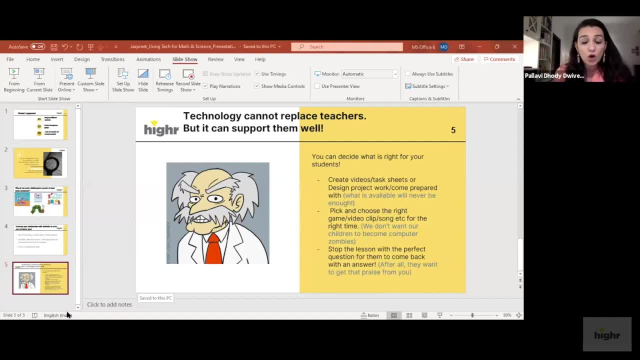 been made free for this time. there's there are some great audio resources also available for primary school students on this great website, where they have a great repository of primary school audio as well as video resources. so thank you on that note to all panelists for having been here with us today and 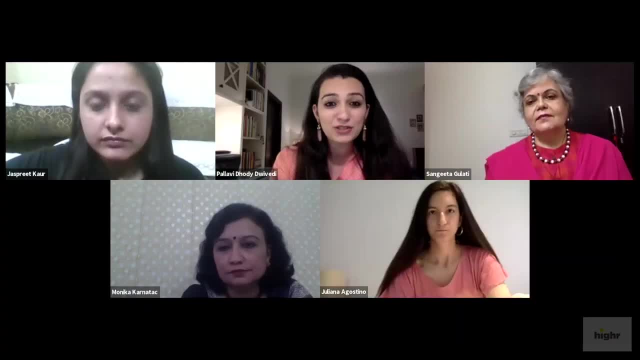 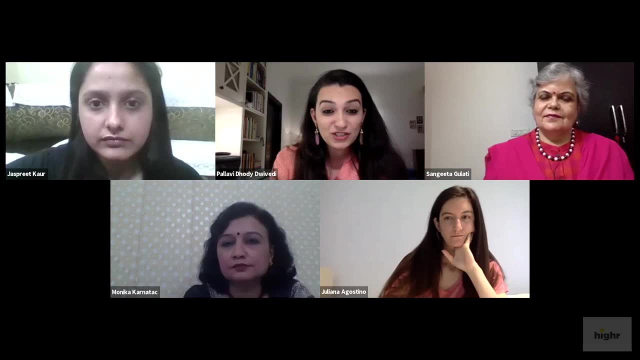 thank you very much to all the the wonderful participants who came in, who asked us these amazing questions, who kept inquiry and learning and and questioning and growing going on, and we look forward to to continue to engage with all of you as the summer of learning goes ahead later.